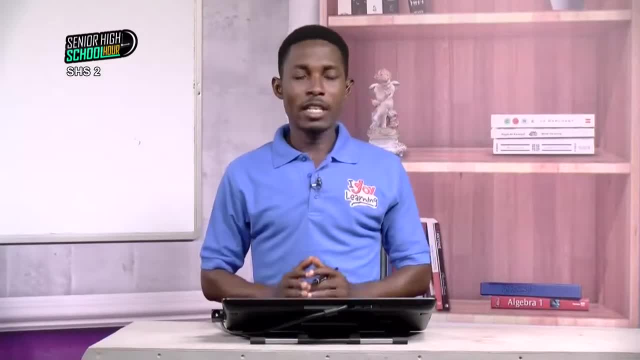 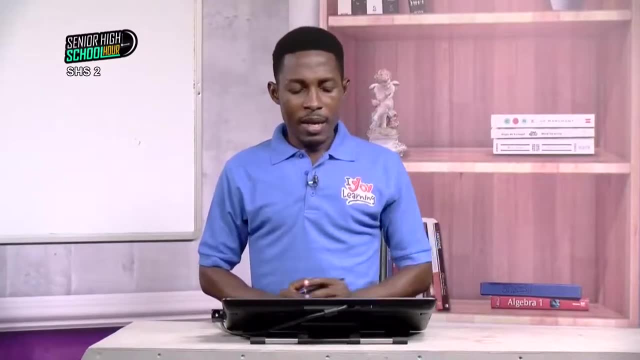 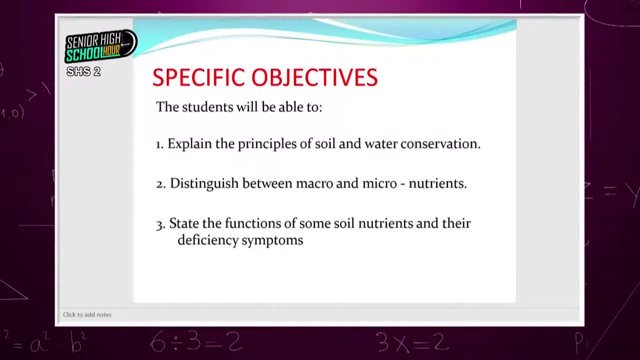 Have your pens, have your books and all that. you need other materials that you need for us to journey through this one hour. At the end of our lesson today, you, the student, should be able to explain the principle of soil and water conservation. 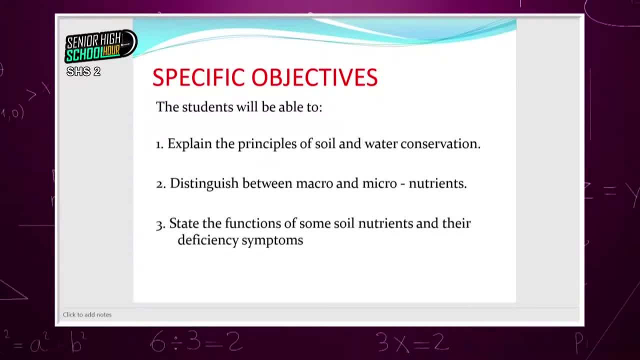 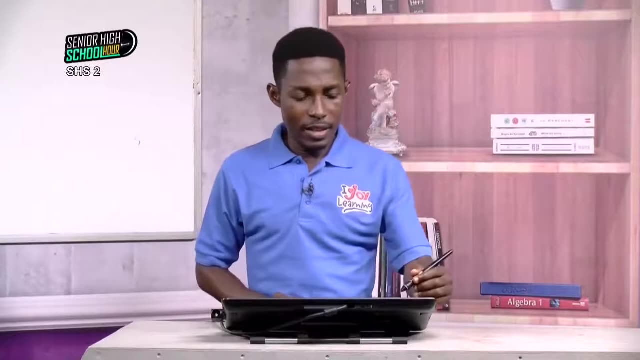 You should be able to distinguish between macro and microorganisms, and also states and functions of soil nutrients and their deficiency symptoms. Yes, from that definition you can see the difference between macro and microorganisms. I believe that there's something about the word soil. 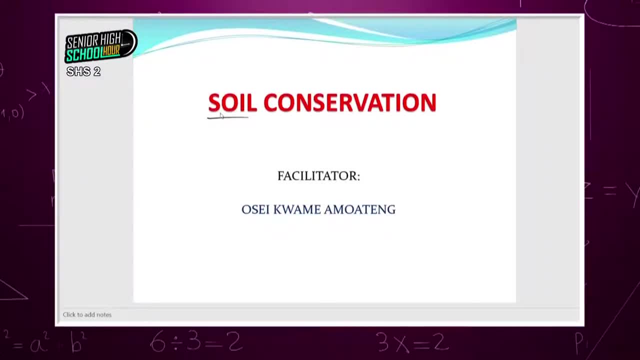 Soil. I believe you've heard soil many times From JHS primary school. you've heard soil. The word is: you've heard. I also believe you've seen the soil before- Why The house you live in is built on the soil. 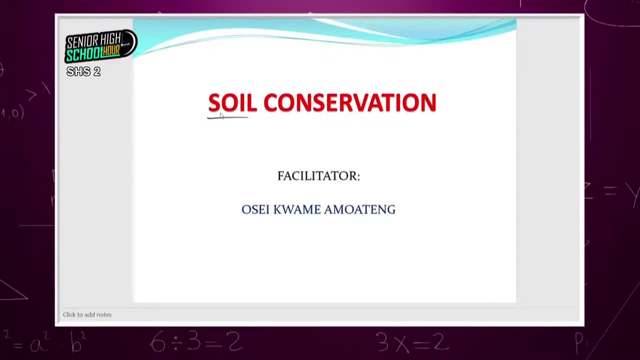 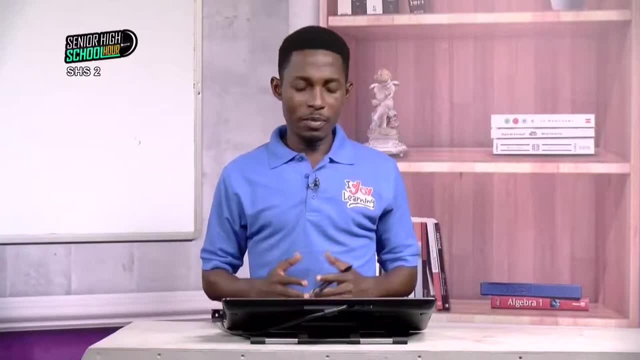 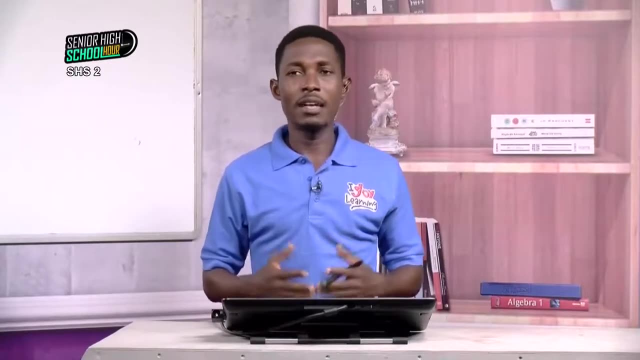 The road we walk on are built on the soil Most of the time. what comes to mind easily is when we talk about farmers. We think farmers plow the land. When we use the word the land, that means they are plowing the soil so that they can plant maize cassava. 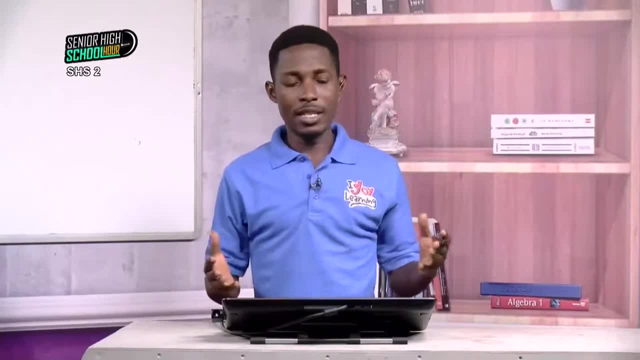 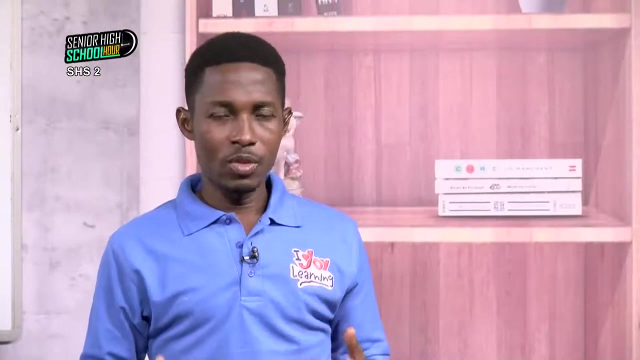 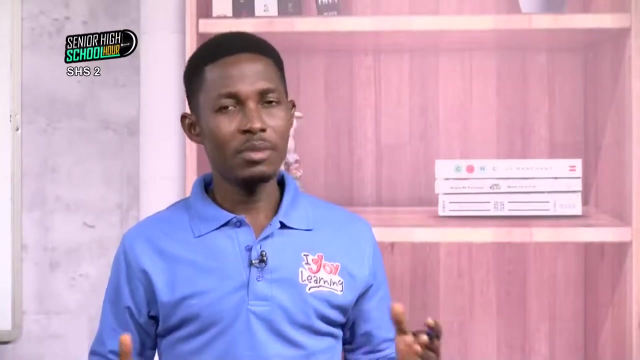 So we uproot maize, uproot cassava, the root tubers from the soil, We plant the maize on the soil, But where do you pass before you go to your school, To the market, to the church? Definitely, apart from the street, you may see some brown colored parts, which probably the soil. 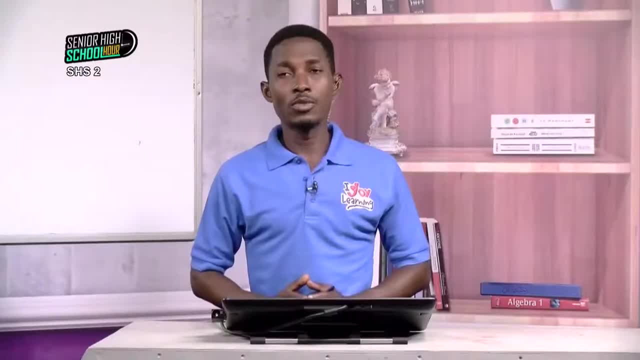 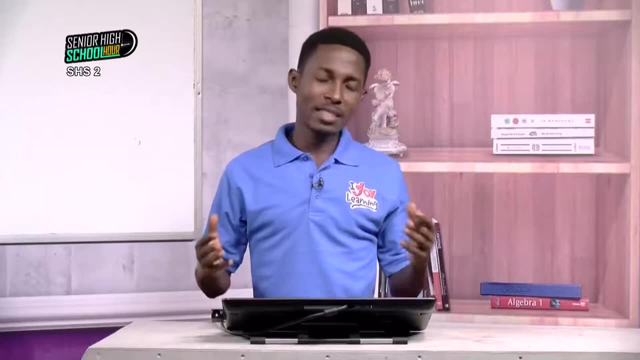 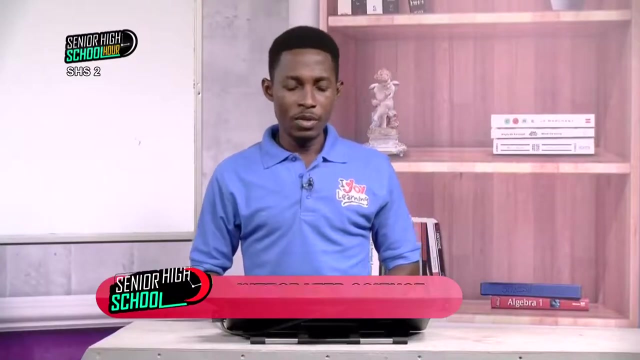 So, by default, you've seen soil before. Usually the boys play football, You have a school park And sometimes you have parts with green grass, parts with soil. So basically, you've seen soil, Soil, Soil. But the question is, where did soil come from? 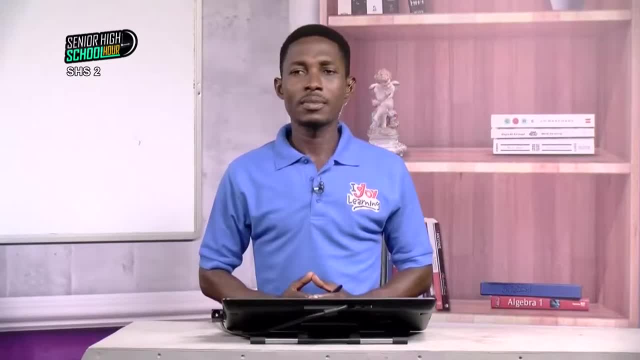 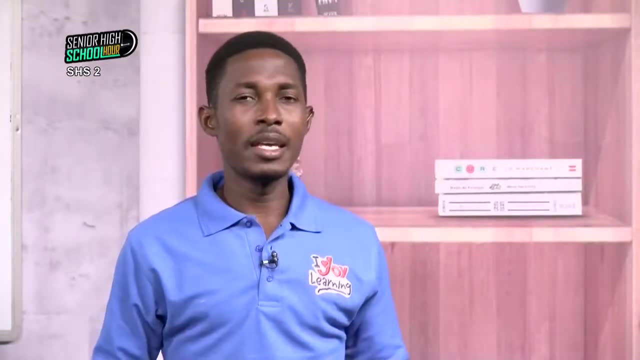 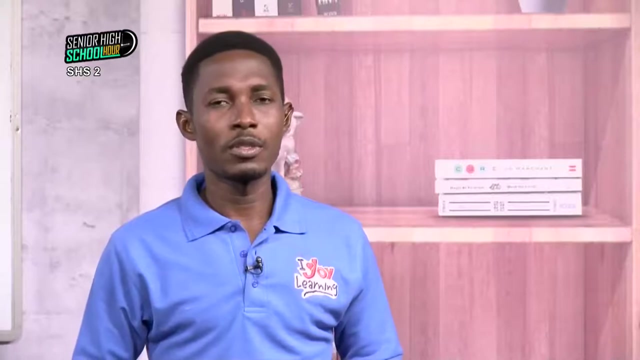 And how will you define soil? Any time you see a stone, a small stone, put in your mind it was a big stone and many things have happened to it for it to keep breaking down into smaller forms. That small stone soon, or some years to come, will crash into very small particles. 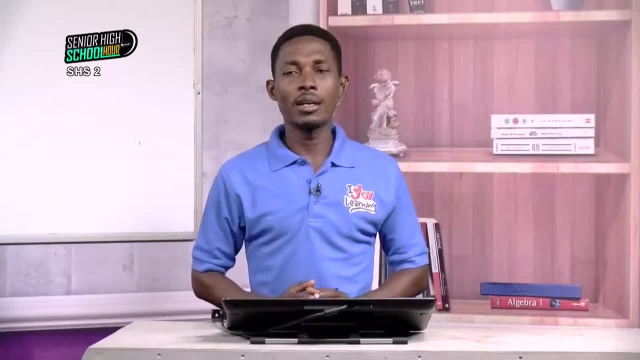 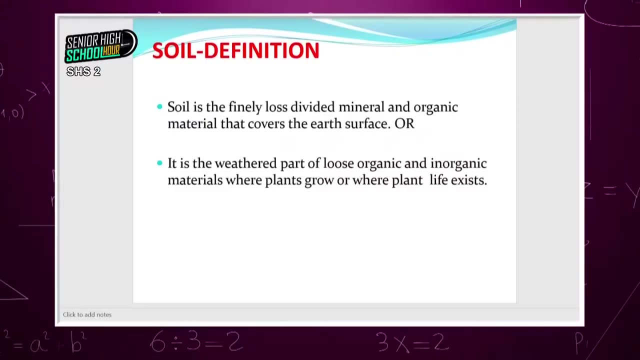 Small particles that you can feel or spread in your palm. So to define soil, we say soil is the finely loose, divided minerals and organic material that cover the earth's surface. It can also be defined as the weathered part of the loose organic and inorganic material. 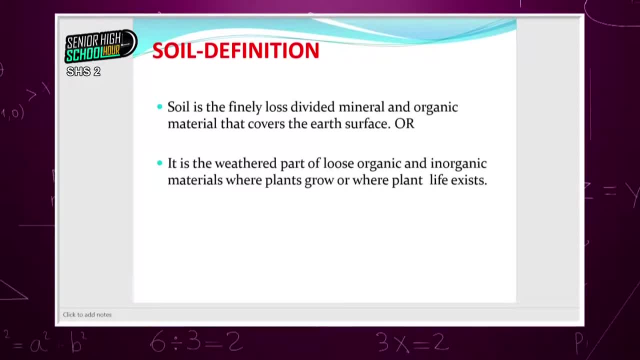 Where plants grow Or where plant life exists. Let's hold on to the word weathered. That is the whole idea of how we get soil. We also look at the earth's surface, So let's start with the weathered idea. As I said, there are big rocks. 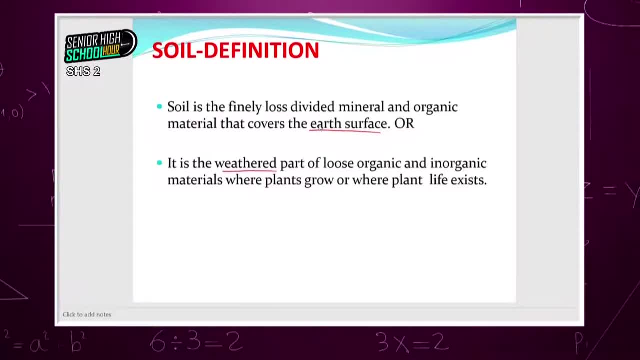 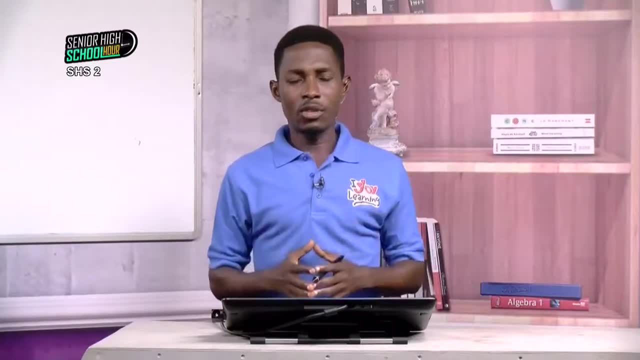 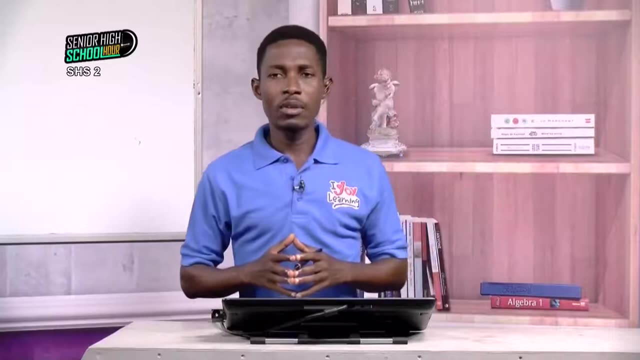 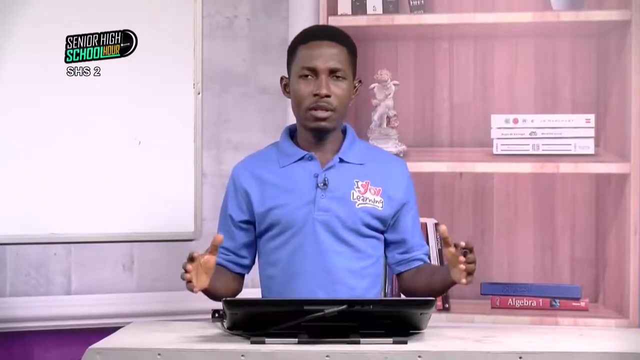 Either below The earth Or some you see as mountains, Some show up in the sea. All these rocks, through some processes, will break down. So the process of breaking down rock through certain processes is called weathering of rocks. So a big rock would divide either by biological means, physical means or chemical means. 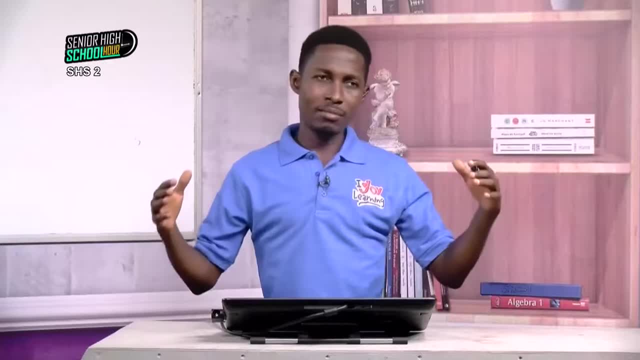 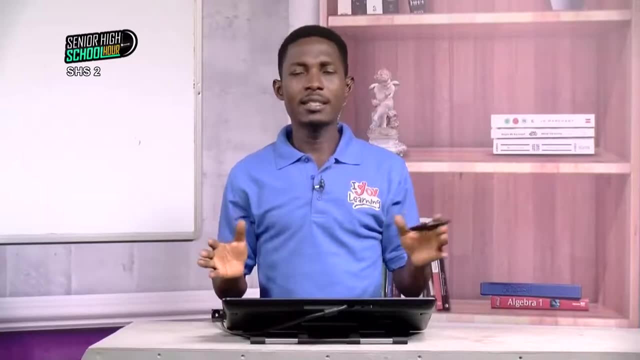 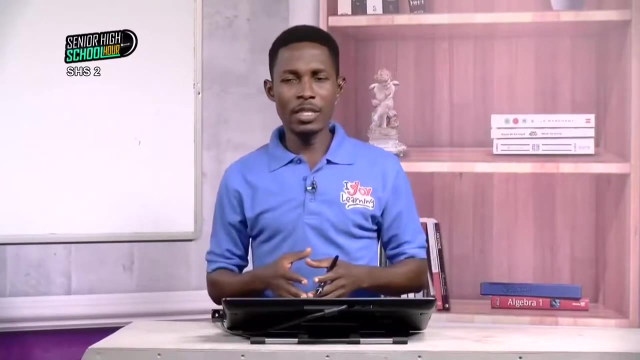 So a big rock would divide into maybe less incisable amounts, Let's say very big. it has been broken down to mini forms or mini size. Those mini size will be broken down again into smaller size, Smaller again to very small size. 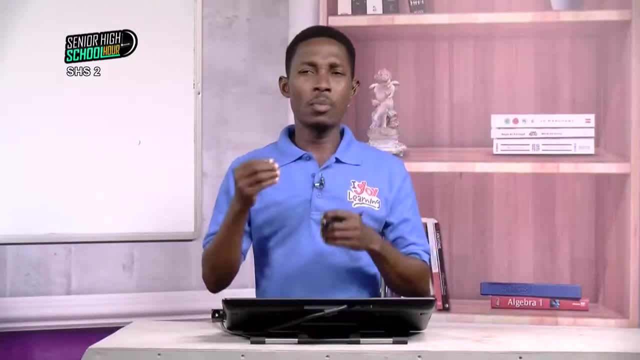 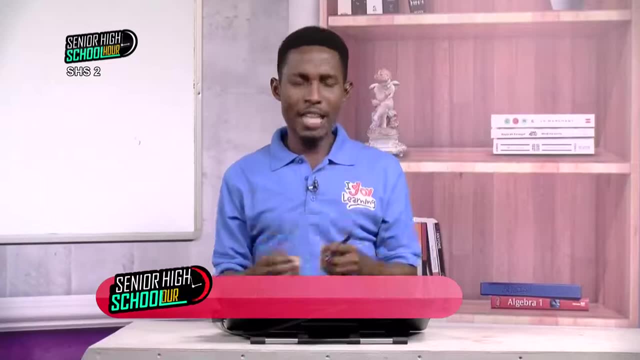 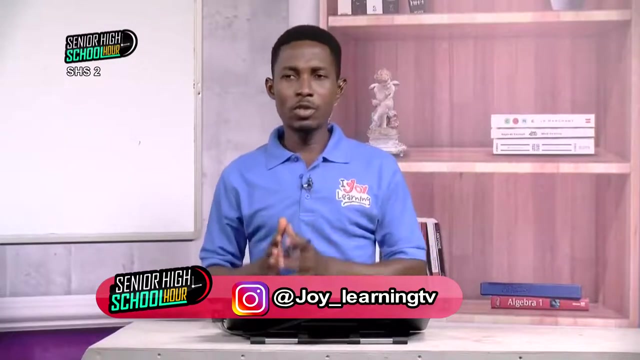 Very small size again to tiny size. You can call pebbles and those things Which can also crash again by processes. That crashed stone is what forms the soil we use. So every soil you see today came from a very big rock. Yes, 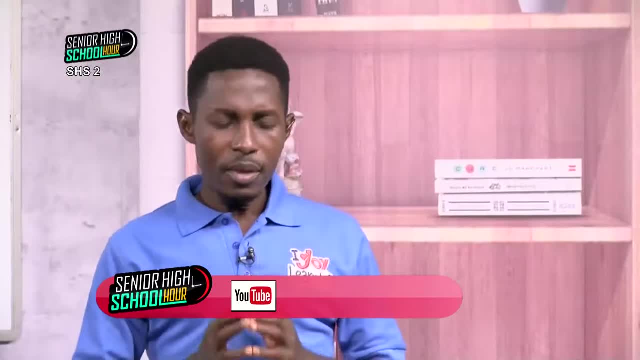 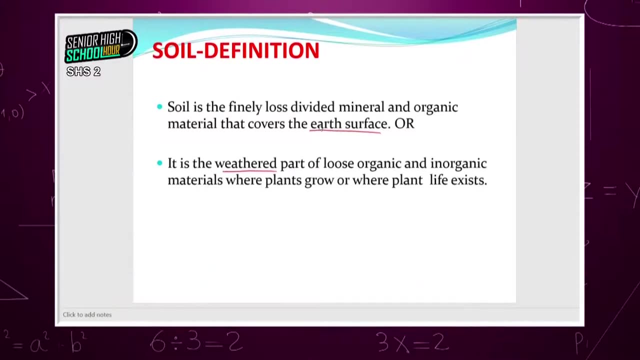 So we get soil from big rocks, But when they crash and they spread on the surface of the land, Let me put the land Because you can use your hand to collect them. We say they are very loose Because you can spread them. 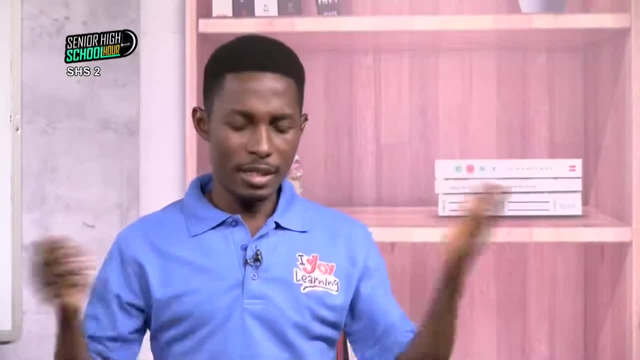 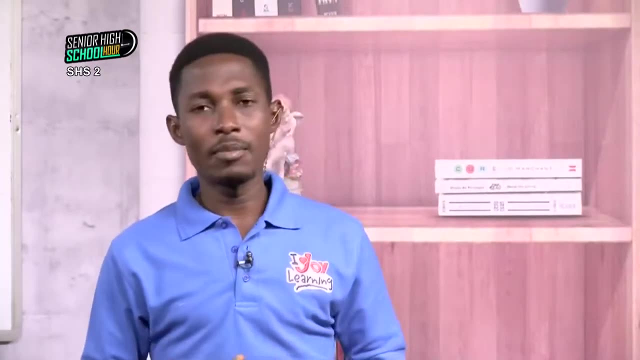 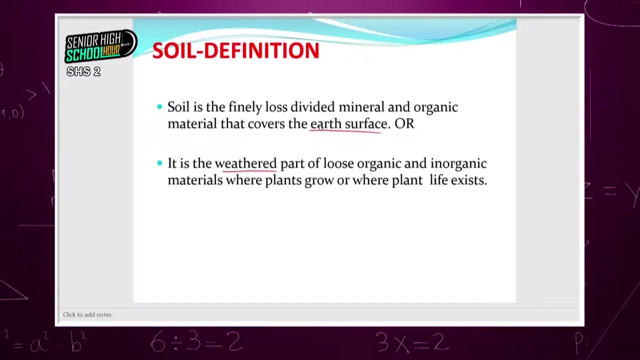 Blow air onto it and it will just disappear. So we say they are loose. They use the word organic and inorganic material. Organic in the sense that they are living, natural or living things. Every soil would have probably microorganisms or some macro organisms. 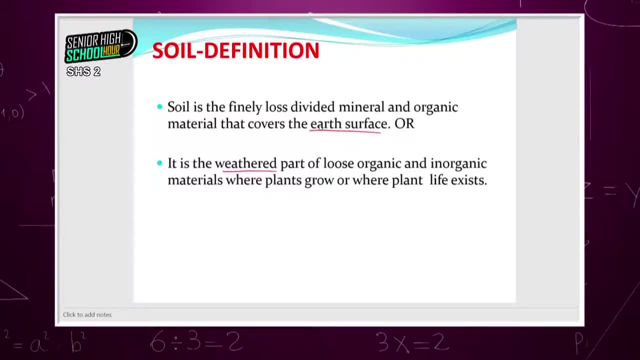 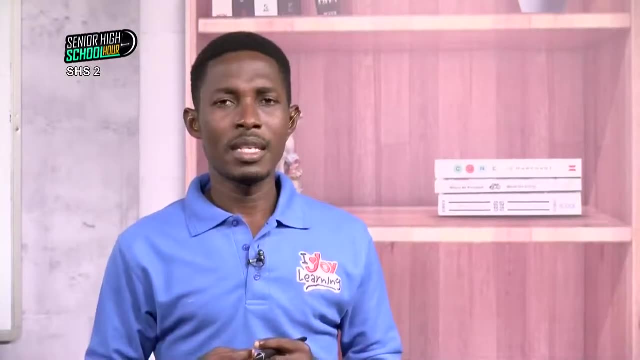 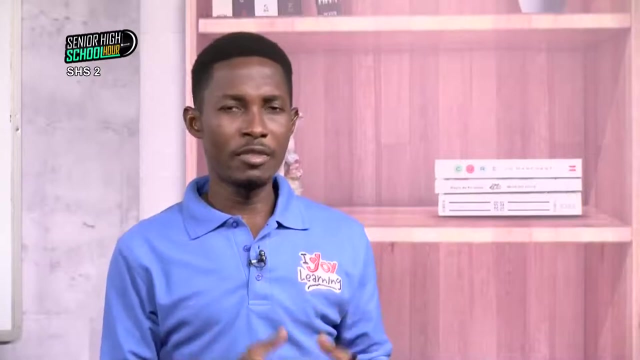 Like earthworm living in them. In addition, when these earthworm or the leaves that fall on the soil decompose, or rot, As we usually use in a simple way, Those things form the humus That mix up with the soil, So the humus, which is a decomposed form of a living organism. 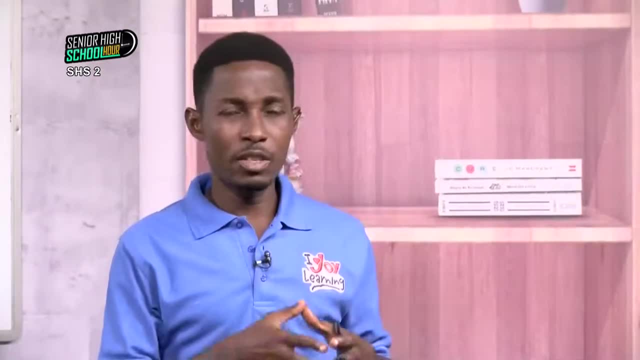 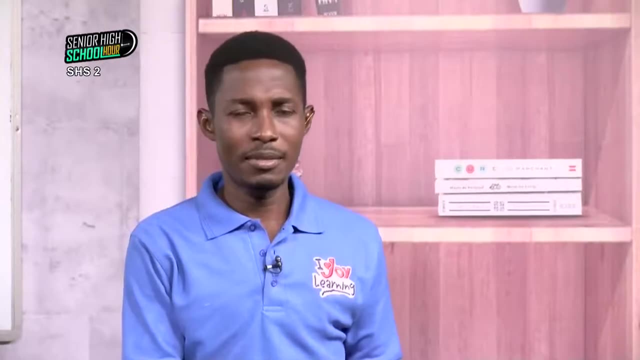 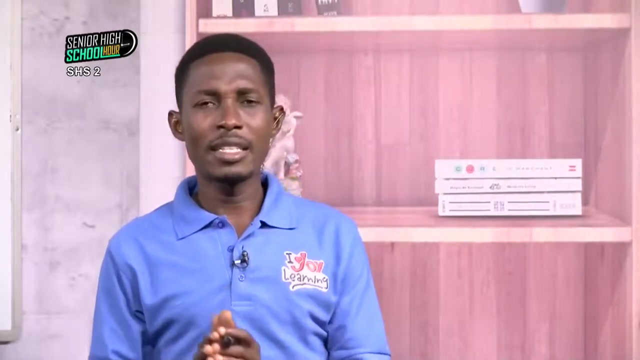 Plus, the living organisms that are living in the soil Constitutes the organic part. Yes, They constitute the organic part. Then this rock itself was a chemical element, And all chemical elements are not organic. We rather classify them as inorganic material. 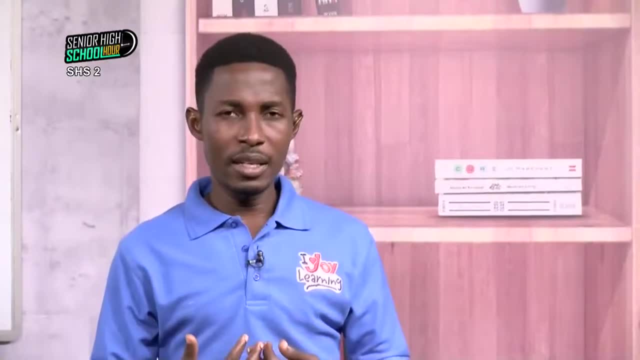 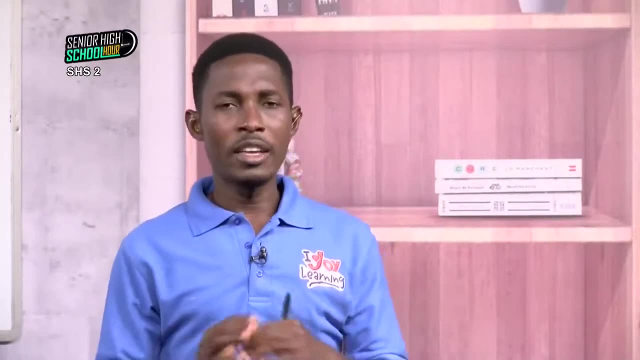 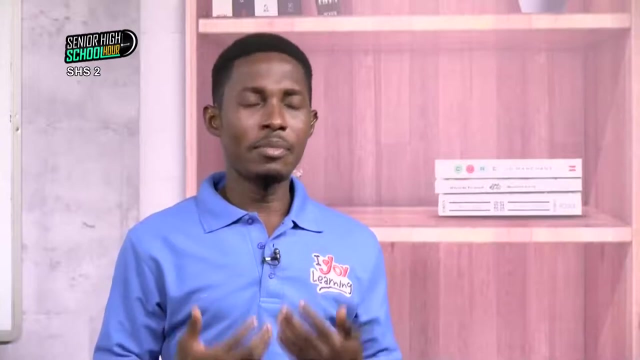 So to get a soil is a combination of living things or natural things And what we may say natural things such as inorganic material. When they form this together, We human beings that work on it, We grow plants on it And plant also. 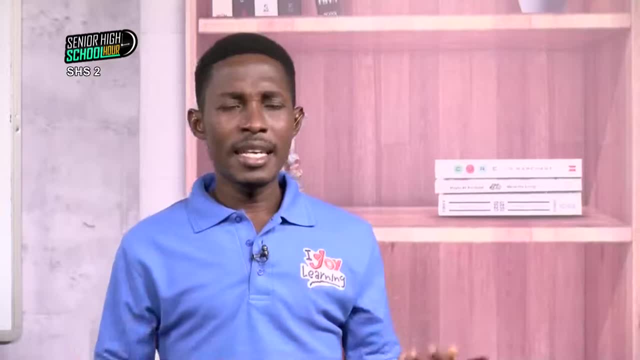 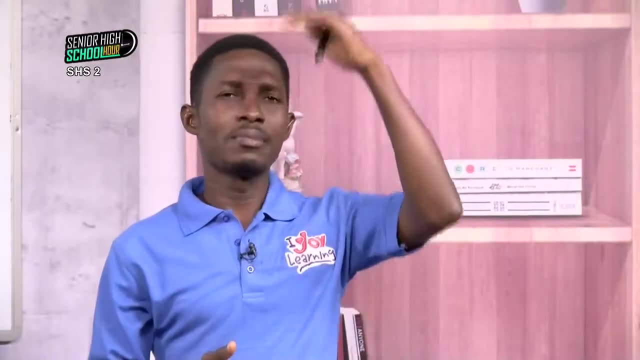 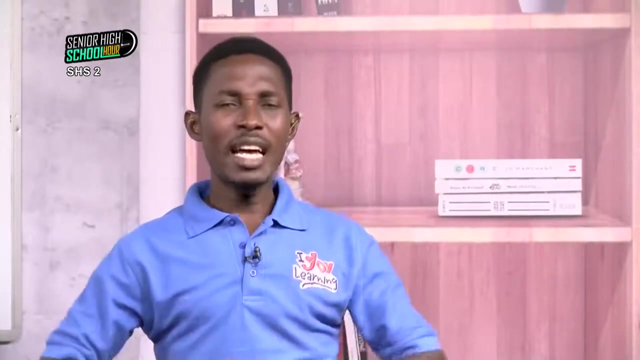 Life exists on them. Secondly, The earth is very big. People move out of this earth With space shuttles and move outside the earth as a planet. But when you come here, you land on a solid path. That solid path we call the land. 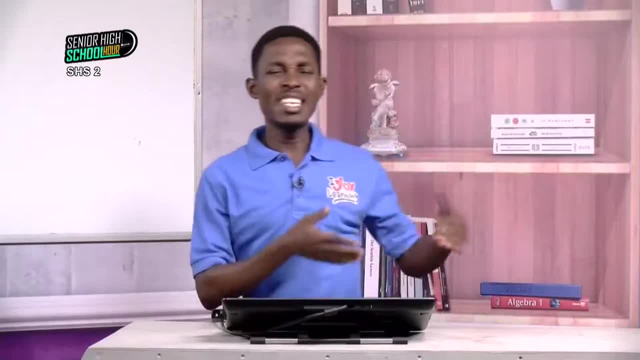 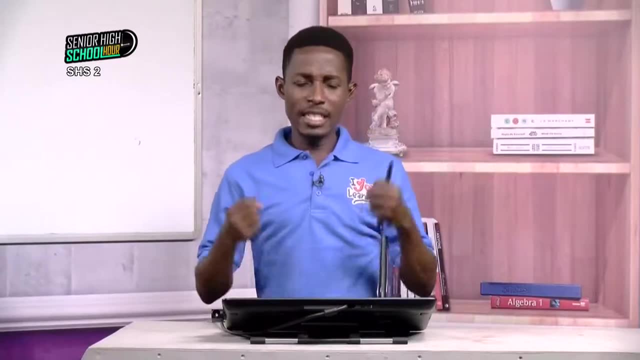 But the surface of that land is where we have soil. Beneath earth, deep, deep, deep, We are going to have huge rocks, Huge, huge, huge, huge rocks. There is the rock that, even when it rains, The rain will penetrate. 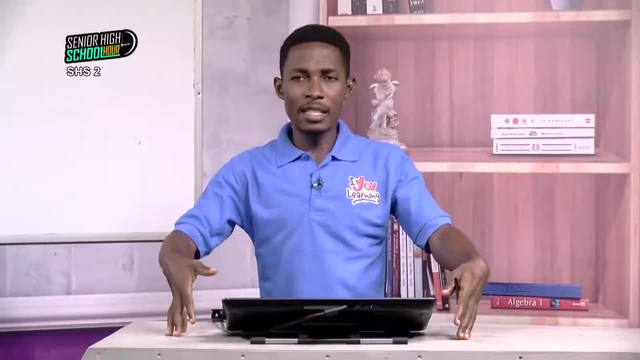 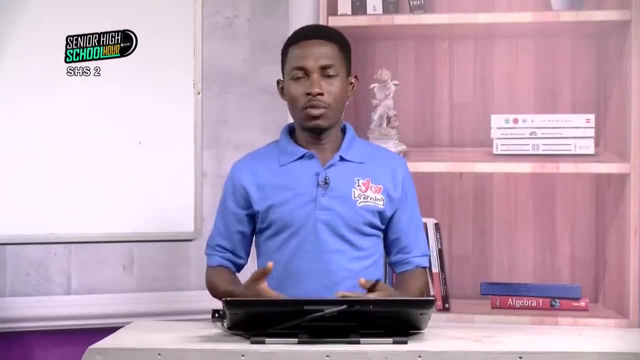 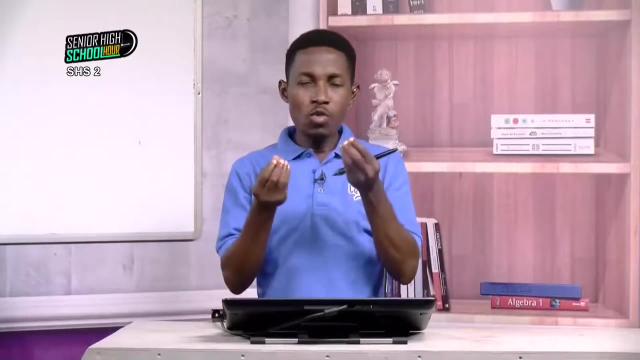 And when it gets there it cannot go again. We call it the land table. So you see that That means down there. we are not going beyond rocks. From rocks Then we go to the volcanic, whatever down there, So where we have that loose one. 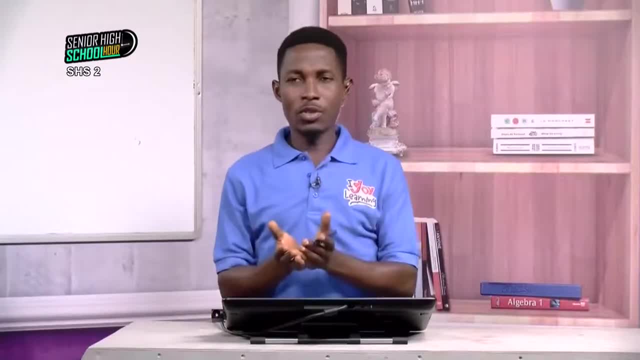 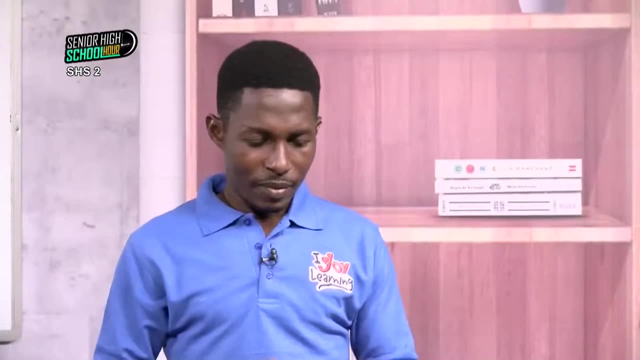 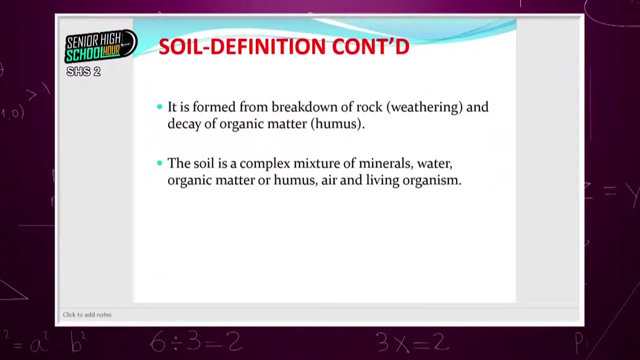 Is the one at the surface. So if you are talking about soil, You are talking about the loose one at the surface, Not the compact, stony ones down there. We can also define. As we said, It is also formed from the breakdown of rocks. 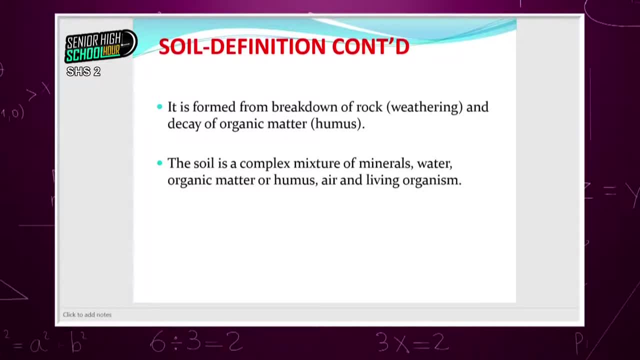 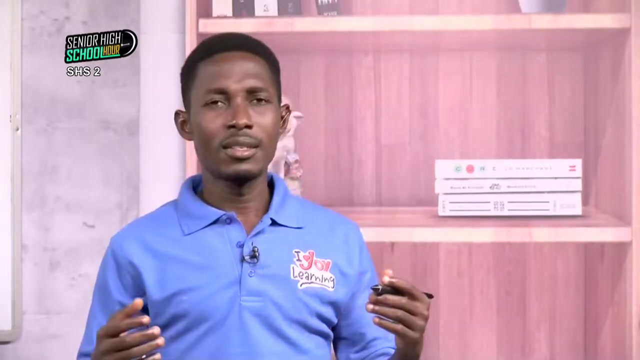 And decay of organic matter. Another accepted definition: That is a complex mixture of mineral Water, Organic matter Or humus, Air And living organisms. So this is how we define the soil. What do you think is the importance of soil? 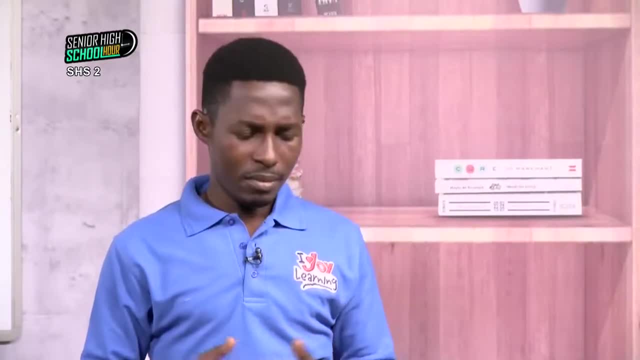 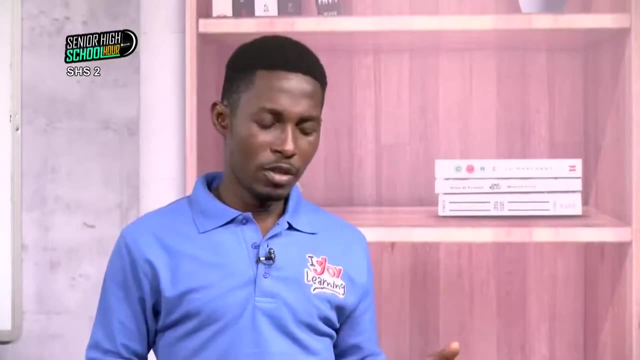 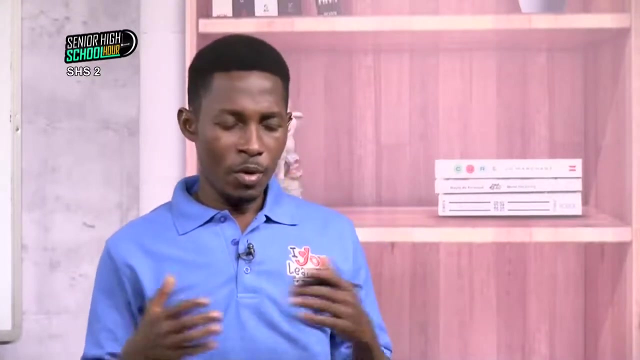 You can see what are its uses From your head, From all that we have discussed. If you look at the farmers points, You know what they use it for For plants. You know what they use it for. So, giving you these ideas, 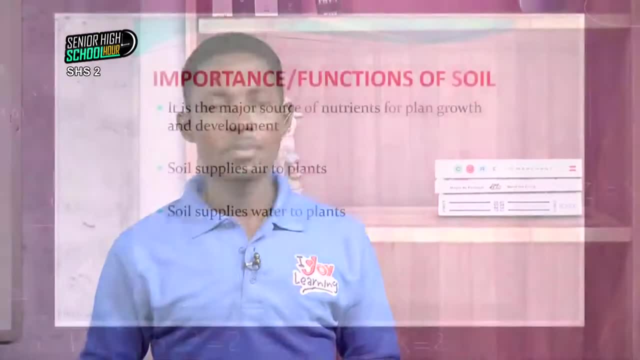 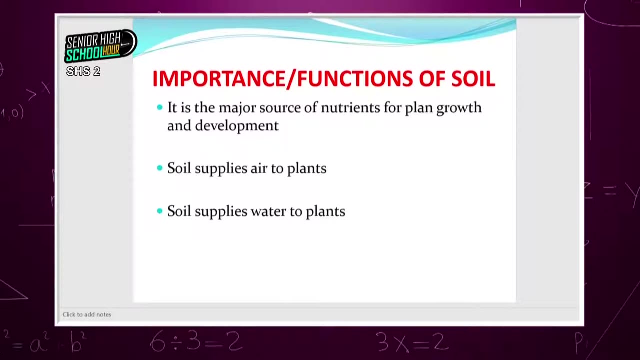 Let's look at the importance of functions of soil. First is that The soil itself Is the source of nutrients for plant growth. Let me Add a T to the word plant here: Plant Growth. Why do we say Nutrients? 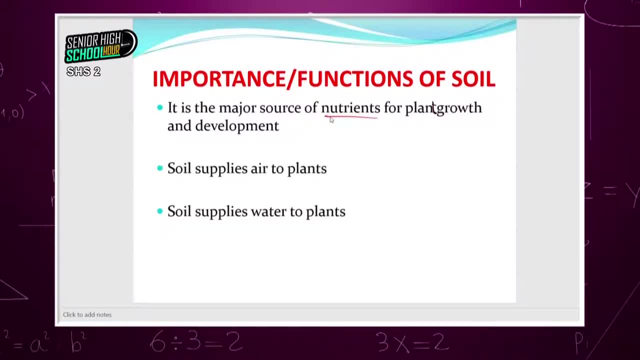 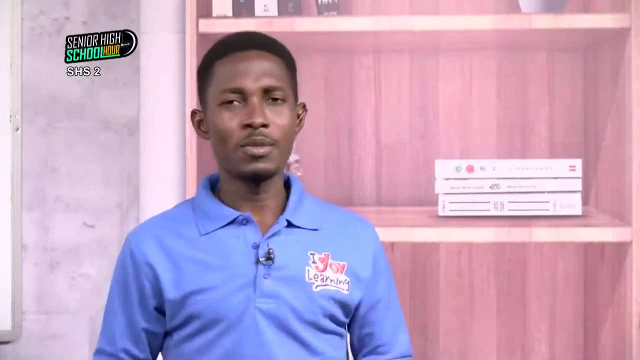 We will be going down The slide and you come across macro and micronutrients. Probably a nutrient Are elements that the plant needs For growth And for a good life, But the rock that was formed, That came from nature, Constitutes elements. 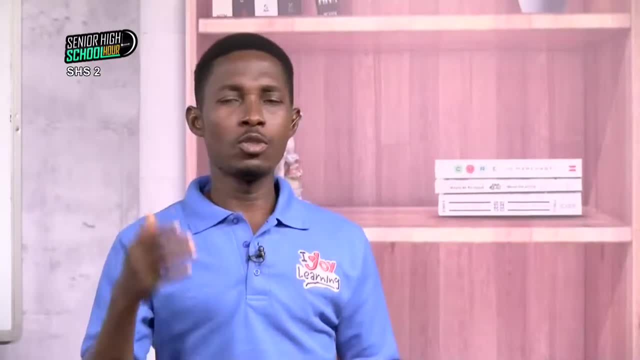 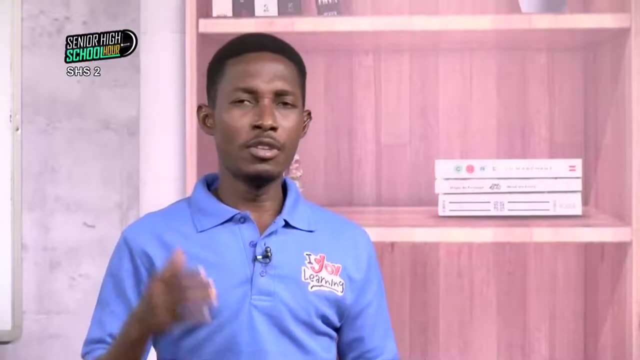 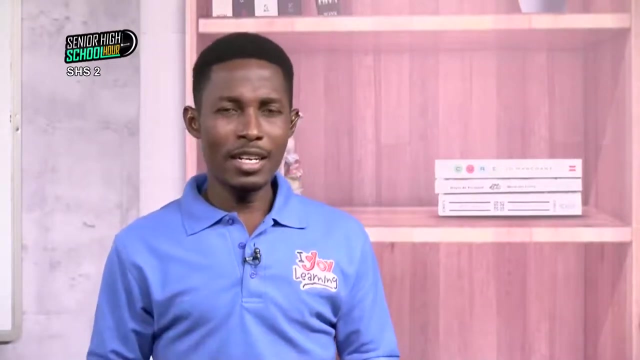 Yes, Elements we studied during the periodic table, Like sodium, Like carbon, Like hydrogen, Like whatever you know- Aluminium, Silicon- All these are elements you know on the periodic table. Yes, When you take the rock And you crash it. 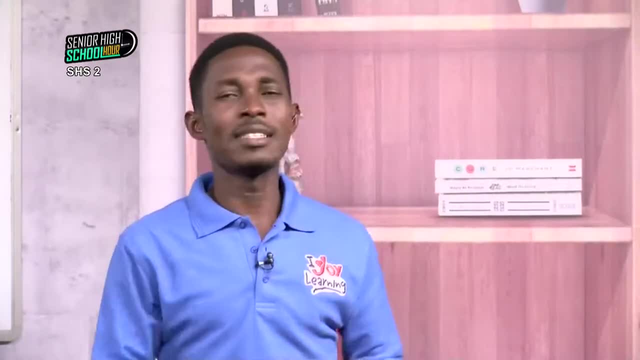 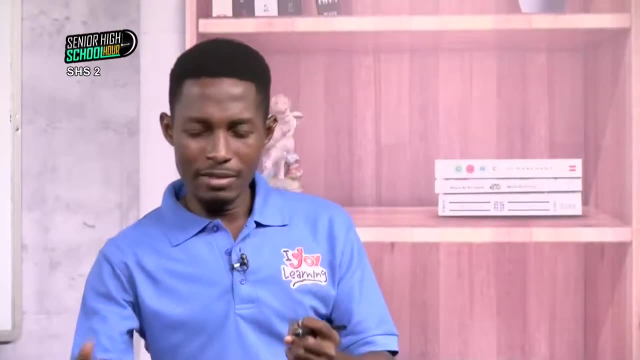 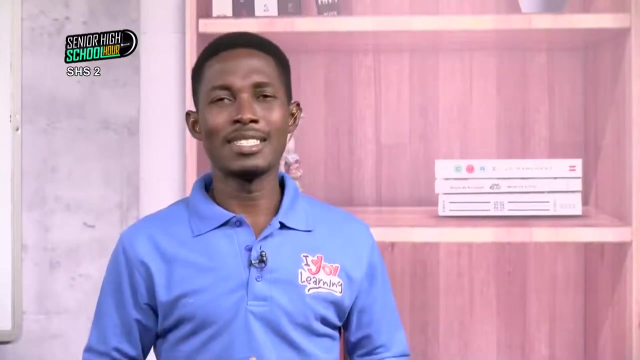 And you test it, You find that they also contain This element. It is this same element the plant needs. So the soil that we work on, That we can use our hand to collect some. It itself, the element, Yes, It itself the element. 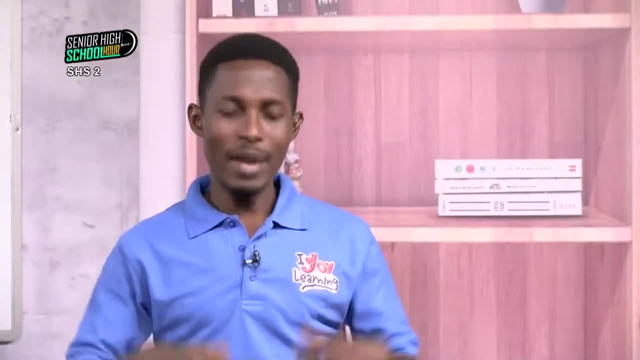 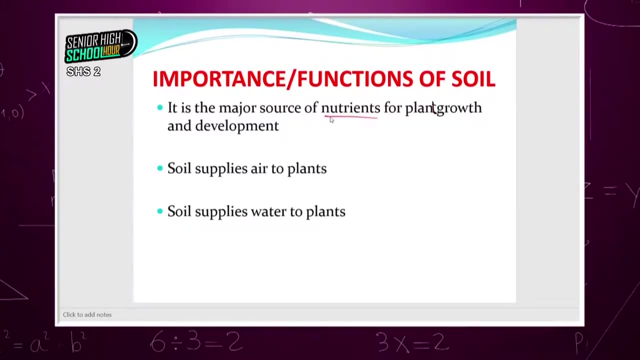 So the soil mixing with water can even go into reactions, But it itself the element. So we say that it is the major source of nutrients For plant growth and development. In addition, When organisms die, They decompose, And those organisms also had nutrients in their body. 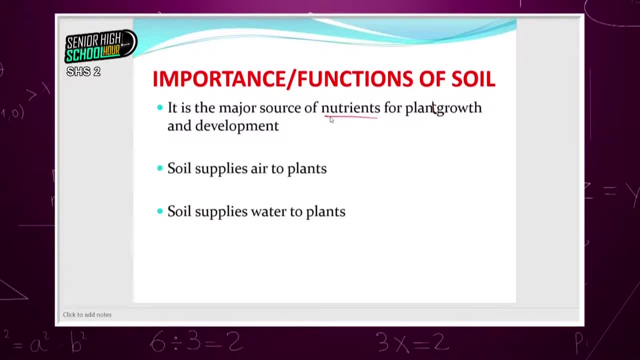 And these nutrients or elements in their body Will decompose into the soil And the plant will make use of it. So the soil as a soil Is the first source of nutrients for the plant and its development. Another is that Plants take water. 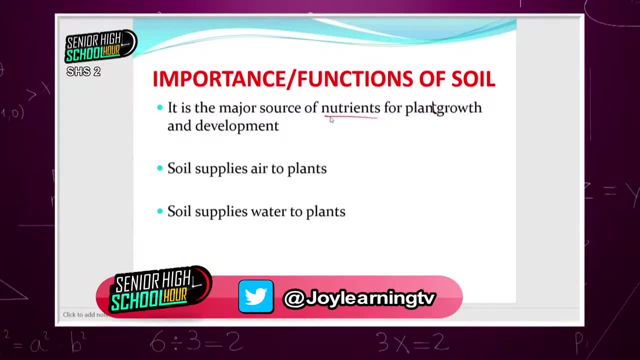 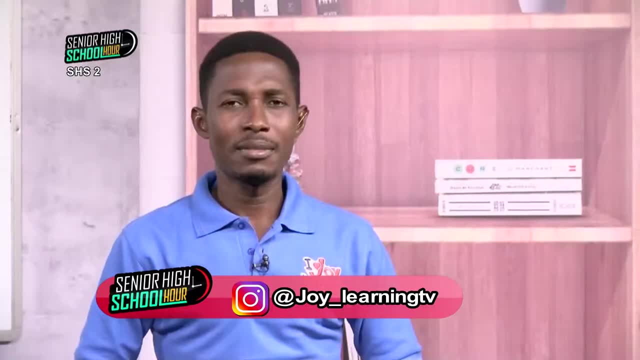 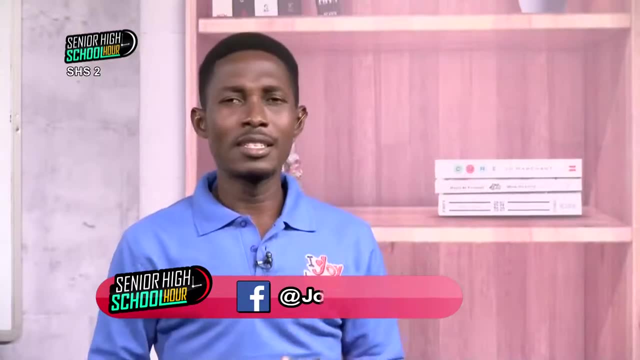 from the soil or from the ground. even when it rains and it settles on the leaf, it cannot penetrate into through the leaves, into the plant, unless probably some few water plants. but for the land plants it's like your body. you breathe in through your nostril, you take water through your mouth when it rains and it settles on your skin. it will not penetrate your skin and enter your body. so for plants to, they need to take water, so they wait for it to rain or settle on the surface of the soil. there are a lot of chemical reactions that will bind some soil to the water, some leach. 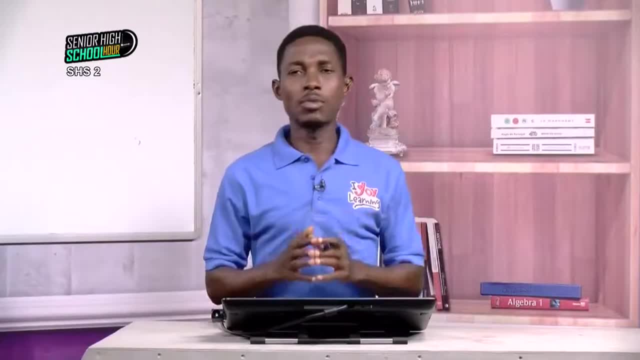 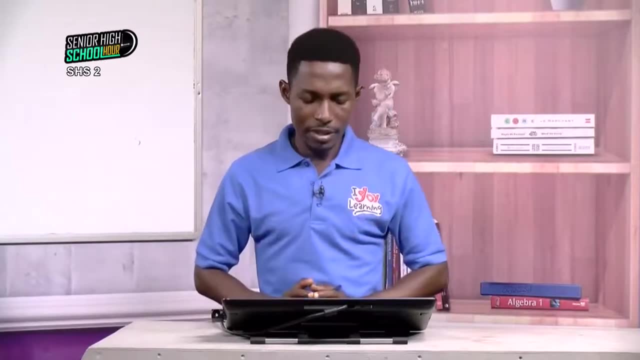 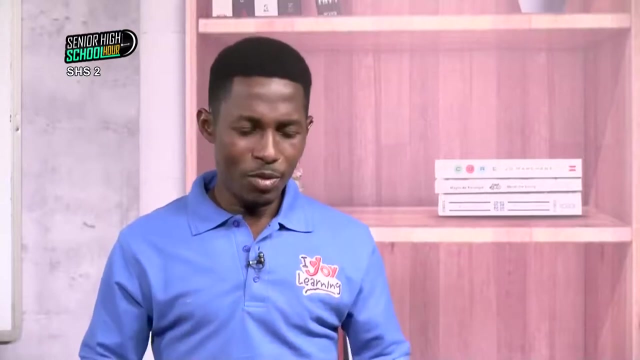 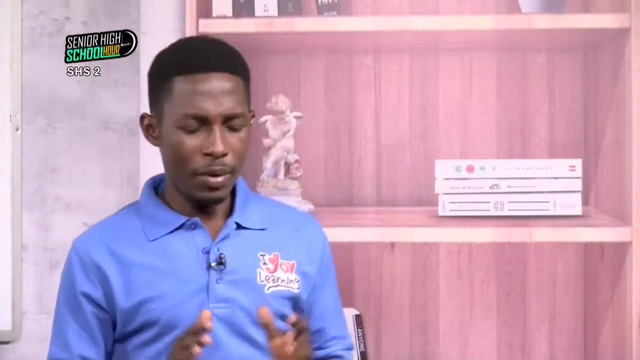 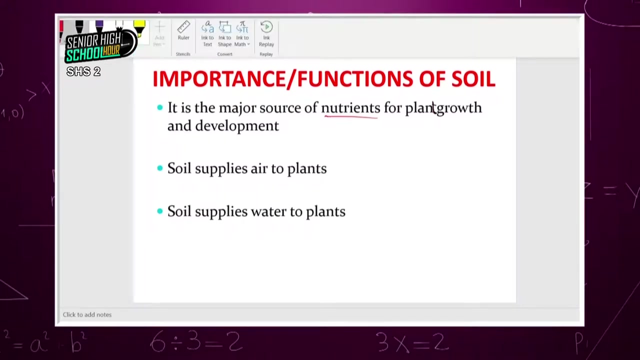 or would penetrate down to the water table. whatever the water is contained in soil before plant can absorb it. another we get into the soil. so the first two is that the air that we breathe, it gets into theera in the soil, and this one would supply some amount of air to the plant. you recall aeration or aeration? 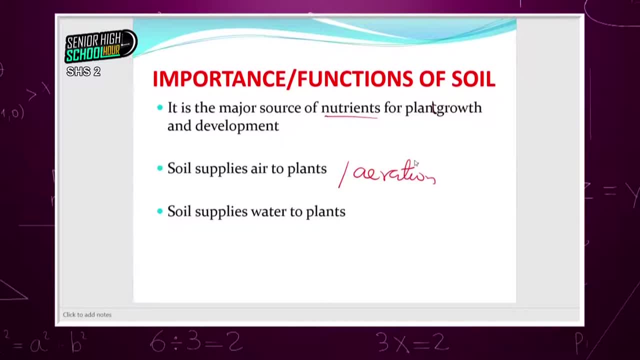 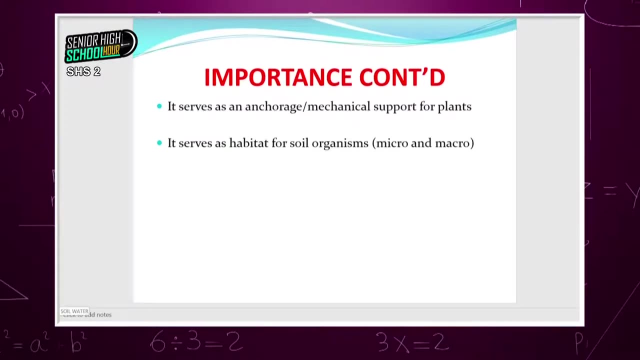 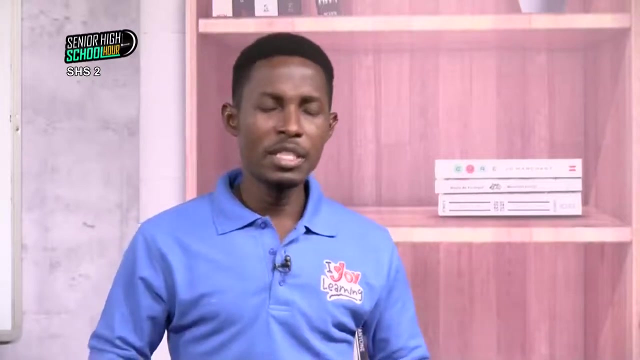 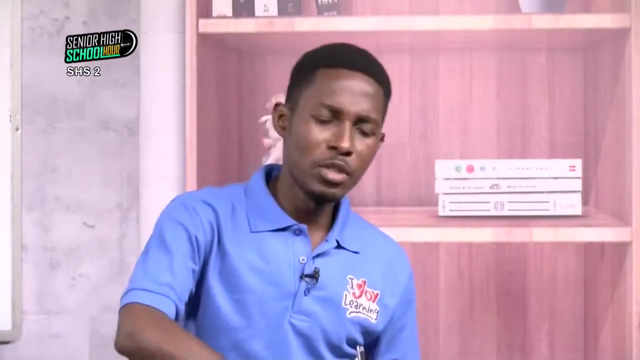 let me appear aeration so plant need adequate amount of air, one from the soil plants when we grow them in the soil. I believe you've seen maize before. after cutting the corn, what do the farmers do? they are put the maize plant and throw it away or burn it. they were a pretty mean that something is. 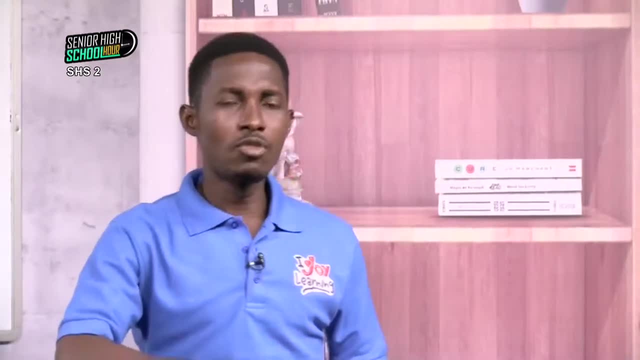 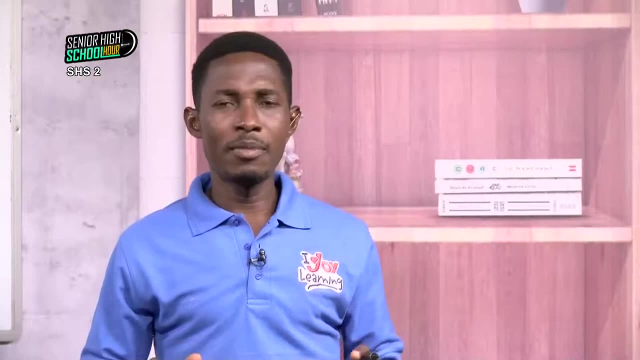 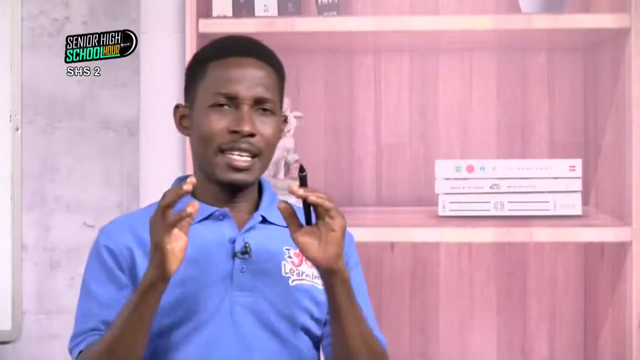 fixed already in the soil. so the plant use their roots to get fixed in the soil so that they can stand, not being pulled away by anybody or by strong wind or anything, so that they can grow. so what we are driving at is that the soil says as an anchorage or mechanical support for the plant. 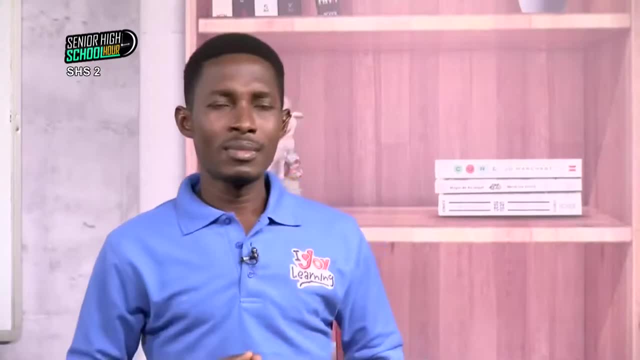 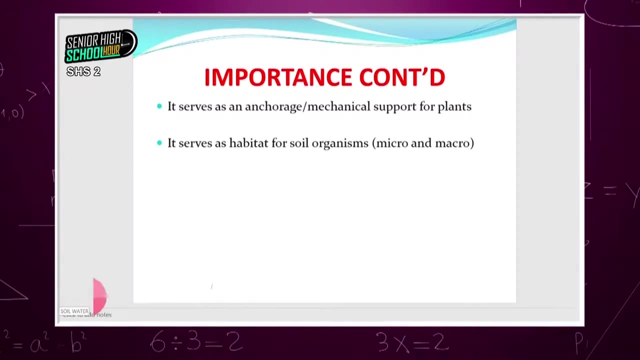 yes, it's for them to grow into it, get firmly hooked in the soil so that they can undergo their life processes. yes, the water plants will get there. they may not have soil in this sense, but they will survive. and one of the last point is that it serves as the habitat for soil organisms. we have things like earthworms. 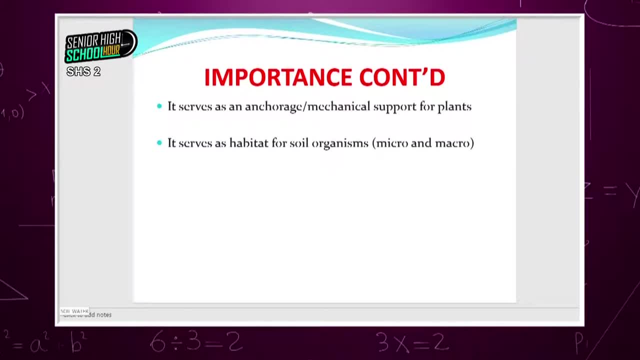 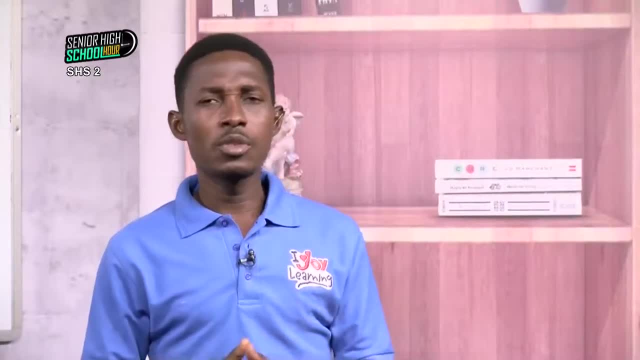 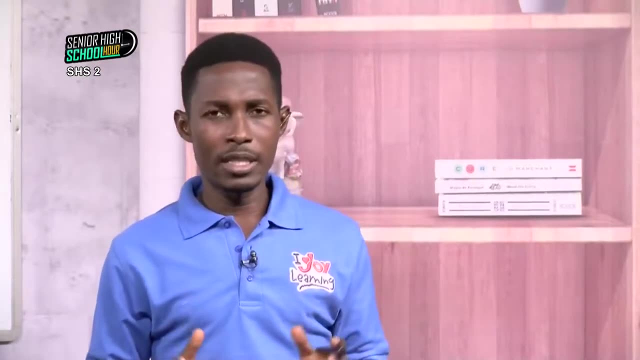 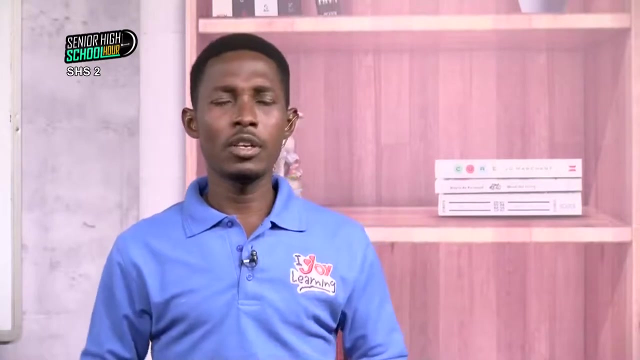 millipedes. they live in the soil or other worms. they are called macro organisms. they have those we don't see with our eyes. usually, when organism dies, you know that it get decomposed or rotten. who does that? they are microorganisms, these microorganisms also living in the soil, and they will decompose these bigger. 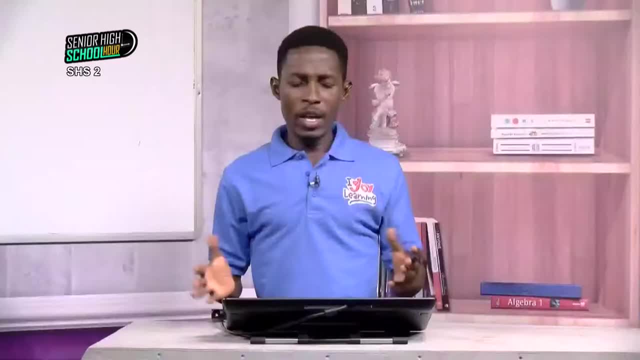 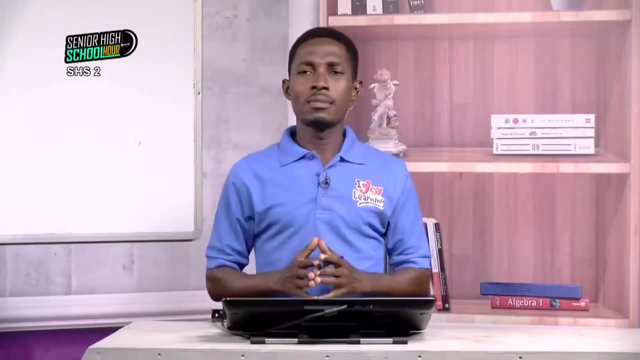 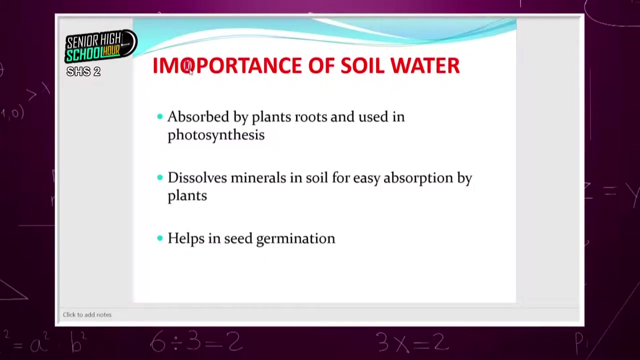 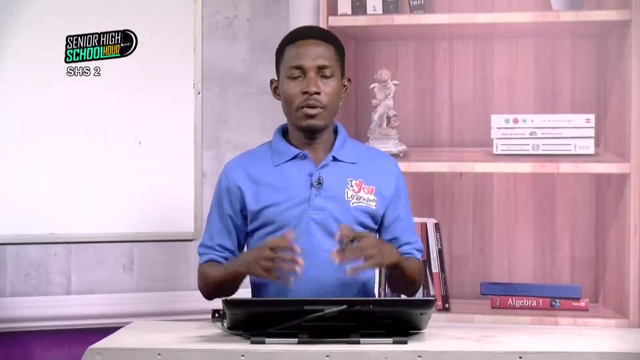 organisms that die. So we have bacteria, we have some prototests, we have some fungi, which are all living in the soil. In addition to this, let's look at the importance of soil water. Remember when we were mentioning the functions or the importance of soil. we 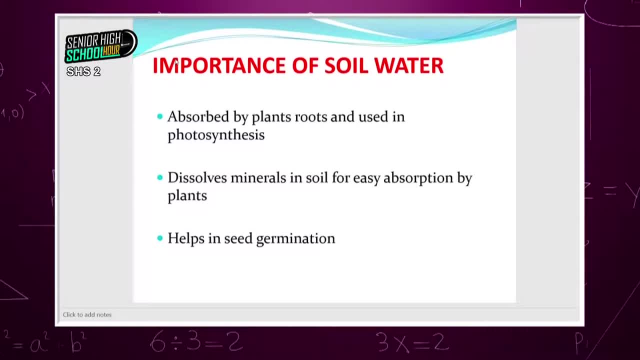 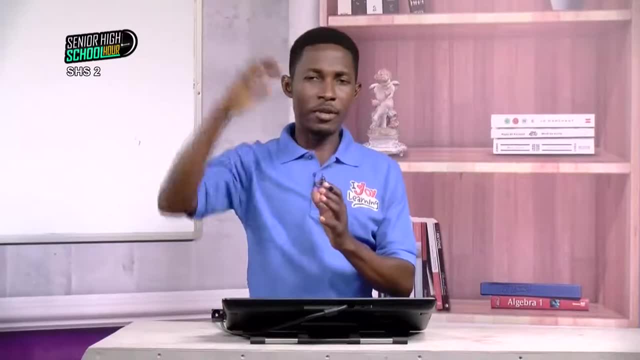 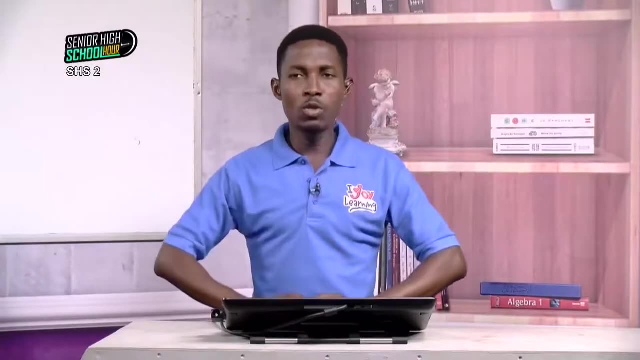 said that it provides them with soil water, And I start with that. We get soil water first. The first process is from the rain that comes from the atmosphere and settles on the soil. Some, immediately, will be hooked on with the reaction of the soil particle itself, Others, 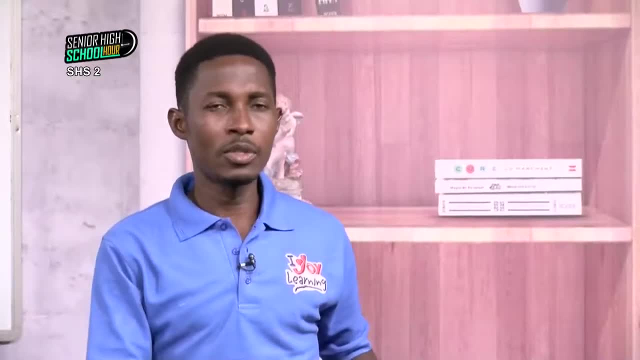 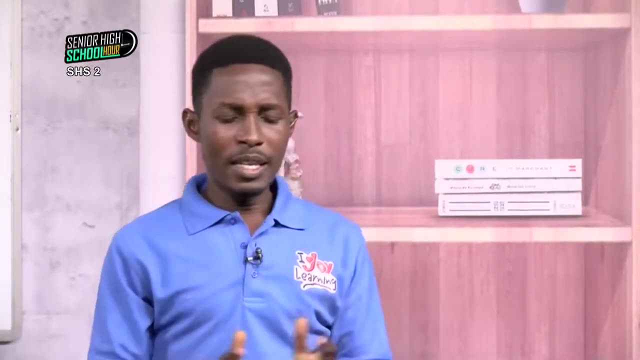 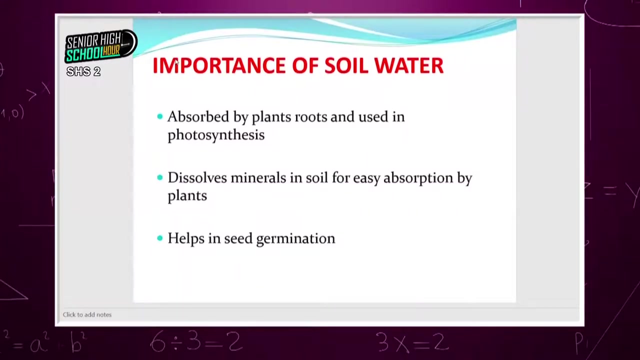 will drain down, down and go to the water table. The day that we want it will rise up. Yes, So these are the sources of soil water. And what would the plant use it for? Sometimes you yourself too can take water in a bucket of water or a watering can, or use an irrigation. 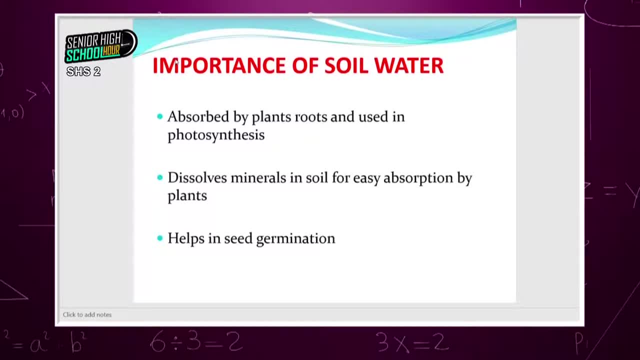 method to water the place. That is also true. It's a source of water. Now we have all these sources of water on the land. What do plants use these for? First of all, the plant uses the soil to water the soil. The soil is the source of water for the soil. 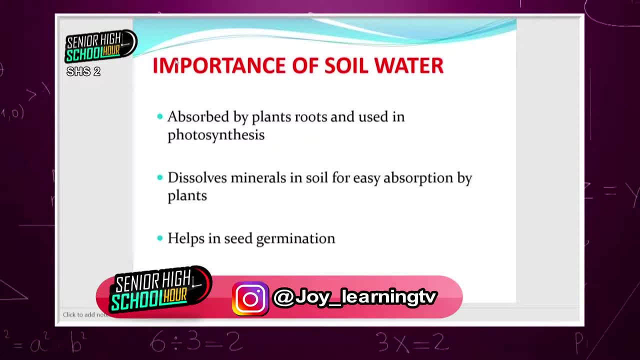 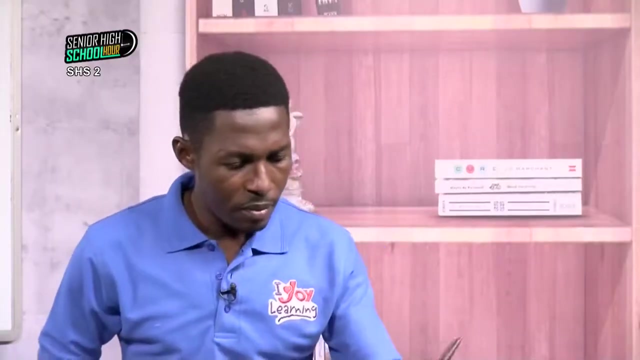 The soil is the source of water for the soil. The soil is the source of water for the soil. The plant roots have an ability to absorb the pool of water around it into the roots and from there will transport it through the stem up. When it gets to the stem up, I hope you've not forgotten your formula of photosynthesis. 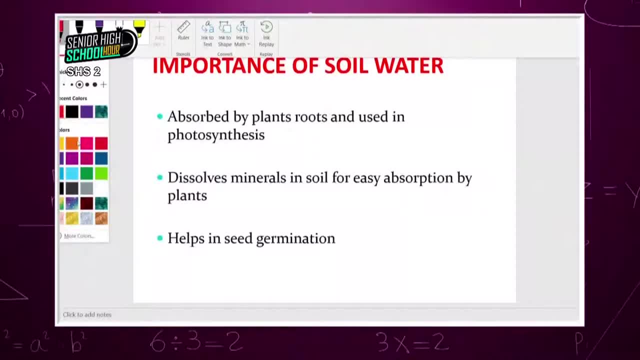 Let me write photosynthesis formula. Yeah, Okay, We have what? Carbon dioxide plus water, giving you your C6H12O6 plus oxygen. Then we put 666.. So the water, this water is the water we are talking about. 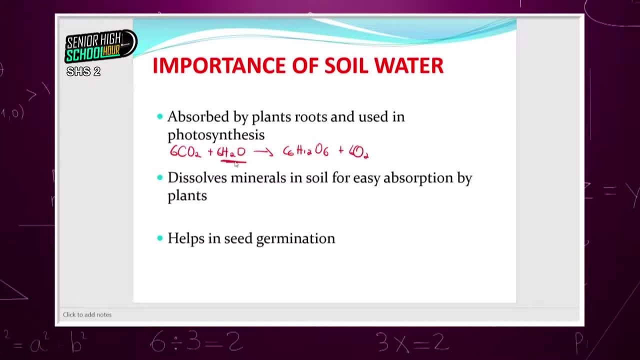 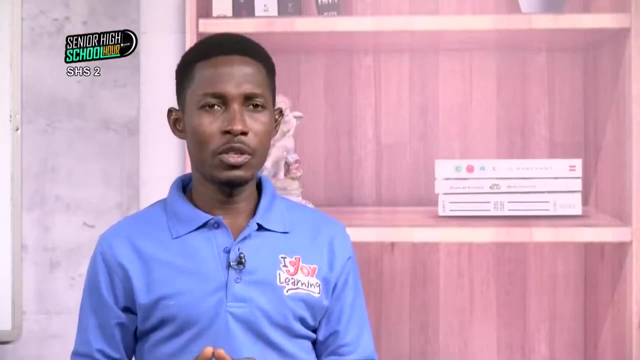 We pick it from the soil or the ground, Then the plant will use this for photosynthesis. The next thing is that I told you that there are a lot of nutrients in the soil. It may come as a result that the rock itself that formed the soil has nutrients. 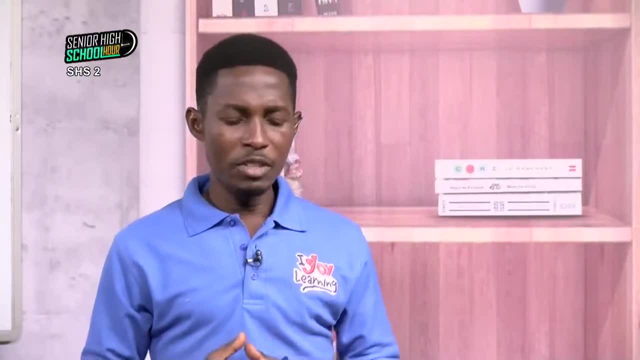 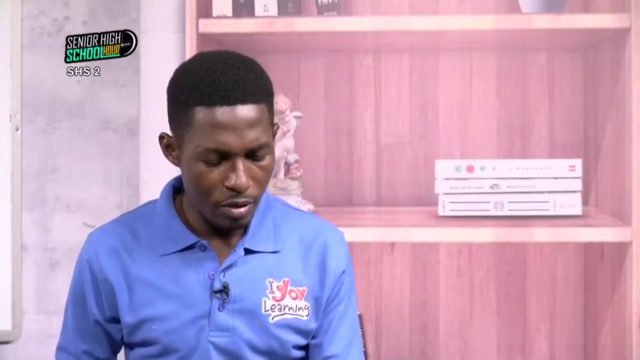 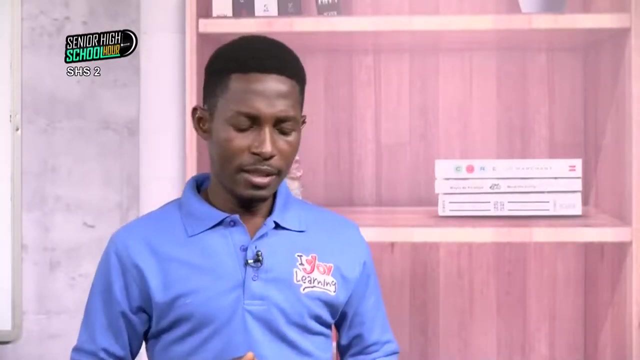 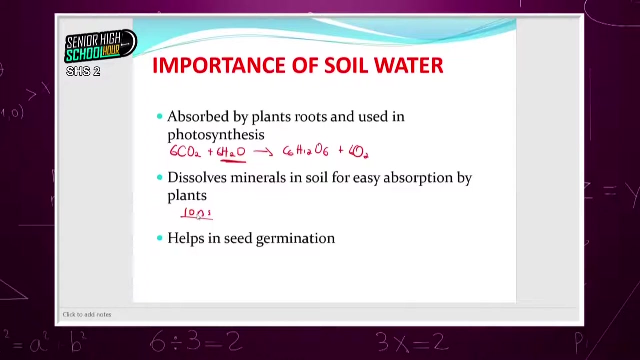 Or we decompose to add nutrients. But for these nutrients to be picked up, they need to react to the soil to form what we call iodine, So that it can easily be picked up by the plants. The same if you ever also observed any time farmers want to plant maize. 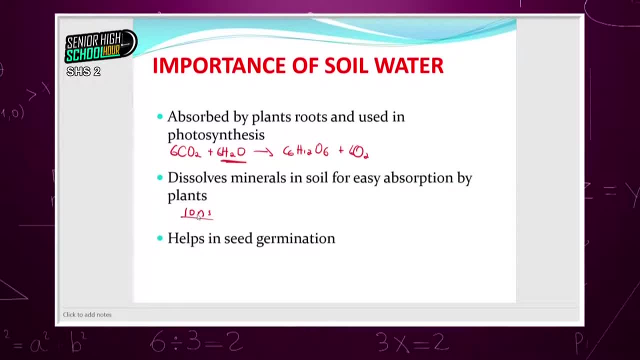 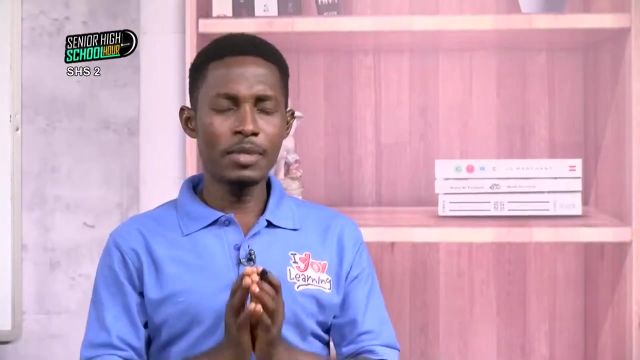 usually, for some reasons, they will soak the maize in a bowl for a day, overnight. Why do you think they do that? There's a lot of chemical reactions that go on in the seed, or the maize seed, To make it put in a certain condition that immediately put in the soil, it can grow. 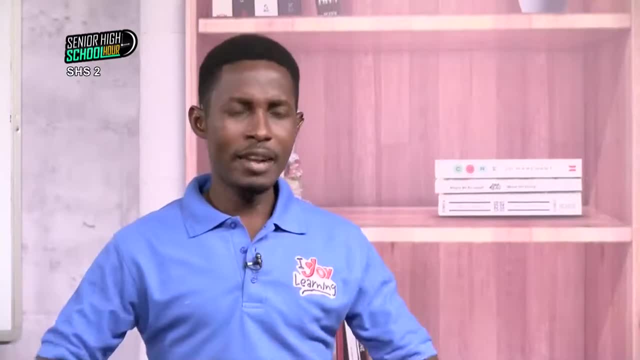 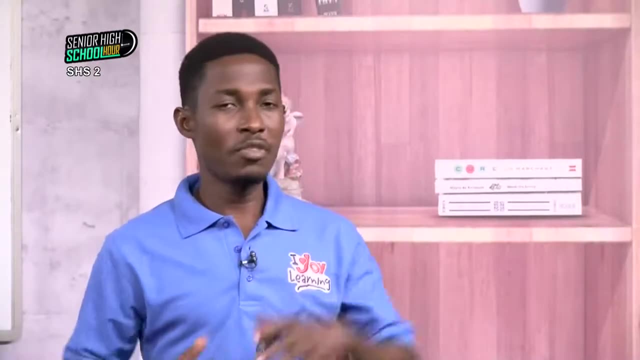 Also note that farmers, after clearing their plant, sometimes burning their farm, they wait for first rain, second rain or third rain before they plant. All this because they don't have enough nutrients. All this because they need water for a process in germination. 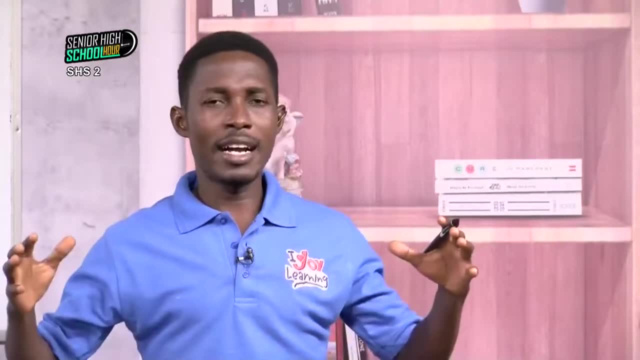 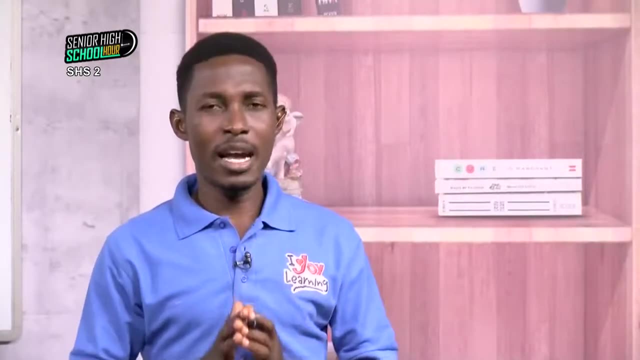 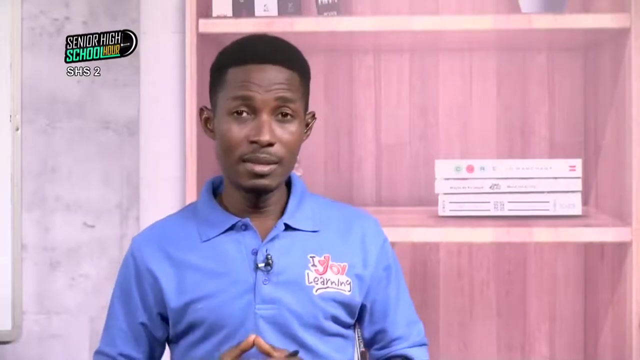 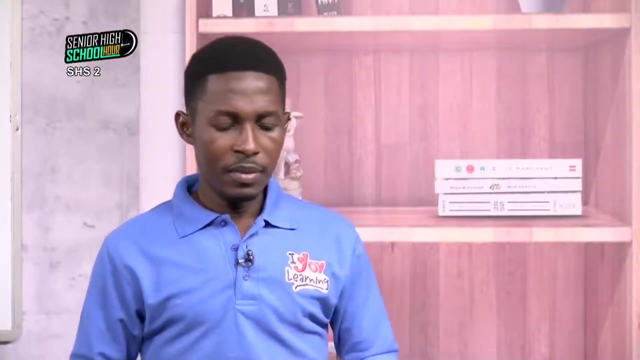 It will let the seed swell break cover to let whatever formed the seedling come out. But all this one requires some chemical reactions, and water does that. So if you see farmers soaking beans maize, there's a reason. Another is that they assist in plant fragility. 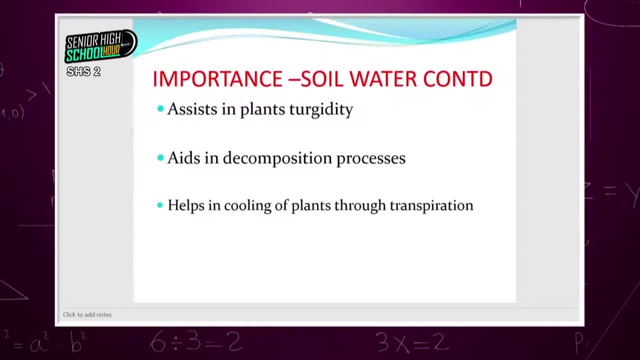 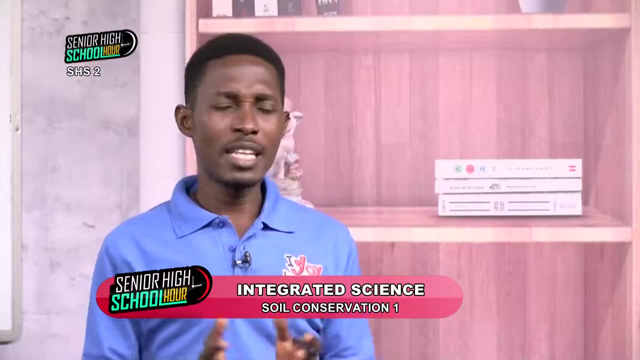 If you can experiment with this. if you have a small potted plant like pepper or tomato, mint, dandelion, try not to water it for some days. You will see that it will wilt, some burning down, curving some way. 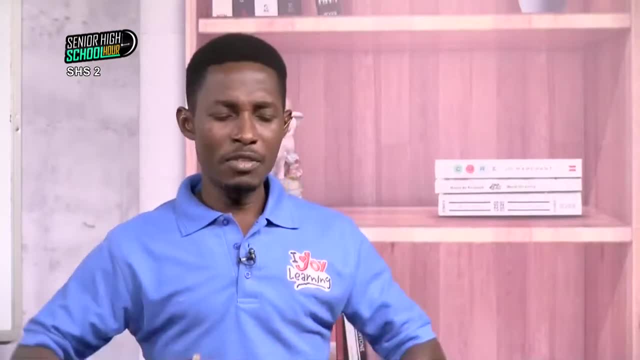 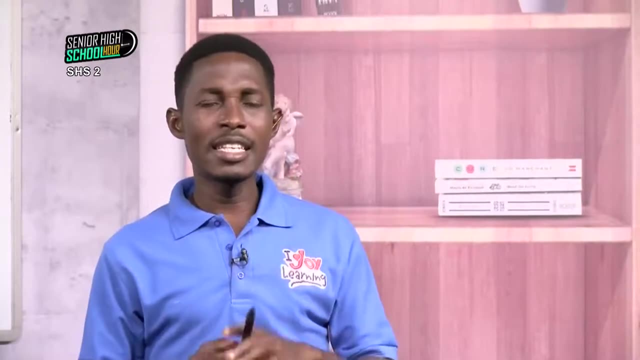 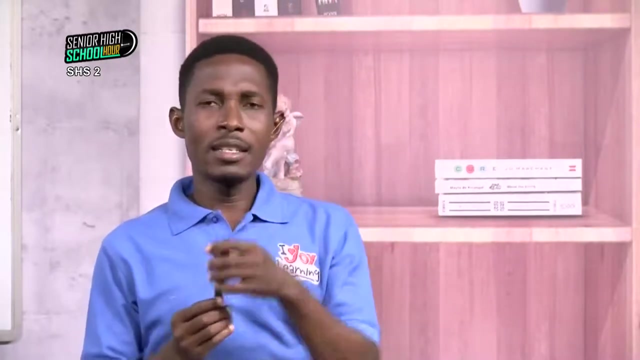 Yes, Now, immediately you give it water, it looks fresh and you see it's standing straight or erect. It is because the cells in there are like a set of pins fixed to each other. If one is fully filled with water it becomes bloated and we say it's turgid. 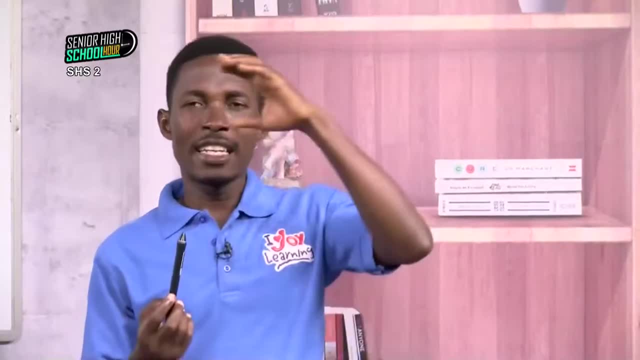 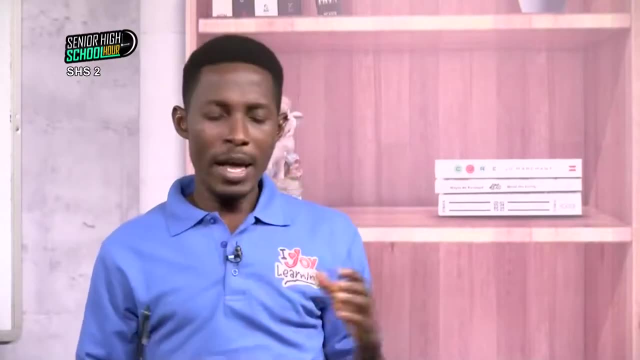 So the turgid one is full with water, it can support the next one who is turgid, the next one who is turgid. In that case the whole plant can stand erect. But all of a sudden, if there is no water in them, they will shrink or they will reduce in size. 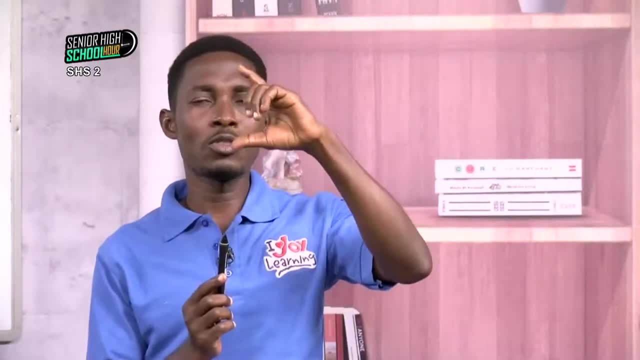 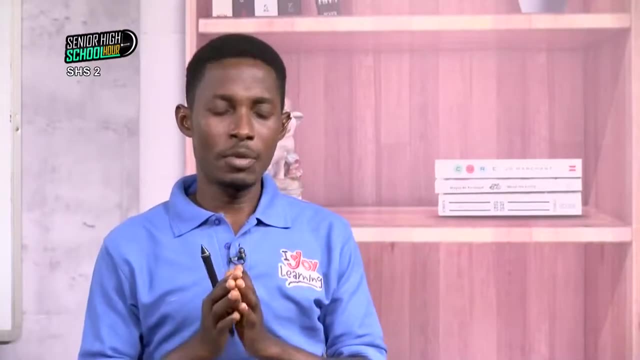 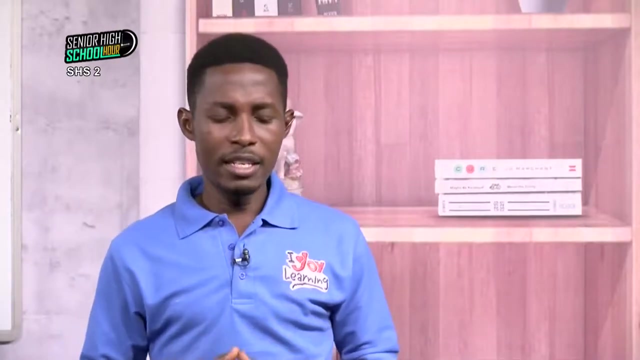 So if I reduce in size, I cannot carry you the one on top. You're also reducing in size. In that case the whole fixed nature or turgid nature will shrink and we say: the plant wilts The same water. we are talking about aids in decomposition processes. 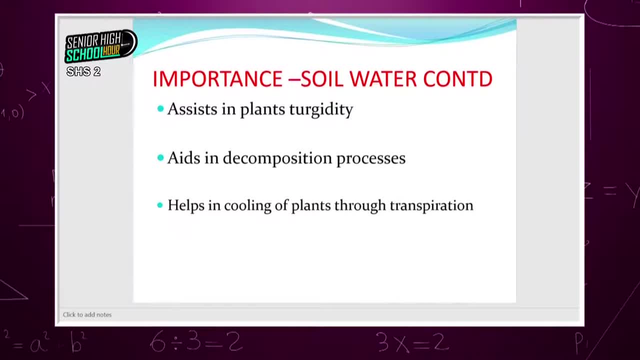 I told you that when we die, the microorganism needs to decompose our body. But water- if water is around and there is enough warmth or good temperature, the rate of decomposition is high. So we are saying that the water that we see, or rains that fall onto the soil, 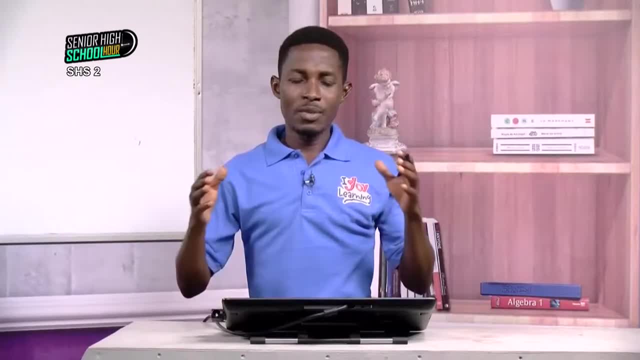 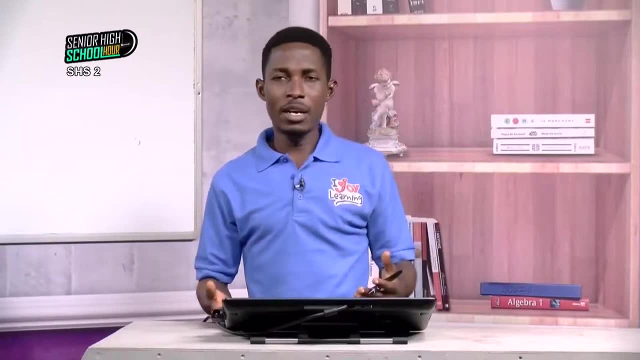 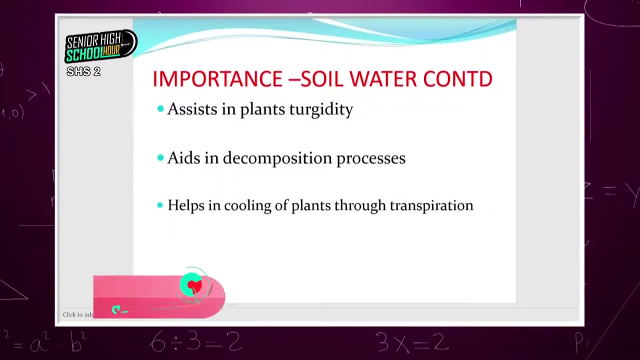 knowingly or unknowingly, there are plants that live on the soil. dead animals on the soil or in the soil will need to be decomposed. The microorganism is already there. The water will come in and a good temperature will come in. 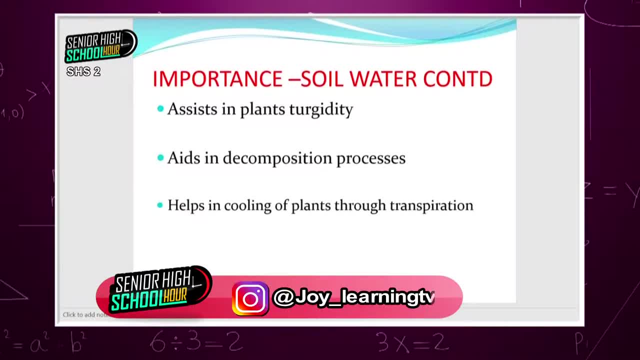 so that the rate or how fast they want to decompose is achieved. And the last one, and the last point is that they help in cooling of plants through transpiration. And what do you mean by the word transpiration? Let me simplify it. 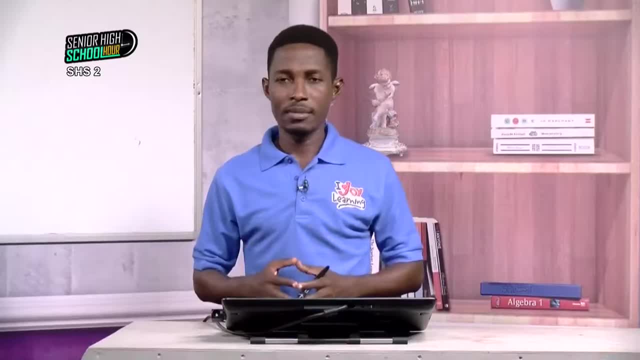 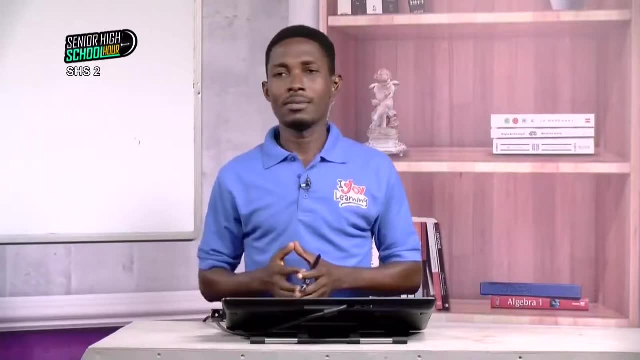 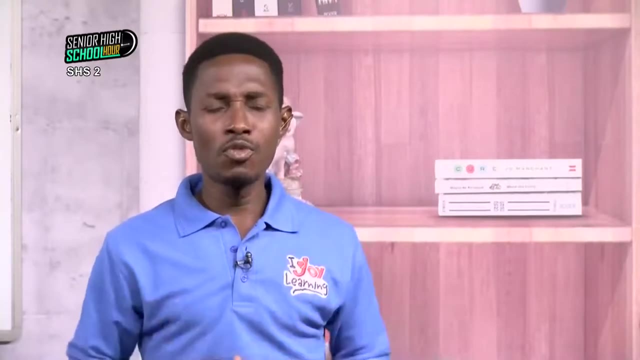 Human beings do what Sweat, And when we sweat onto our skin it evaporates. It's like doing what comes from your mouth. like the steam, Plants also have a means that, when they are filled with too much water and they are in the day and the sun is up. 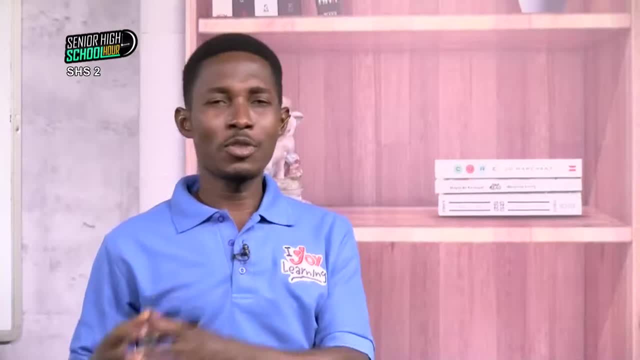 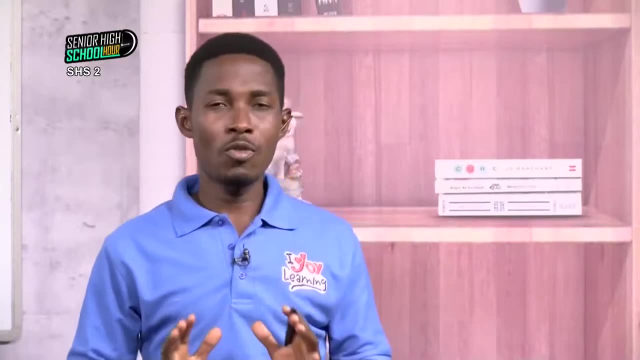 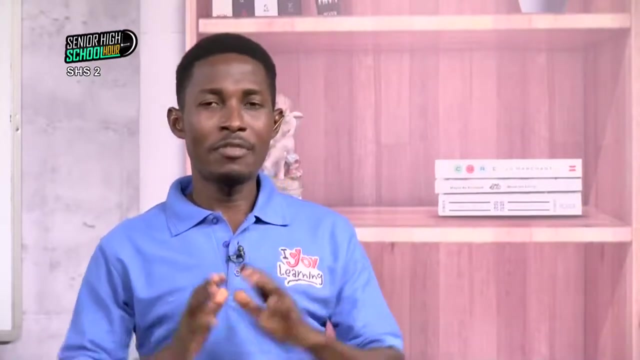 and they feel like sweating. What you call sweating? they invariably call it transpiration. Transpiration is just the loss of water in the form of water vapor. Yes, the loss of water in the form of water vapor. So when we also sweat here, 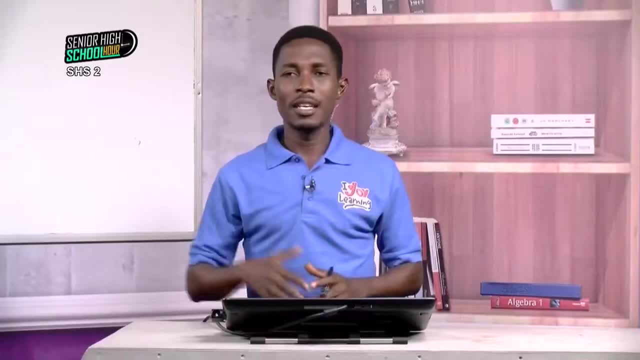 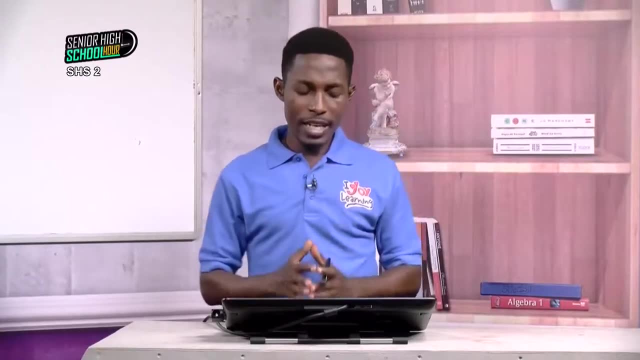 from our skin in the form of vapor to the atmosphere. In plants we are calling it transpiration, In humans we are calling it evaporation. So we say that anytime you sweat and sweat leaves your body, you see that your temperature. 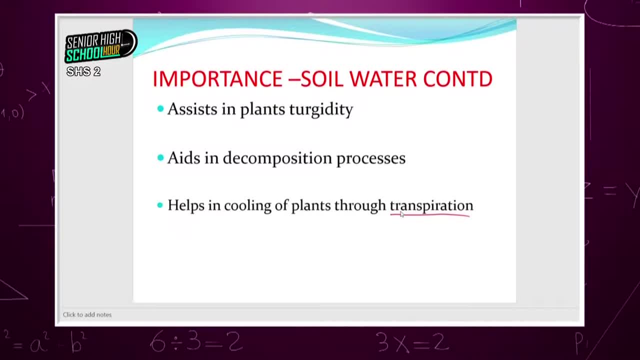 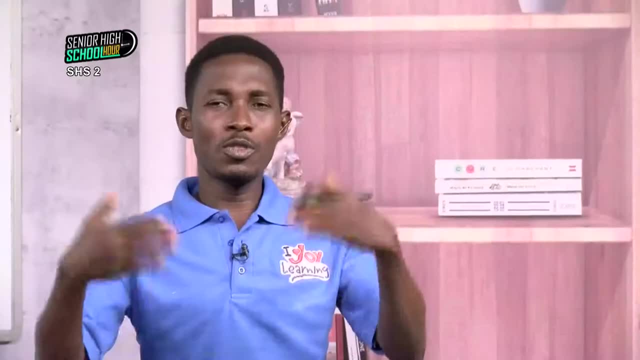 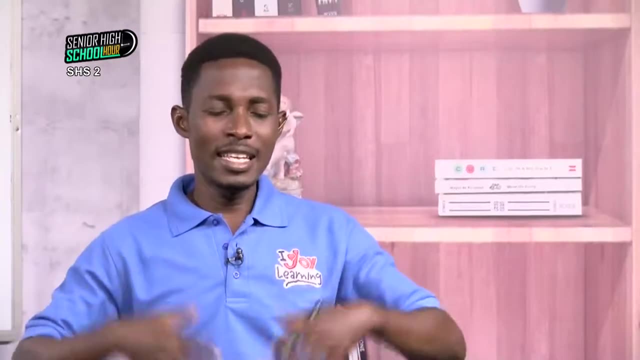 the hotness in you has been removed by the evaporation, So your temperature cools down again. Plants are like you, So when they also transpire and they lose the water in the form of water vapor, it makes the heat inside of the plant calm down. 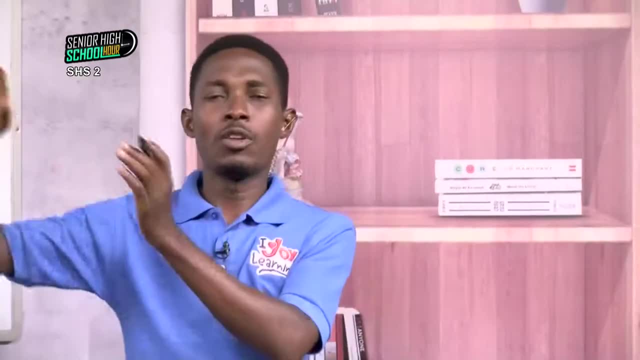 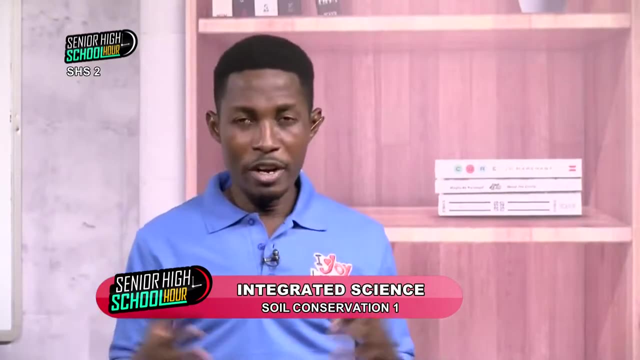 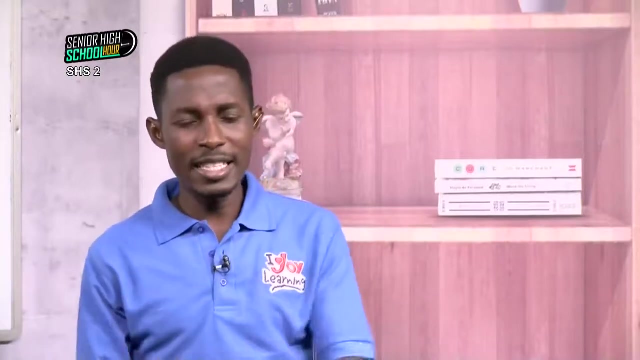 Because the heat accompanied the water and they were lost together. Try on your own, too, When you feel very hot. one means of reducing your temperature is when you urinate. Imagine you urinate. you see some heat leaving, because the heat came with the urine. 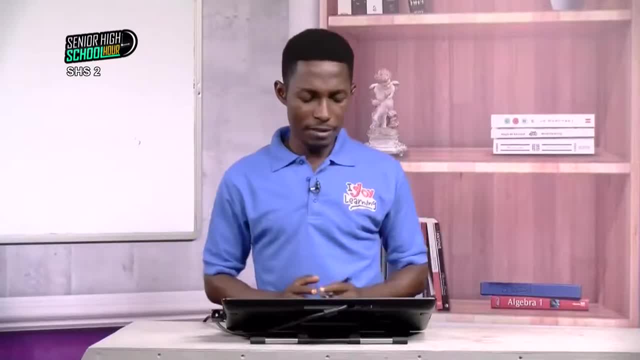 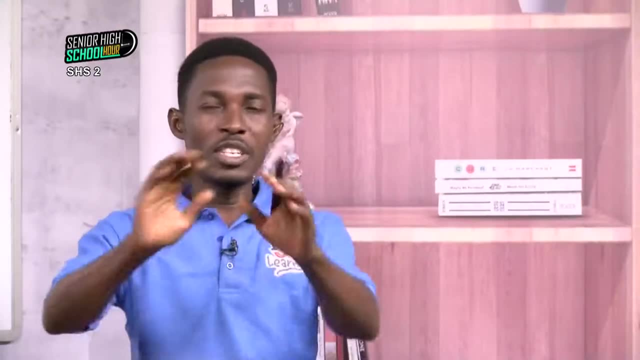 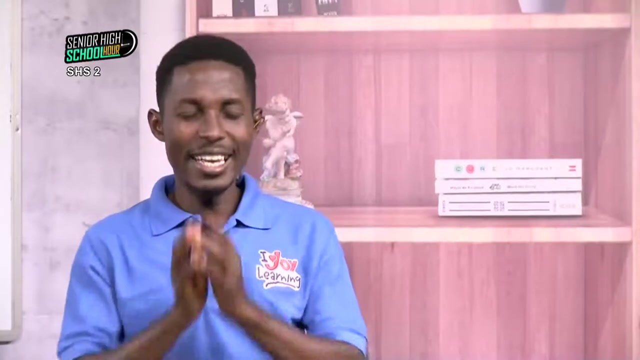 And that's the same idea with transpiration. We are on soil and the soil water conservation. I just told you what we need: soil water for A lot of functions, So the plant need it almost every day, every time. Like you, you also need water. 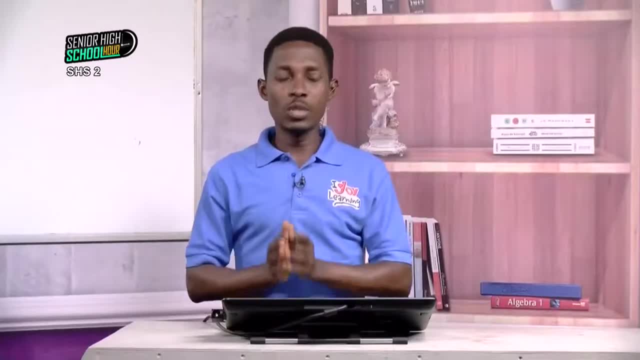 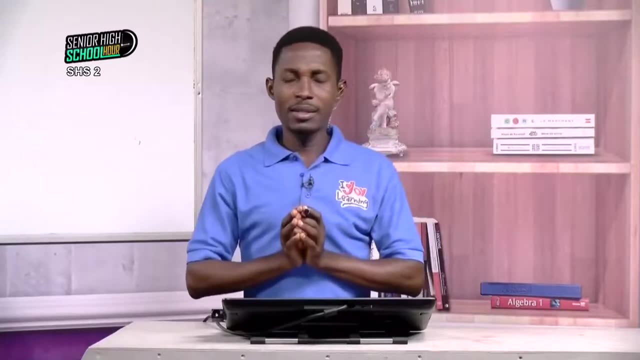 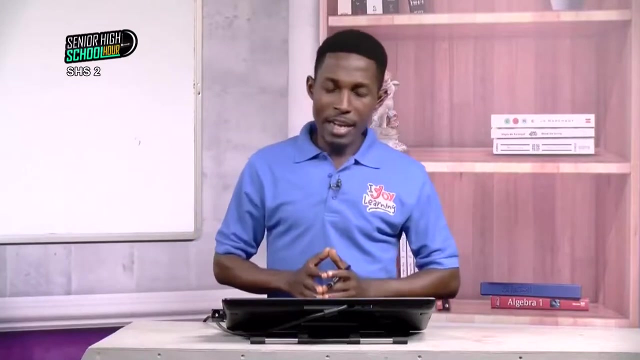 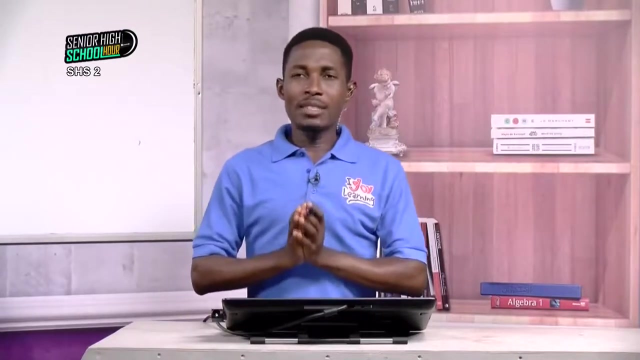 But certain things can let us lose this water. So we have to put in practices that will prevent the carrying away of this soil and soil water, And they are rather referred to as soil and soil water conservation. So our practices should prevent first erosion, soil erosion. 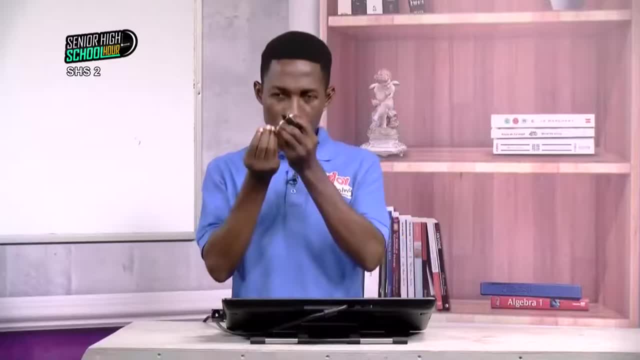 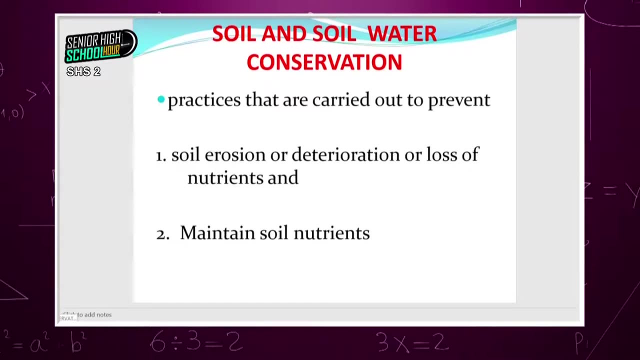 And when we say soil erosion, any means by which the soil particles on the surface of the land is carried from one place to somewhere- It can be carried by wind, or it can be carried by rain or water. We want to prevent that Also. we also want to prevent 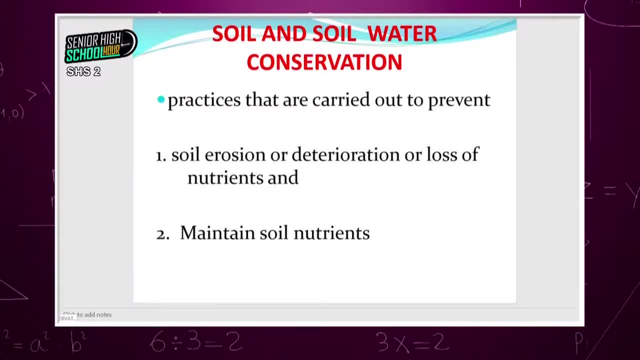 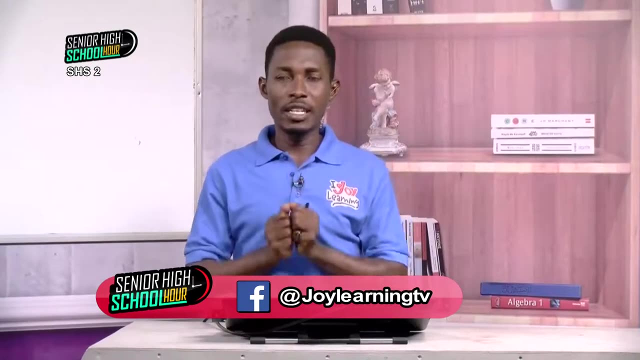 the loss of soil nutrients. So we say maintenance of soil nutrients or preventing soil loss, soil nutrient loss. I've shown you how we get nutrients. The soil itself is a nutrient and the things that decompose and adapt are nutrients. We want to prevent the loss of these two things. 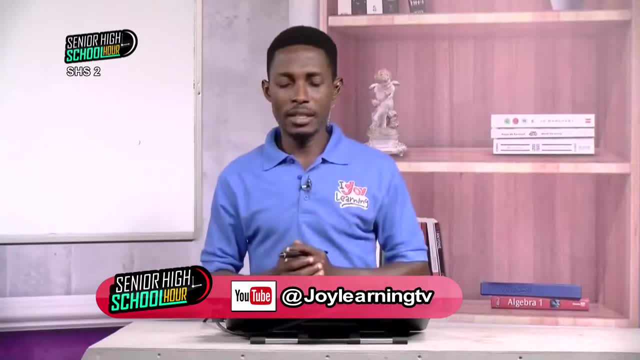 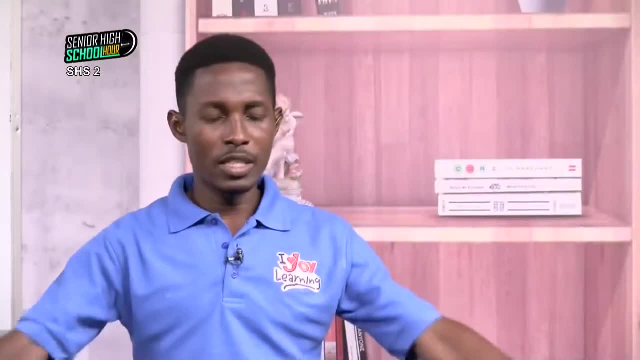 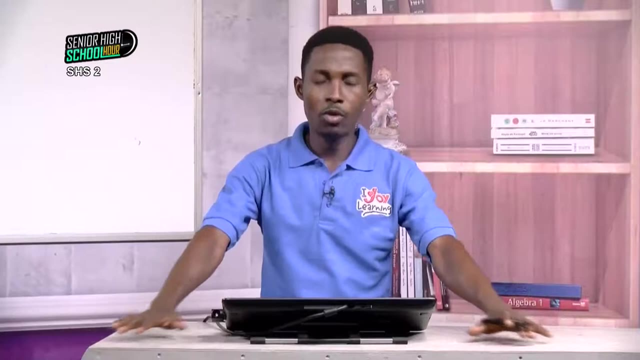 Let's see how we can prevent it. Let's brainstorm and think deep. Imagine this platform is full of water. It's full of sand or soil, any form, whatever you know soil, Loamy, clay or sandy soil Here. 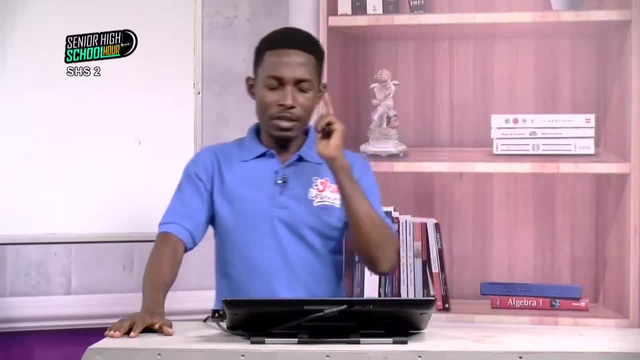 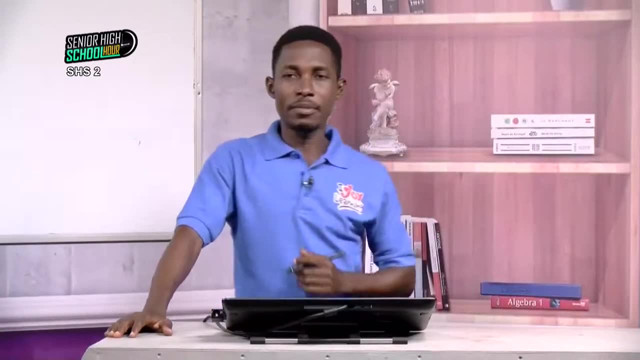 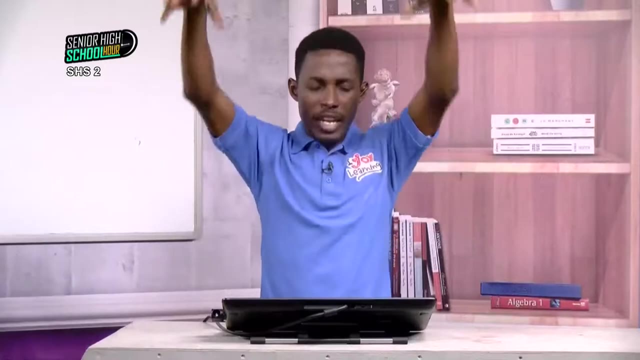 And I said we want to prevent what Erosion, Erosion which will carry some away or the nutrients being carried away. So what are the means we will carry away If it rains and it can touch this place or touch the soil? 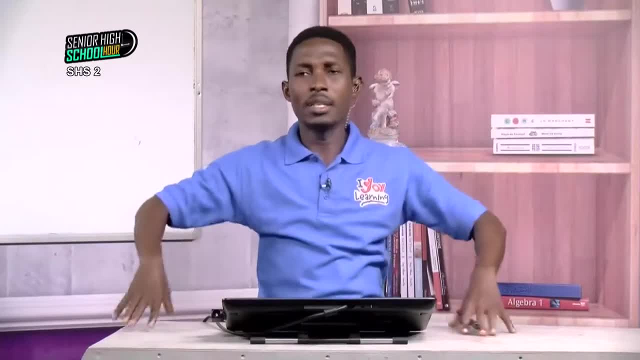 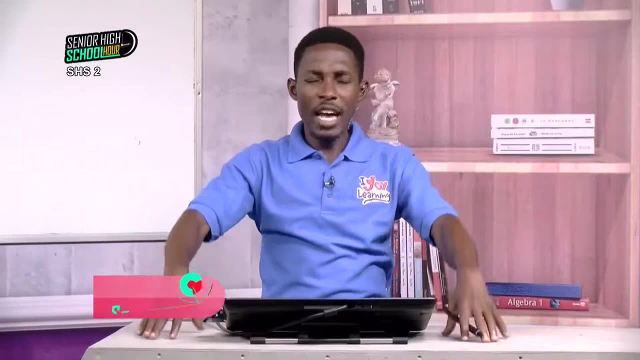 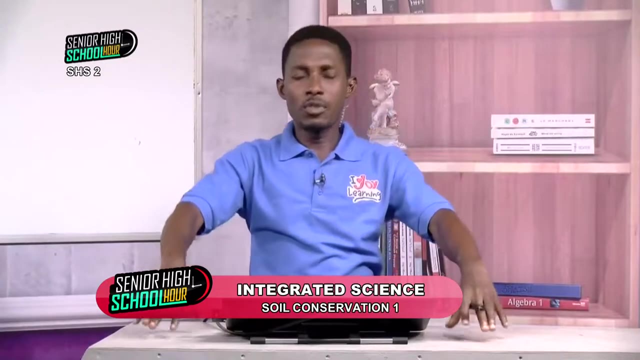 it will disperse the soil from where they are to another place. So with this, then, the first thing we are supposed to do is try to prevent this rain or the water from touching the soil, Or even if it will touch it, prevent that the impact is not so much. 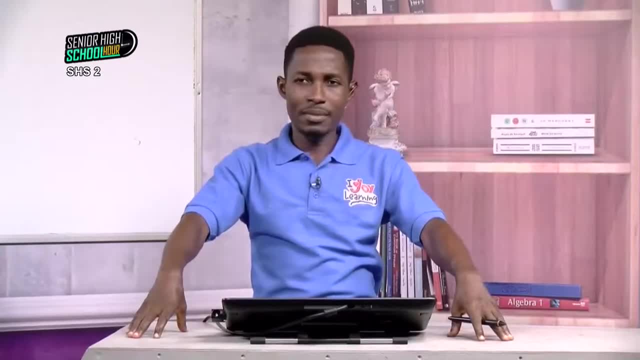 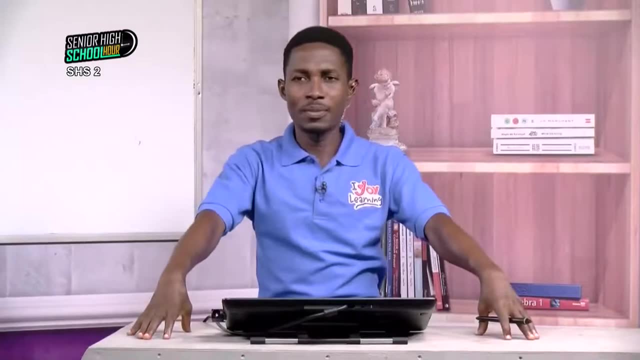 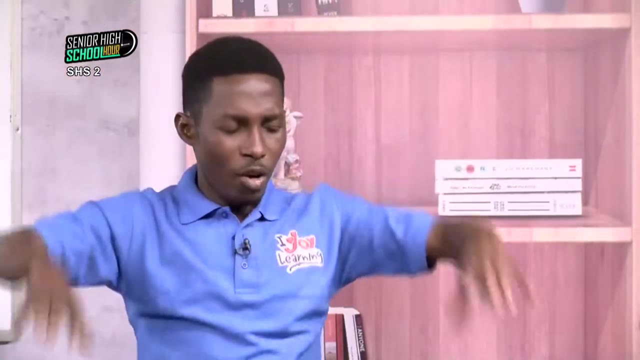 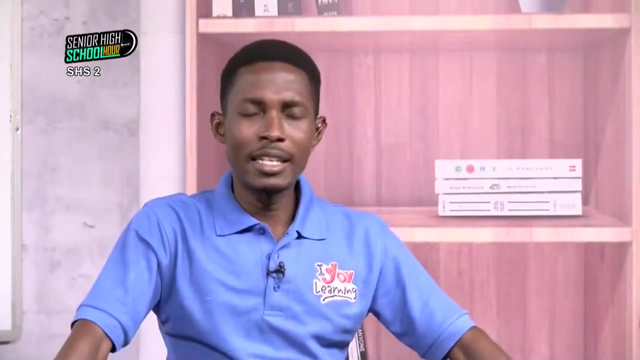 that it will carry it away at a top rate. Yes, So what do you think we can do if we want to prevent the heavy downpour of water onto the soil so strongly that it will just splash it and carry it away, like you see, under heavy rains? 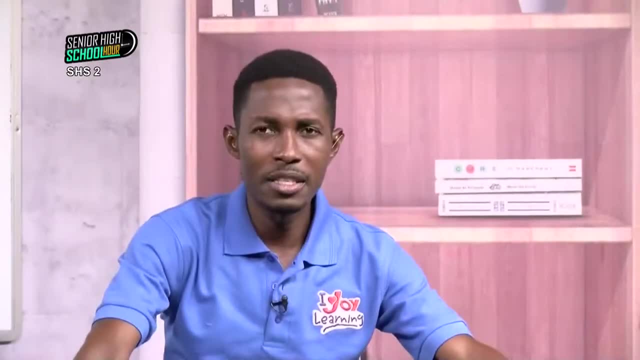 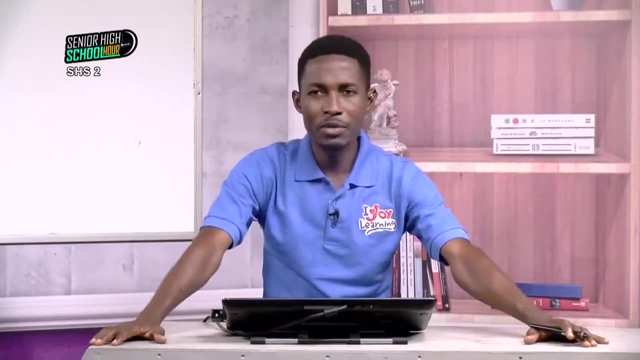 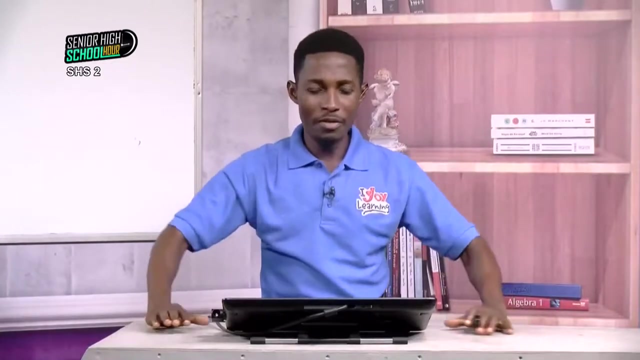 So the first thing could be: then let's cover this place. If you don't want dust to fall on something, what do you do? You cover the place with something. Yeah, So, covering the place with something in terms of soil, covering the soil with something. 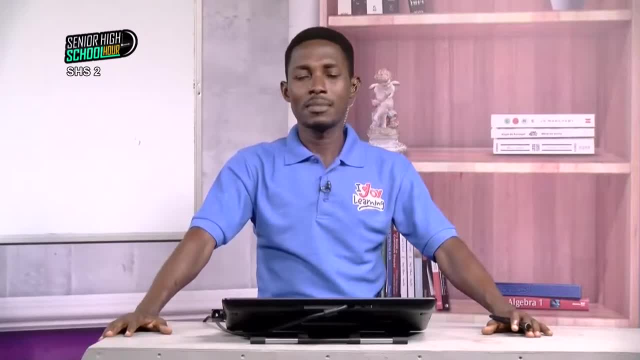 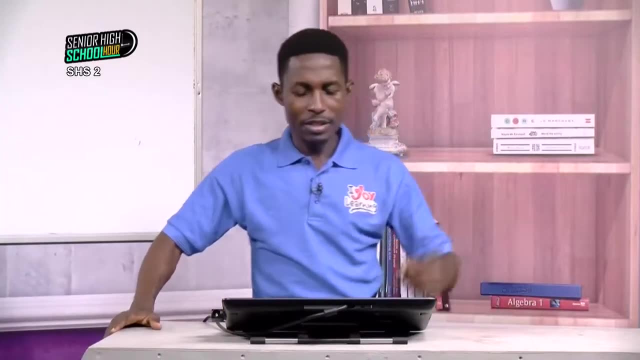 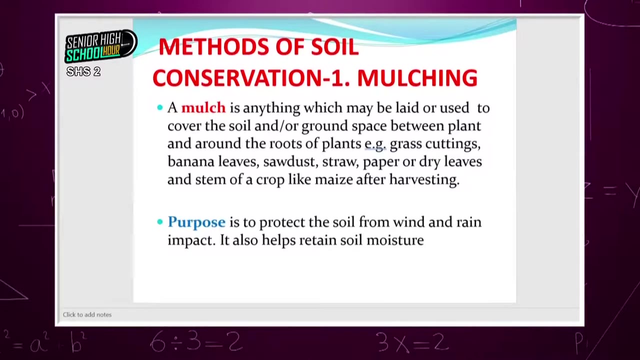 is what we term as mulching. Whatever you want to use to cover the soil surface, it's called mulching. So let's look at mulching methods of soil conservation. So a mulch is anything which may be laid or used to cover the soil. 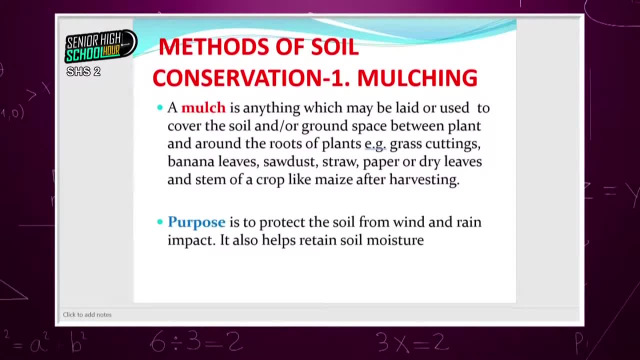 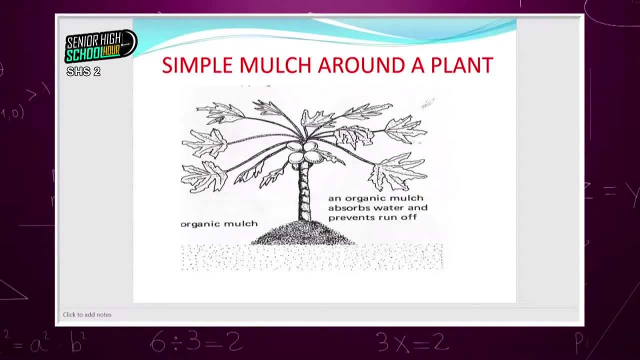 and or ground spaces between plants and around the root of plants. Let me give you a picture of this, So you see that under the plant we have something like you can say grass, whatever material has been used to cover the base of the plant. 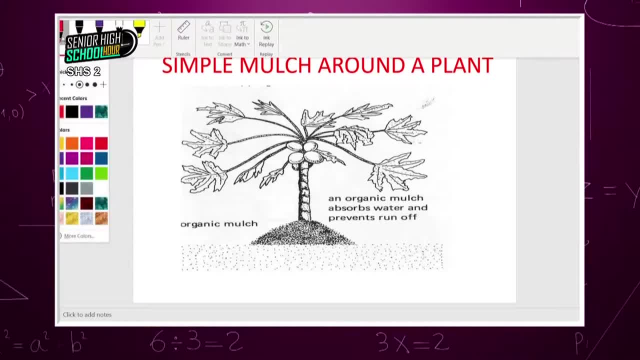 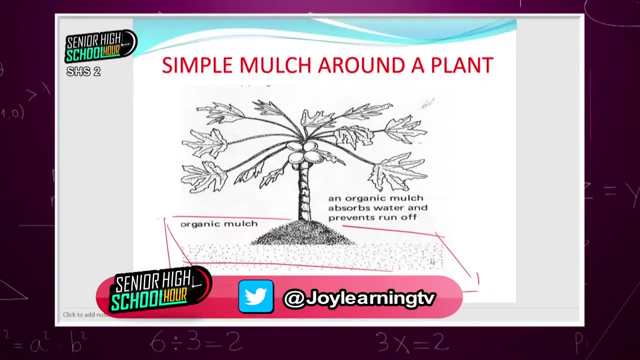 We could use it to spread the entire area. like this, You can use it to cover this whole area, But that would be difficult. The reason I'm showing this: if a farmer has a huge land, it may be difficult to cover the whole land. 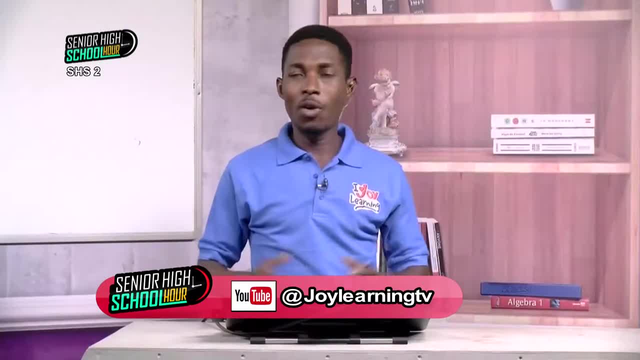 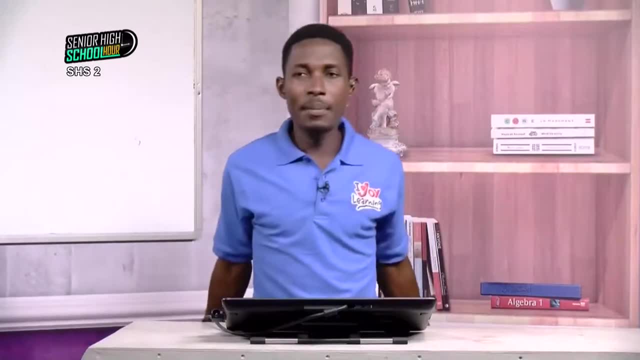 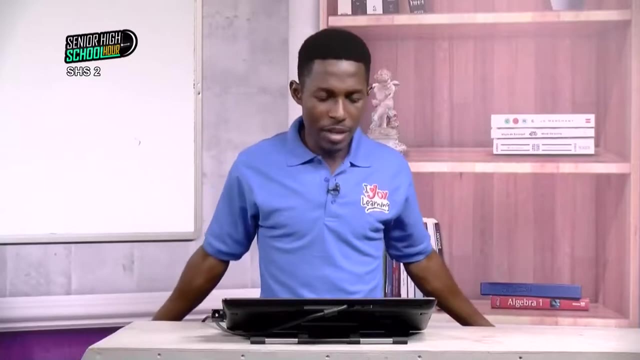 with maybe a rubber or grasses across. So some prefer to do it just at the base. But if you see them using rubber, a polythene, to cover the whole surface, they are doing mulching. If you see them spreading grasses, 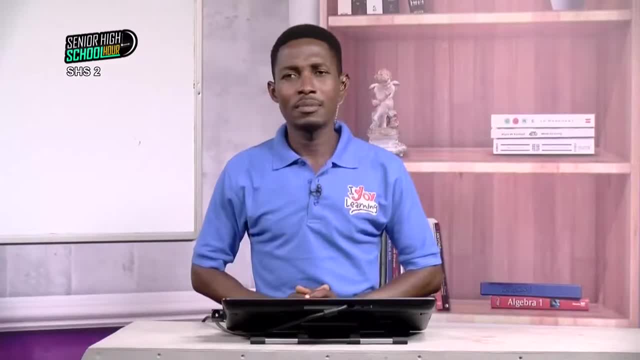 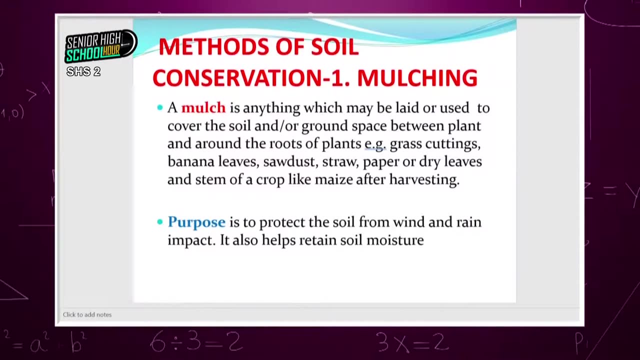 on their farm they are also doing mulching. So mulching is just when we lay anything, the word is anything that can cover the soil surface or ground space between plants and around the roots of plants. So we have banana leaves. You go to the village. 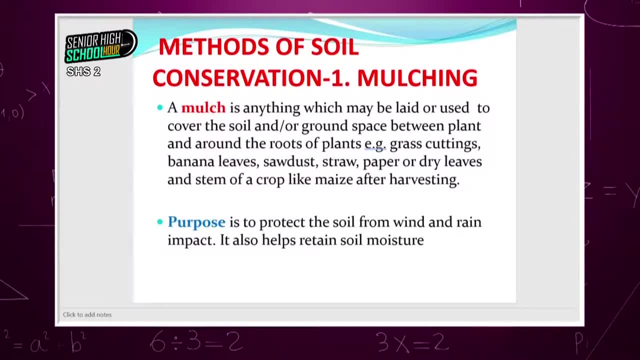 you see them cutting banana leaves to cover the soil. We have sawdust that they spread, paper or dry leaves, straw, grass cartons, then stem of some crops like maize. When they finish harvesting they just cut it and leave it. 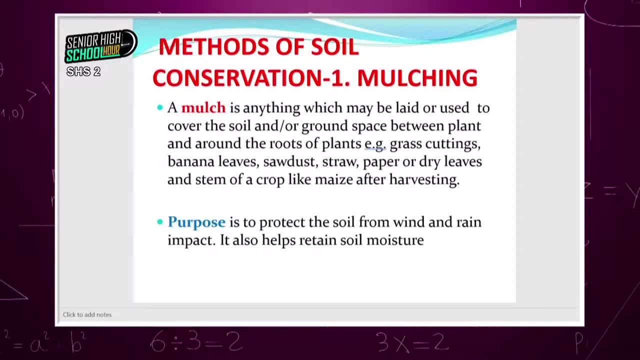 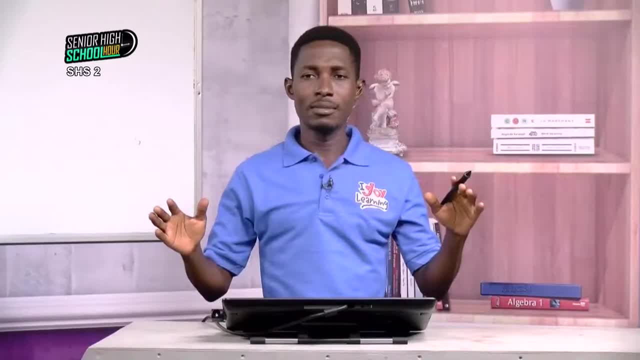 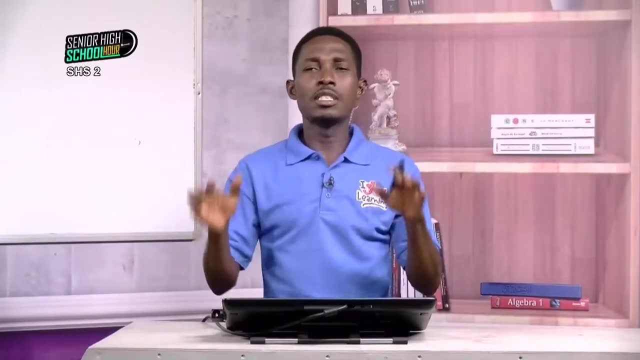 on the surface of the land. What they are doing is also mulching, Because after harvesting, if they should burn immediately, they will expose the land, So they will cut and just leave it in crisscross fashion. so when it rains, it reduces the impact of the rain. from touching the soil. Then, as I said, the first aim is to reduce the impact of the rain from touching the soil. The second aim is to retain soil nutrients and soil moisture. Yes, when we cover it the scorching sun. 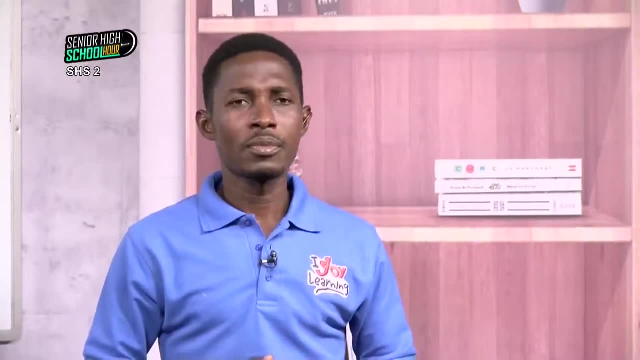 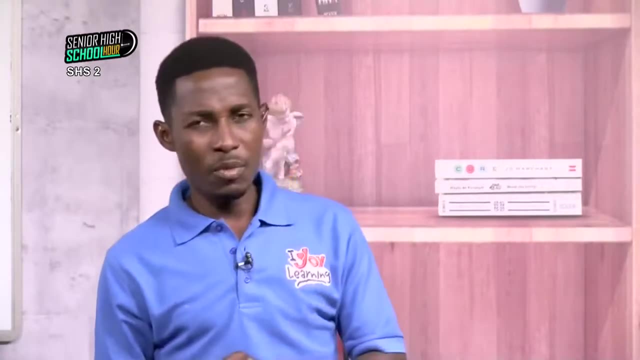 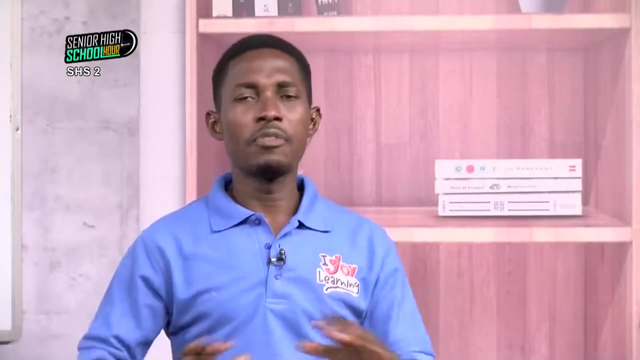 will not get access to the soil, Because if they get access to the soil they will evaporate the water in them. They may even kill some organisms and also destroy some nutrients. So when we cover it we prevent these conditions or these actions. 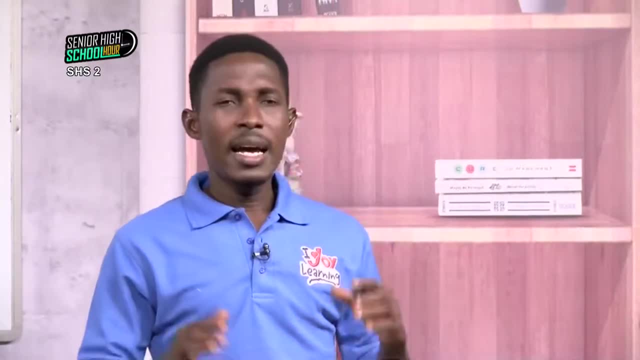 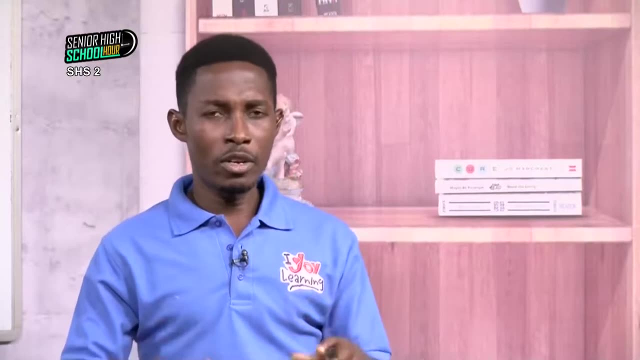 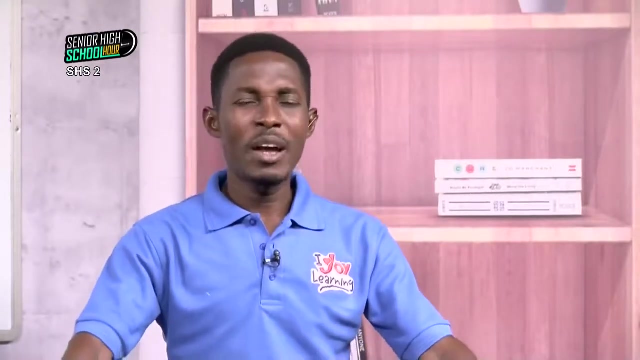 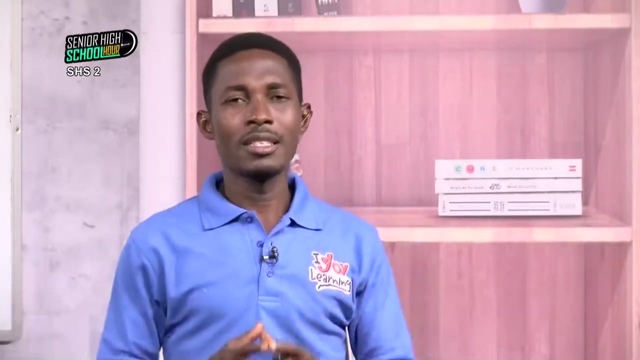 from taking place. Another means of preventing soil and soil water from being lost is that if you have a mulch, that can be artificial or natural. But if you want benefits, what do you do? You would rather grow a plant that has probably a broad branch. 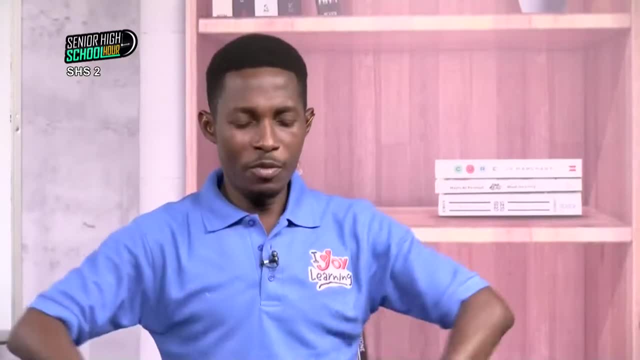 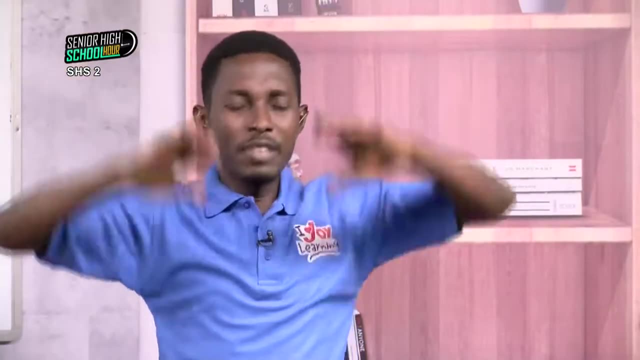 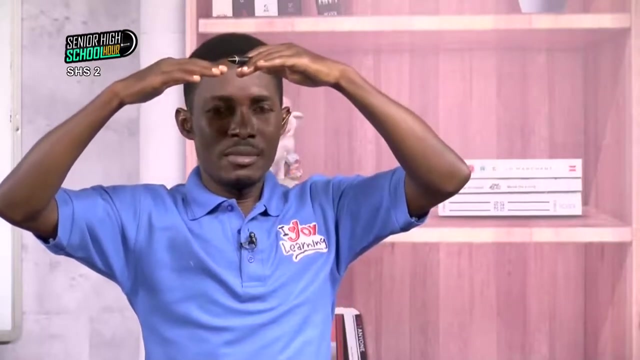 with many leaves, so that what we should have covered on the ground than we are doing at the top. So, before the rains even get to the ground, we have reduced the impact of the speed and the strength of the rain from getting to the ground. Though it will come, the leaves and the branches will take the heavy beating first and slowly let it trickle down at a lower rate. The same broad branches and leaves can also prevent the sun, the scorching sun, from destroying the soil. So what we are saying? 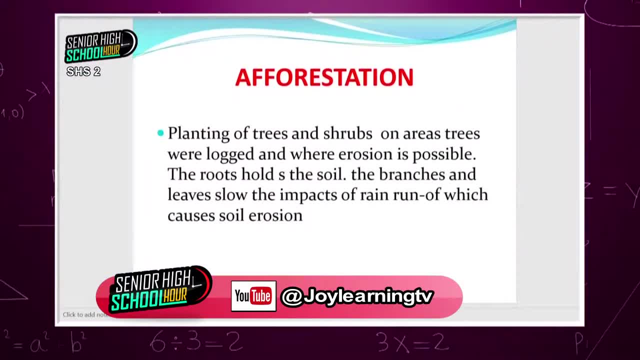 is what we term as afforestation, Planting trees- I used the word trees when I was talking- and straps on areas where trees were logged and where erosion is possible. When we do that too, the roots of the plant or the tree will hold soil together. 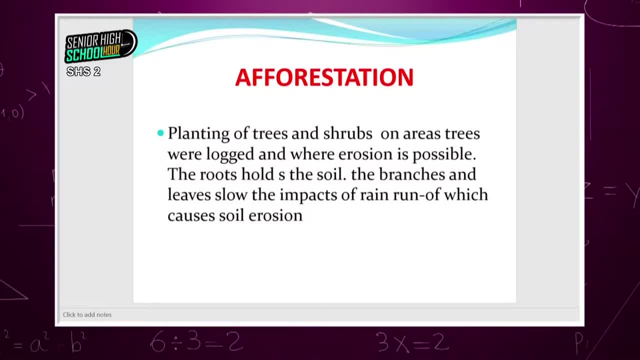 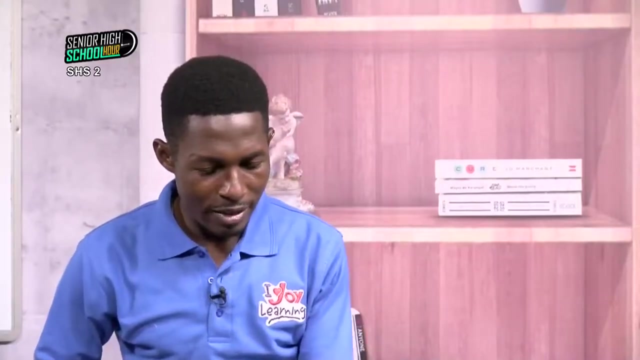 Like I said, the branches and the leaves will slow the impact of rain runoff, which can cause soil erosion. Another form of afforestation, this time not trees, because the word afforestation has the idea of trees in the forest, So there's something like: 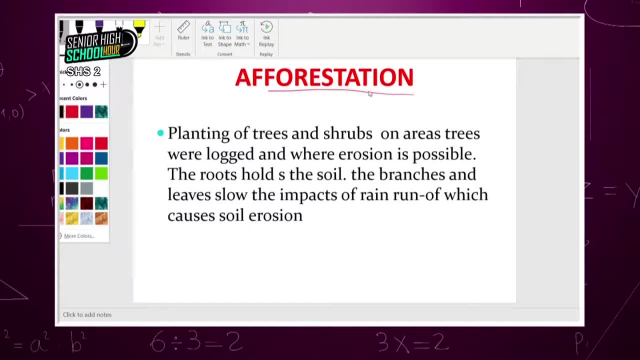 forest in it. Watch this word forest in it. So it's like growing forests are mostly made of trees and few low plants, But we are going to what the farmers usually do Instead of planting trees that the next day they need to cut down. rather, the farmers will prefer to plant crops or plants that are very close to the ground, like granite beans, those with broad leaves that are also close to the ground. These kind of plants are called the cover crops, because these crops will cover the surface of the land for you. 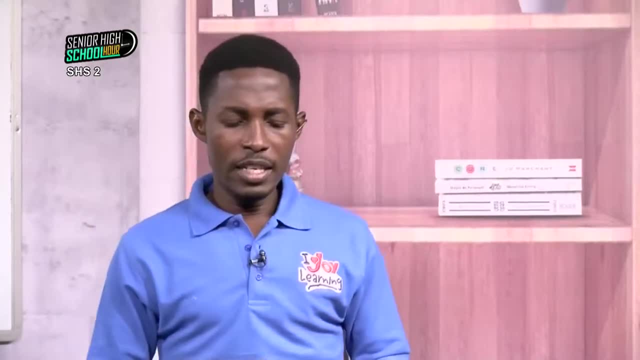 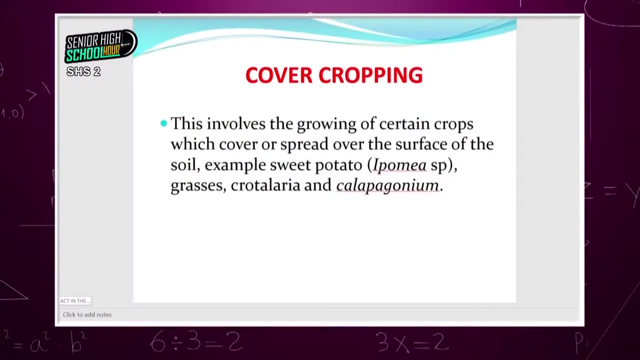 So we say this involves the growing of certain crops which cover or spread over the surface of the soil like sweet potato. It's one creeping plant that before you realize, the whole place is covered by the sweet potato. We have your normal grasses, the ranes. 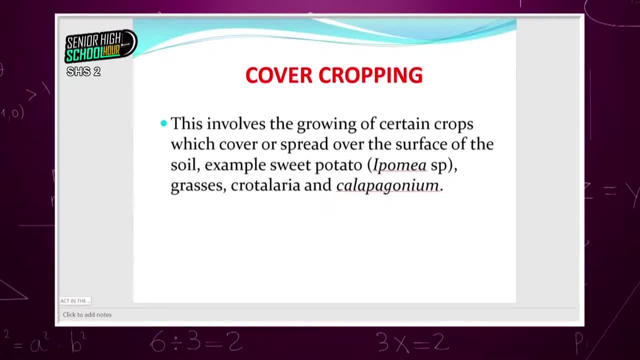 the green grass we have. they are always around you, These plants. what it does is that first, the roots holds the soil together. Roots hold soil together. What again can you add? Let me give you the answers. So we say: the root holds. 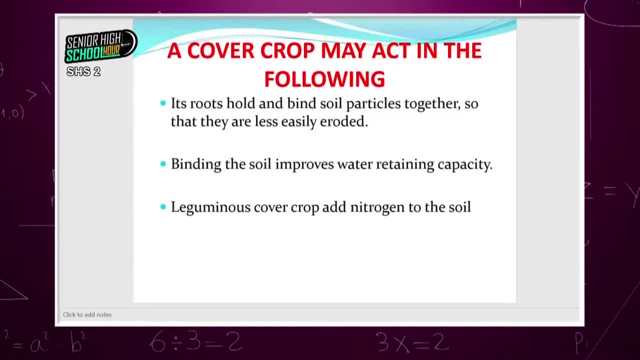 and binds soil particles together so that they are less easily eroded or dislodged. Another is that binding the soil together also improves the retaining capacity of the soil. What are they retaining? They are retaining water. Yes, If the soil is loose. 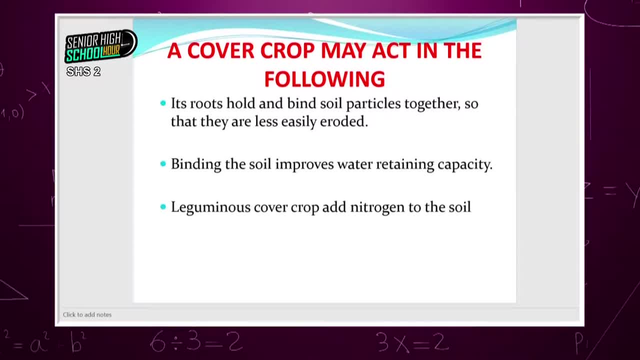 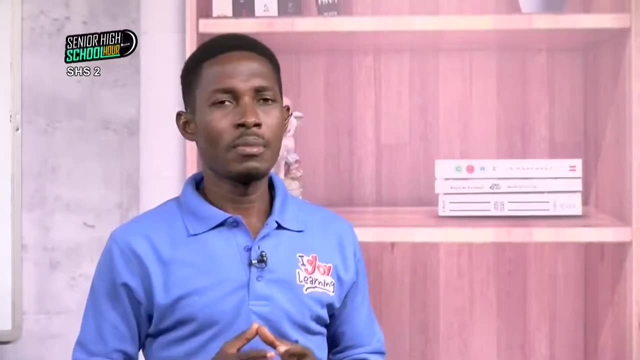 and we plant a cover crop, most of the particles of the soil will grow around the roots, As they do so whenever it rains. water will not easily pass through immediately and be leached or drained to the water table, But rather they will take enough days. 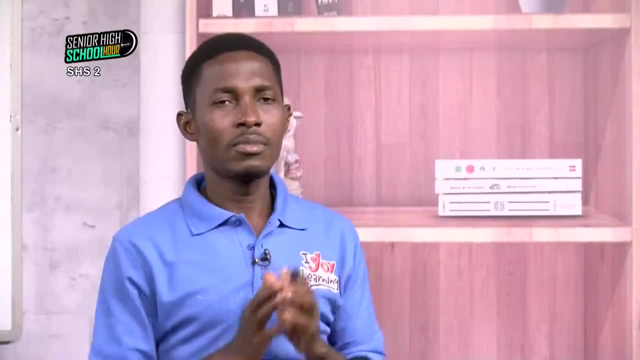 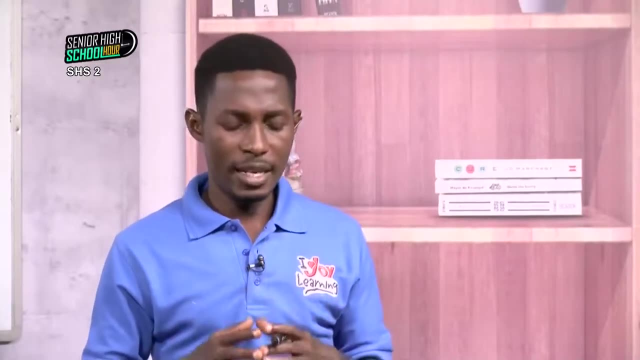 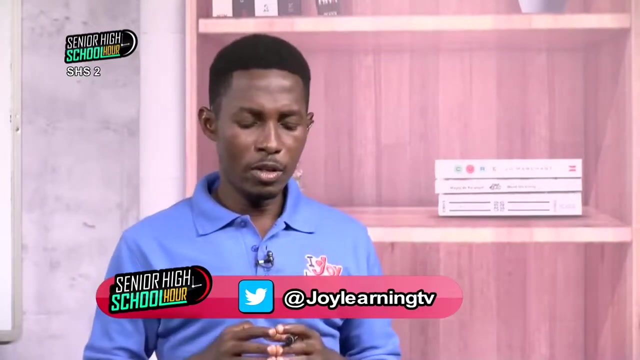 to stay and, at a good rate, drain off. So we are saying that the ability to hold it for some time is what we call the water retaining capacity. In addition, some plants which are called the leguminous plants, after performing all the other functions, 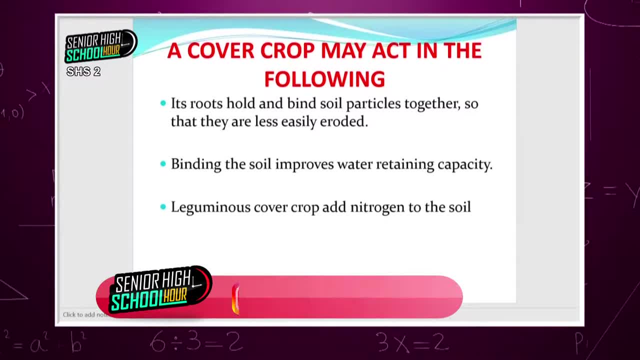 they have the ability to have a relationship with certain bacteria in their roots, And the process will lead to they taking nitrogen from the soil, from the atmosphere, converting it in a certain way, giving some to the legume plant and releasing the rest to the soil. 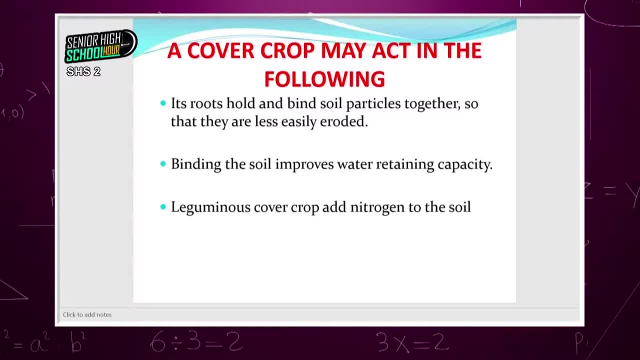 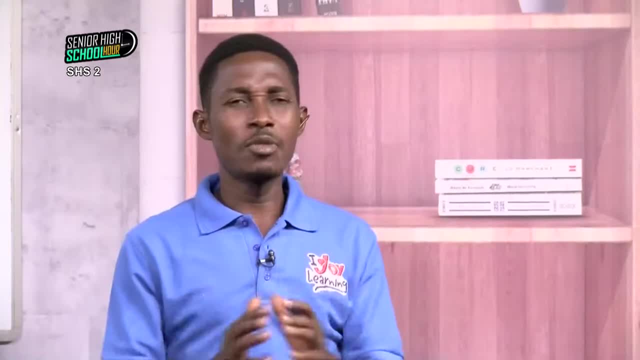 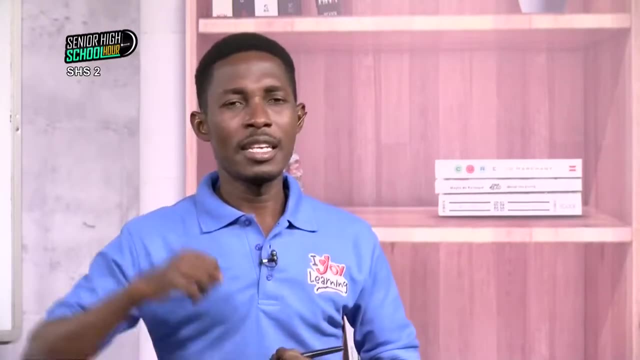 So a soil that is lacking a lot of nitrogen. the best way is don't go and do it the artificial way. Just plant leguminous plants and they will trap some bacteria, go through a process, get the atmosphere nitrogen, share it into two. 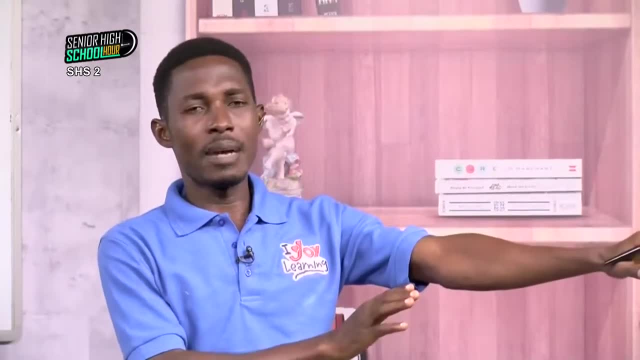 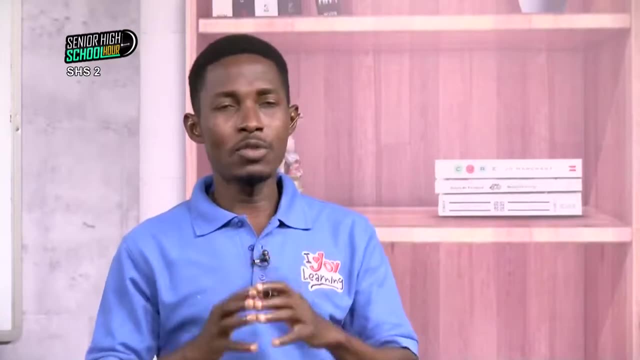 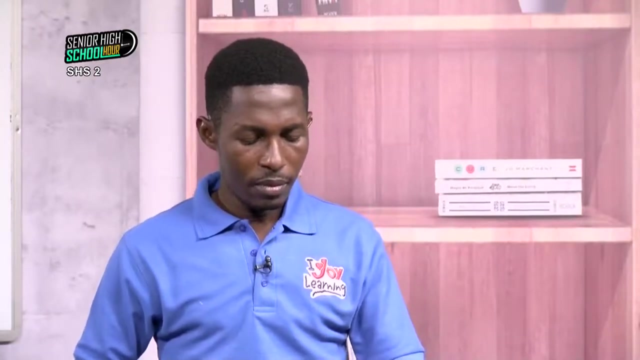 give one to the plant and the bacteria itself and leave the rest in the soil. Very soon the soil then becomes tends to have a lot of nitrogen in them. Now we have also said that e-leaves are so broad that when the rain falls on it, 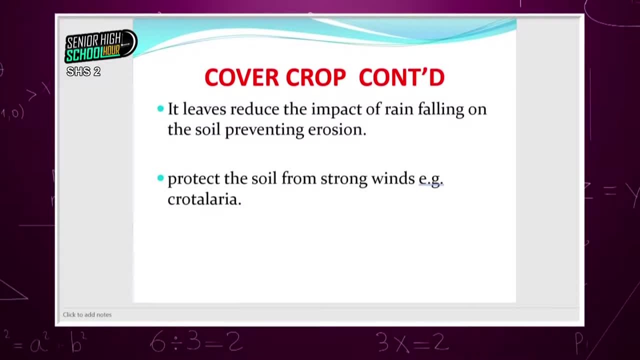 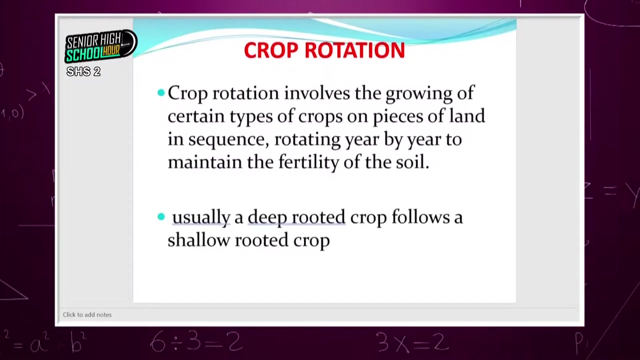 its impact is reduced. The same thing, the same thing. leaves can also protect the soil from strong wind so that they don't face erosion. Another approach to conserving soil and the soil water is what we call the crop rotation. We define crop rotation as: 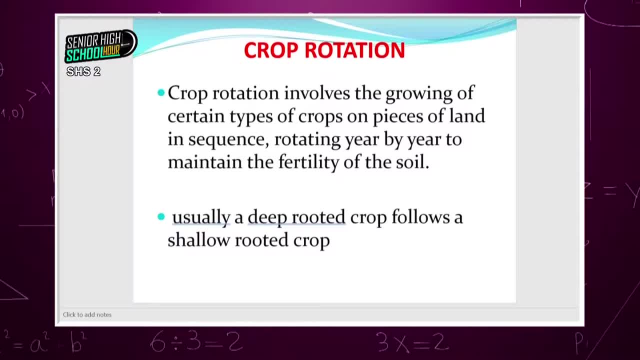 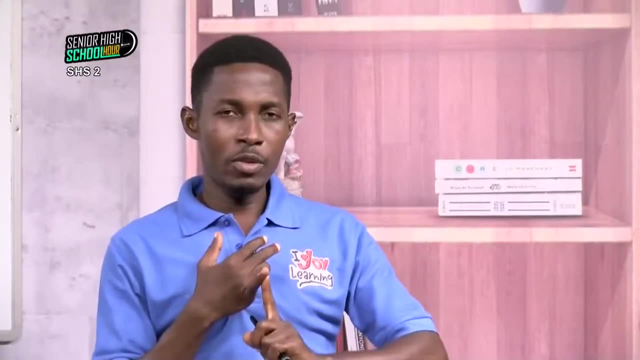 a process involving the growing of certain type of crops on a piece of land in sequence, rotating it year by year, so that we maintain the fertility of the soil. Remember we are preventing two things: loss of the soil particles by erosion, and also maintaining the nutrients. 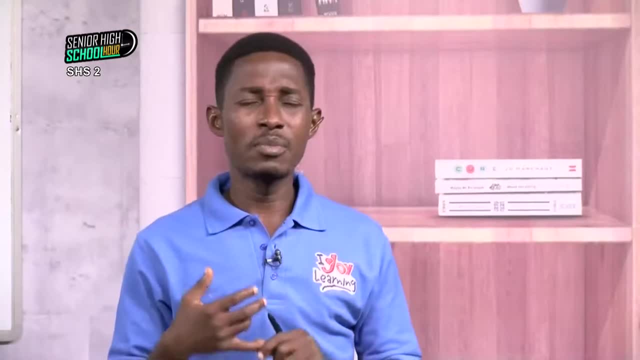 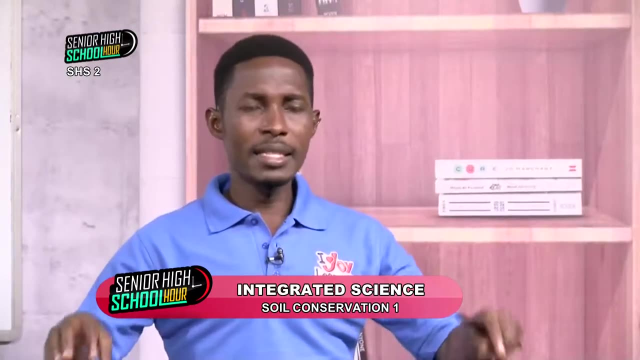 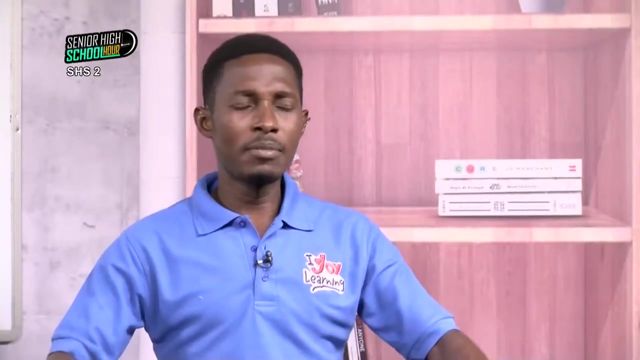 In crop rotation. what we actually are doing is maintaining the soil fertility or e-nutrients. Why, If I keep planting maize here, maize has specific requirements- If in a year, I have to plant maize, which is a three-month crop? and assuming every three months I can plant the maize, what happens is that generally too much I plant, the maize will take some nutrients. The next three months the same maize will take that same specific nutrient. So about four successive planting the next year. then the nutrient needed by that plant has been exhausted. Why are you going to get it So? farmers rather thought it this way: Assuming one plant needs legume, we'll plant a leguminous crop first, like what I explained. Then the legume will give nutrients. such as nitrogen to the soil. After, let's say, three months, we'll harvest it. Then we'll come and plant another plant that rather needs the nitrogen that the legume plant had already deposited there. So when they take it away, it means that we've lost the nitrogen. 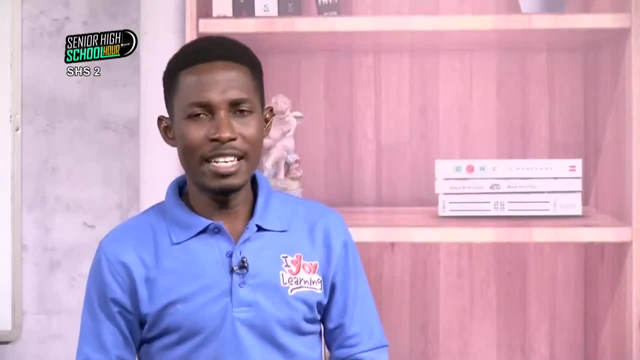 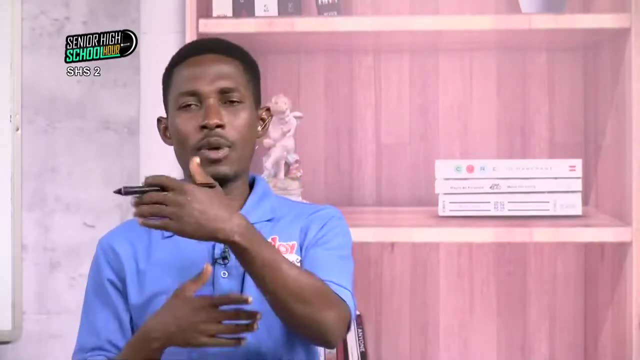 Then we'll come and plant another plant that can give us that nitrogen back. So you see that we plant something that brings some nutrients, Then we plant another one that takes it out, Then we plant another one that brings it. So you see what we are doing. 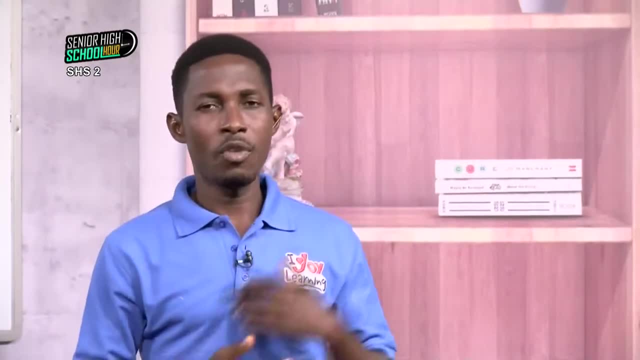 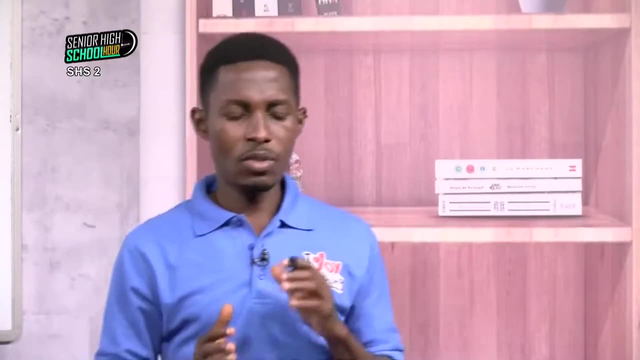 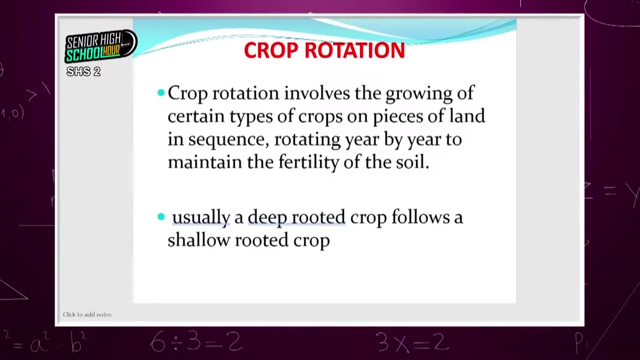 We are rotating the planting from one plant to the other based on certain calculations, Decisions we have to make, And that's what we term as crop rotation. So most of you say: usually a deep rooted crop follows a shallow rooted crop. Why? 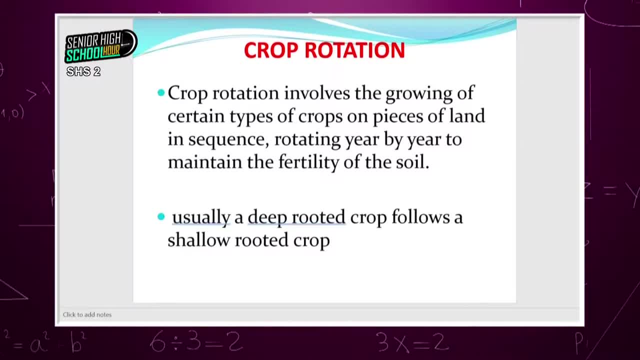 The deep will require to take their nutrients deep down, not at the surface, Because the roots, rather, will grow so deep. it will take their roots, their nutrients, deep down. Then damage will deplete all the nutrients down there. Then we'll plant another. shallow rooted plant who rather the next time don't need to go deep but will just take a few at the top. When they take those at the top, probably leaching and other things will drain some of the nutrients that was at the top down. 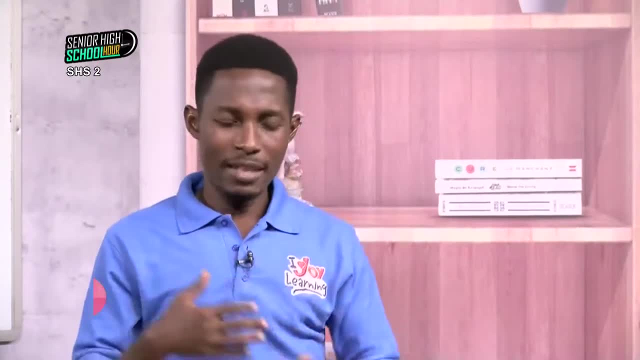 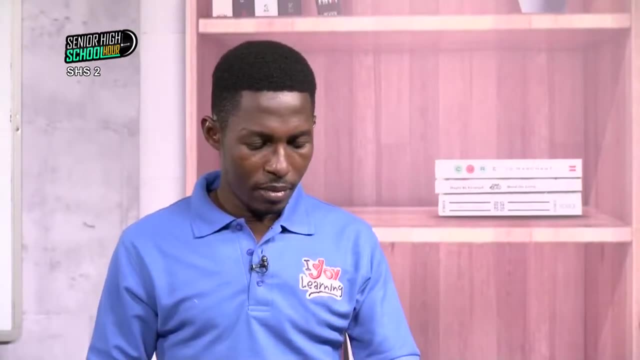 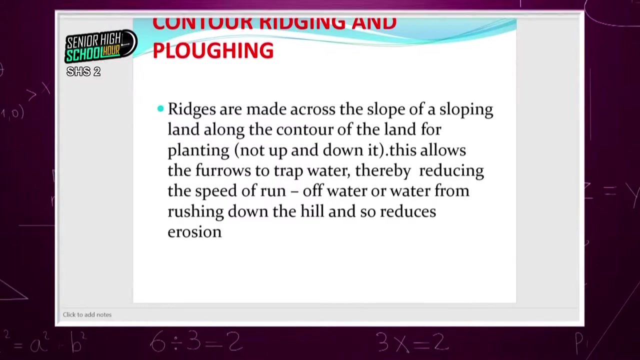 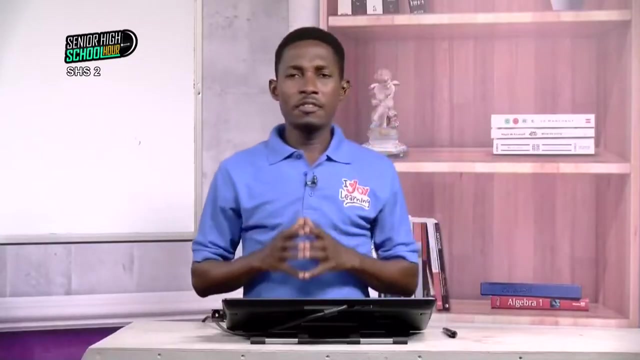 Then we rotate it in that order. This is how the farmers utilize crop rotation. Another is what we call contour or ridge plowing. When you are on a slopey land, sometimes you see farmers planting on, maybe the hillside of a mountain. 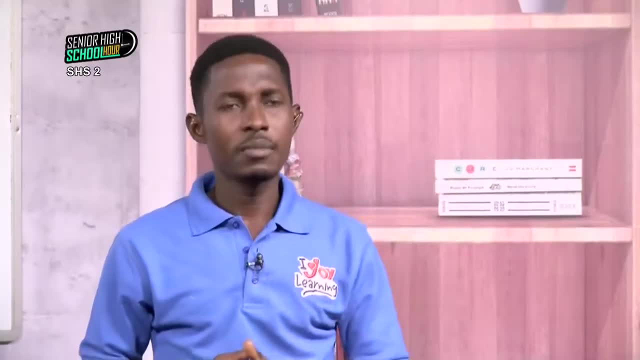 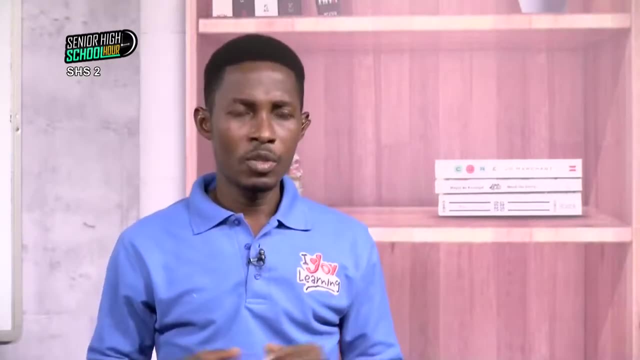 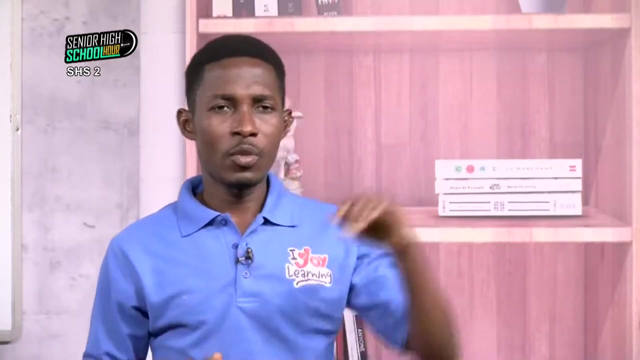 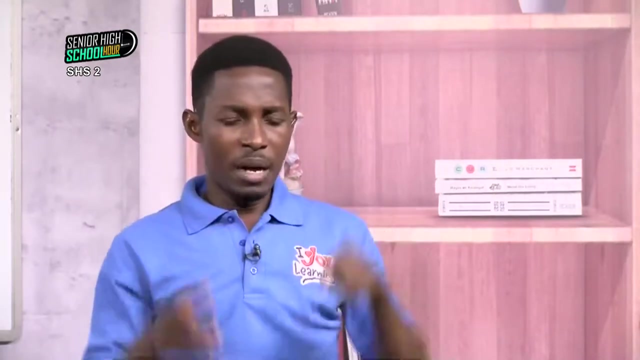 They will need to prevent the soil from being eroded or carried away. There are two things they do. They either plant along the contour or they do terracing. When they plant around the contour in that direction of the mountain, what they are doing is contour plowing. 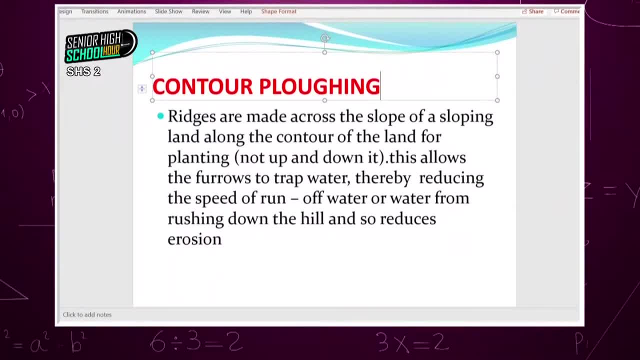 That means they are growing the plant in that direction. This will hold the soil from being run down If they decide to do what we call the steps method, which is called a terracing. Let's look at a picture of a terracing. 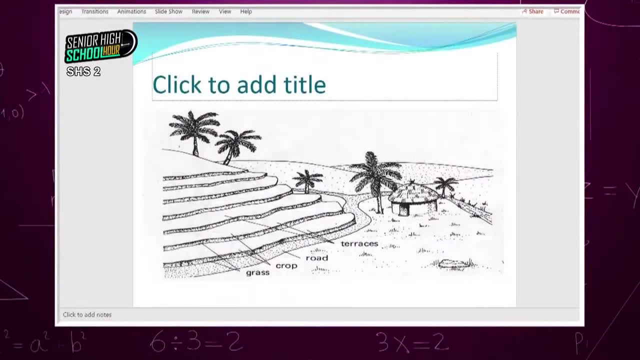 It's a step. They create the normal steps. If the rain is washing the soil, it will start from the first step. It has to go at this time, before it goes down. In that sense, we are reducing the speed at which the soil is washed away. 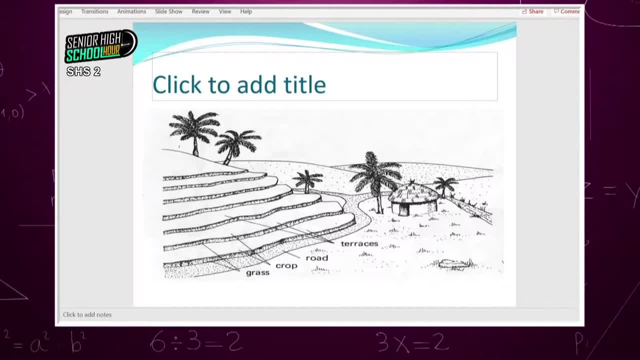 as compared to if it's on the hilly side of the mountain, That one will just come on the slope very straight If it's coming and there's steps. this way, it will reduce the rate at which the soil was washed away. 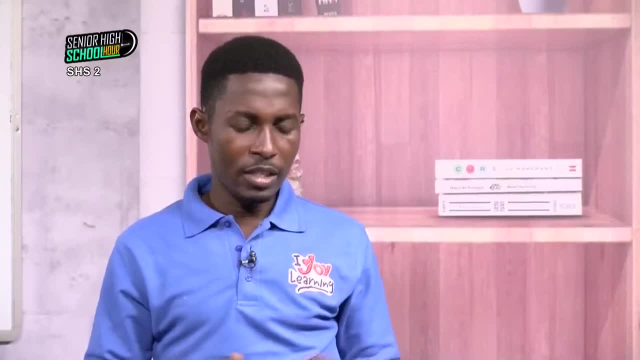 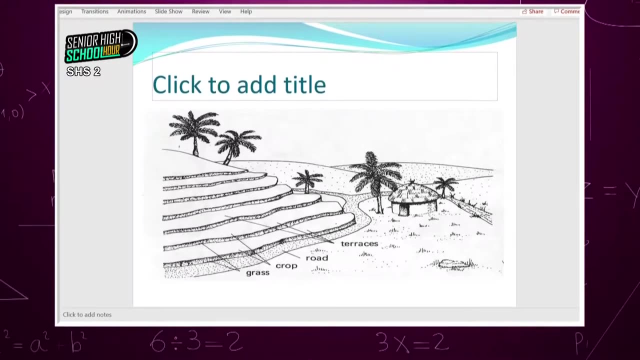 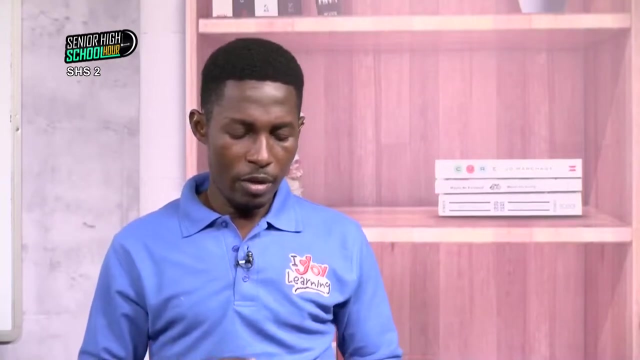 That's terracing. This is terracing. That's the picture you are going to see. Terracing deals with steps like your staircase, While contour means plowing along the design of the land to prevent the rain from washing away the soil by water. 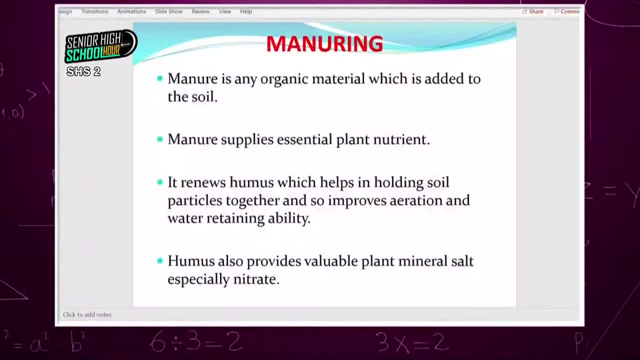 Another means is manuring. Sometimes, by excessive planting, soil nutrients are lost. To get back to it, we rather spread onto the farm either organic or inorganic substances. That is called. the process is called manuring. What we spread is called. 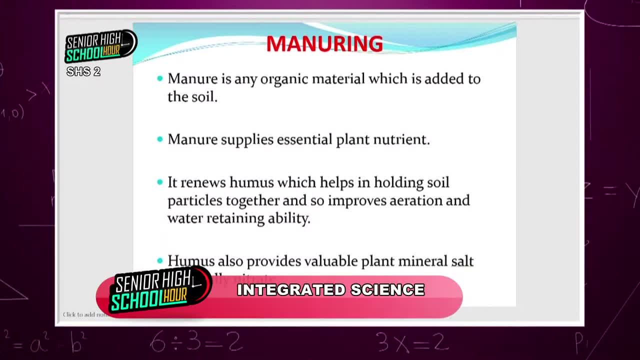 the manure. Manure is inorganic material which is added to the soil. The aim is to supply the plant with a lot of nutrients or to renew, usually the humus that was in the soil that was lost. There are types of manure. 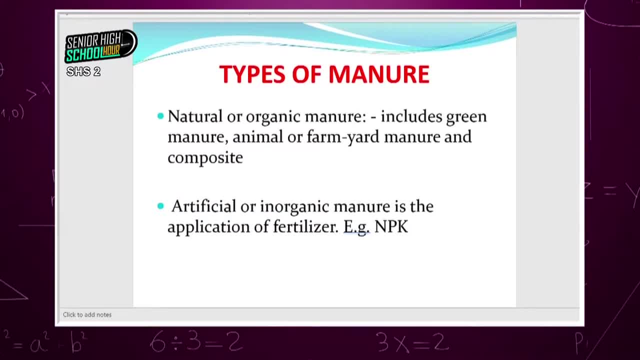 We have the natural, organic and artificial. Natural means comes from nature, such as you can even add Africa matter to it, the animal or farm yard manure and the composite. Composite is formed when they put things like fish cabbage and use a process. 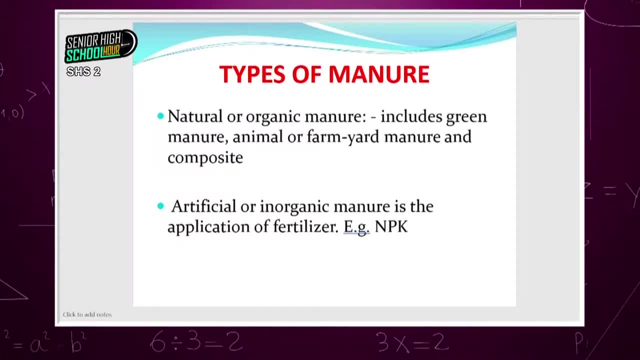 to decompose it and later spread it onto the farm. The artificial or inorganic ones are the fertilizers we buy, manufactured from the industries Usually. we have a popular one called MPK that farmers spread onto their farm. P stands for nitrogen, P stands for phosphorus. 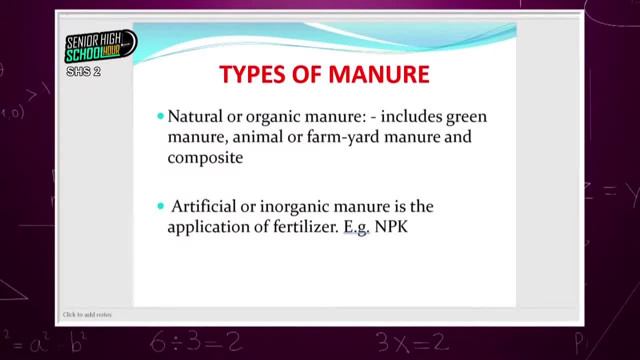 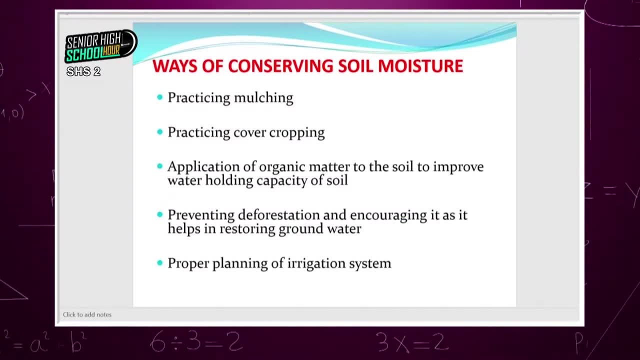 and K stands for potassium. So, for all that we've discussed, we summarize some of them and use as a means of conserving soil moisture. If it has rained and there's a lot of moisture in the soil, what will happen? for us to prevent the moisture? 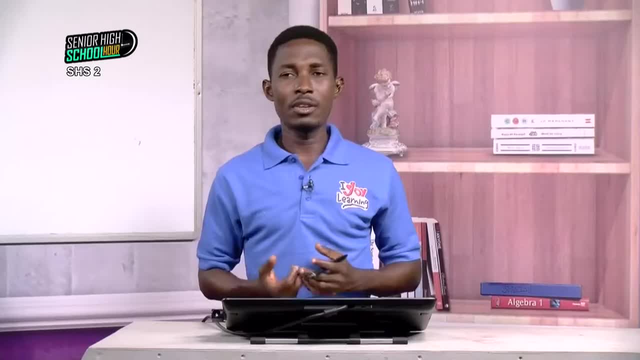 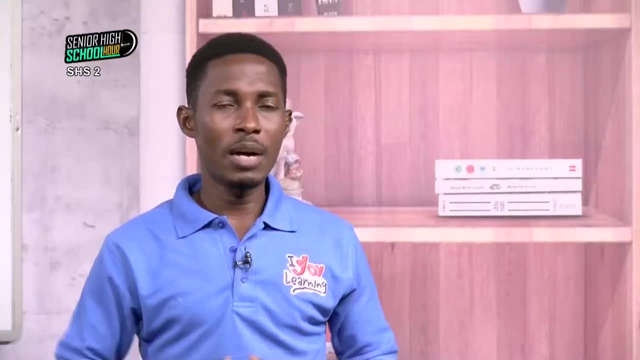 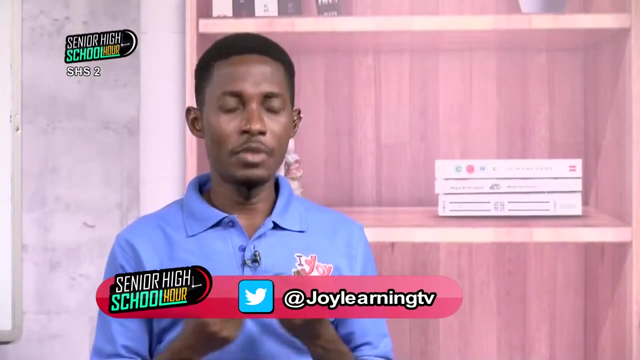 from being lost. One is your cover cropping, Another is your mulching, Another is the organic manager I just spoke about. Once you spread on it, it has the ability to increase the soil structure so that it can retain water, Also prevent deforestation. 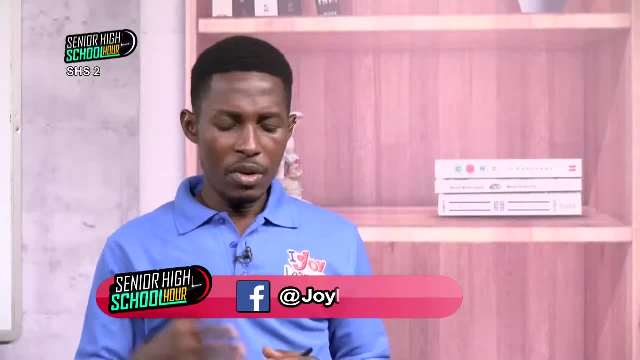 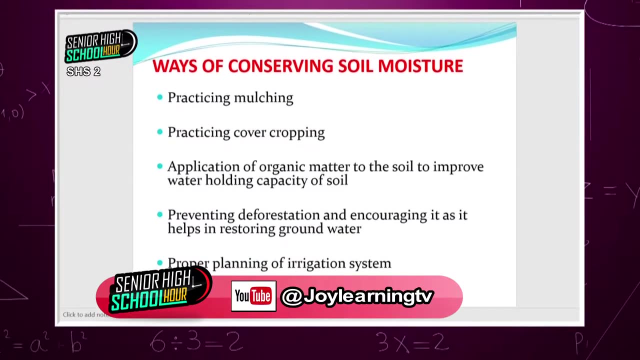 and rather encourage afforestation. When you encourage afforestation and prevent deforestation, it covers the land so that most water is reserved or contained in the groundwater. Then irrigation: Use proper irrigation method. If there's no water and you rather give some more water. 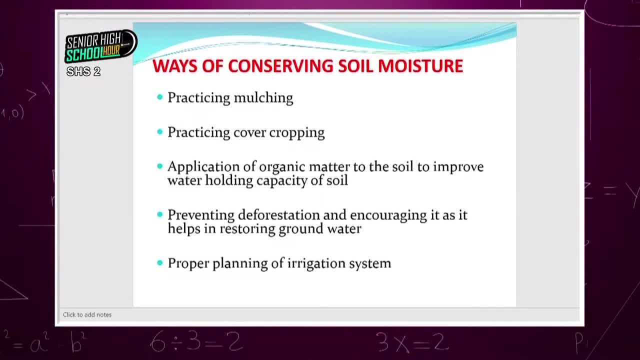 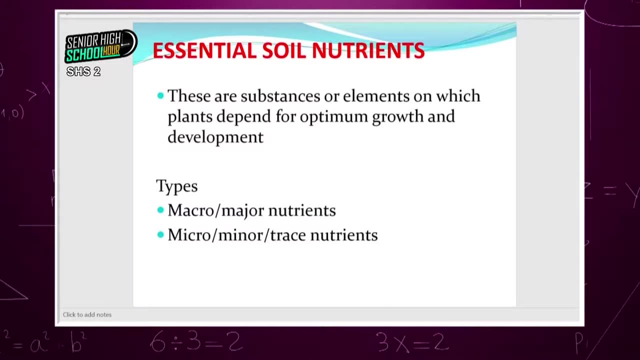 the little in the water will be lost. We also mentioned soil nutrients. I said that there are substance or elements which plant depend on it for optimum growth and development, As the elements you see on your periodic table. but they occur either naturally or artificially in the soil. 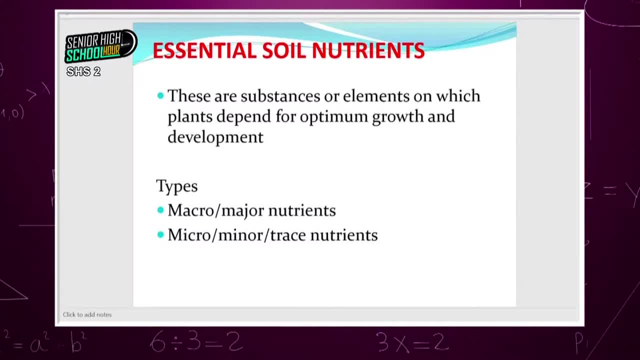 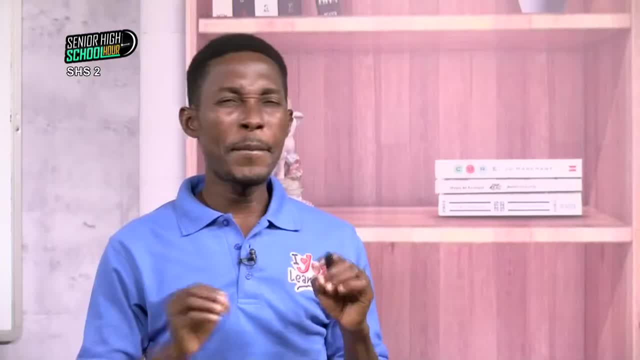 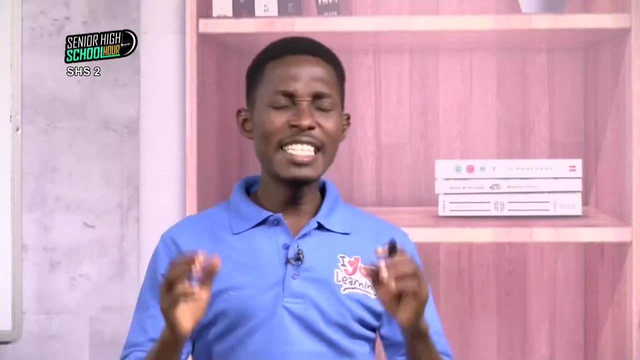 There are two types: the micro and the macronutrient. Why do we use the word macro and micro? Okay, let me turn around and say major and minor. Major means that they are needed in large amounts or quantities on most basis to 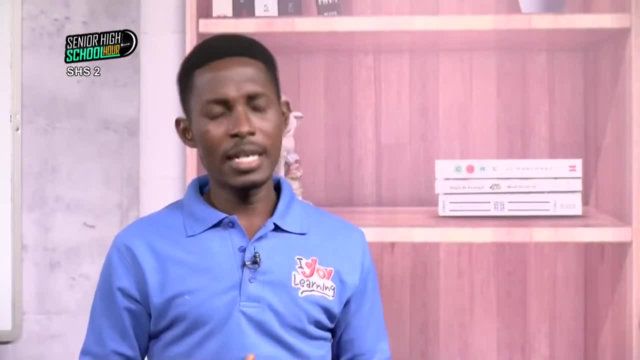 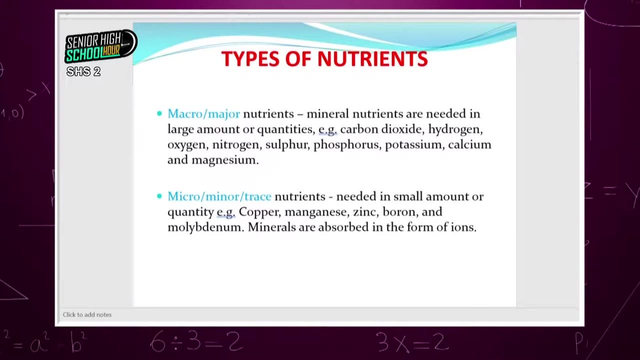 or in very short times. Example is the carbon dioxide, the hydrogen, the oxygen, the nitrogen. sorry, the carbon itself, not the carbon dioxide the carbon itself: Hydrogen oxygen, nitrogen, sulfur, phosphorus, potassium, calcium. 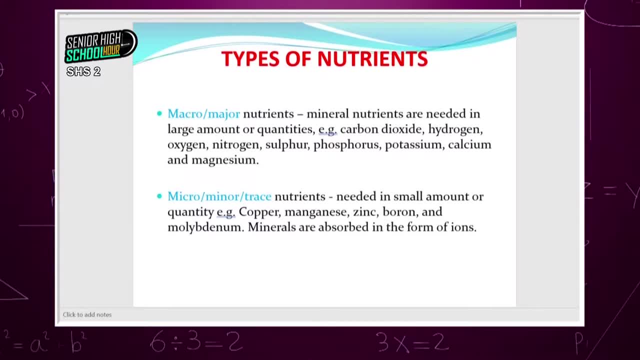 and magnesium. These are the major ones that plant need on large and on daily basis. Micro or minor means needed in small, small, small, small, small amount or small quantities. You can say trace amounts. You have as copper, manganese, zinc, boron. 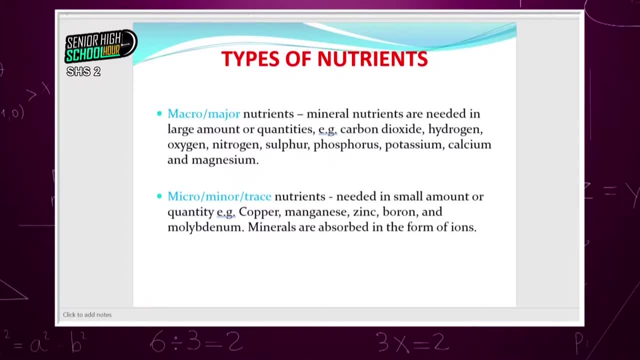 and molybdenum. Note that whether you are major or you are minor, for the plant to use you you have to be in the form of ions. So what I mentioned were neutral states. They need to react and lose some electrons somewhere. 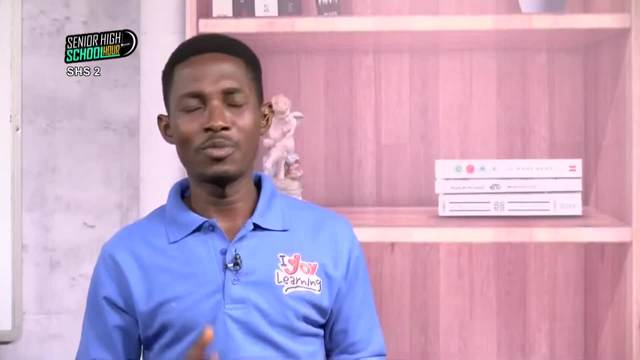 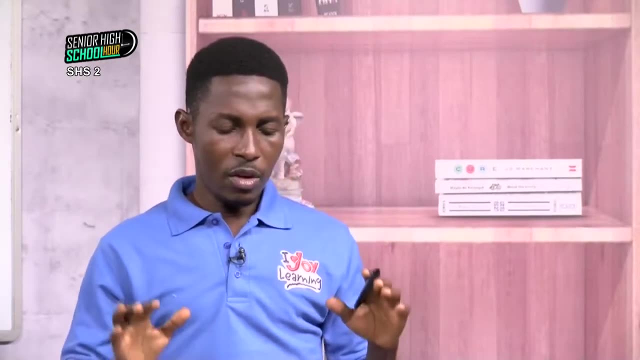 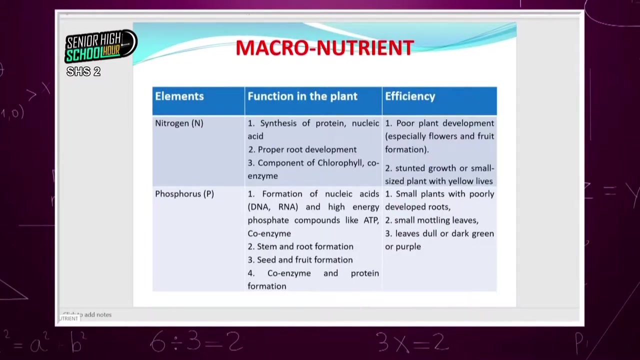 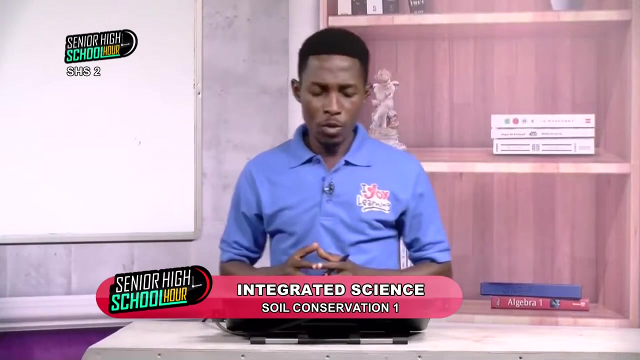 and become either a cation or anion before the plant can pick them up On your screen. you are supposed to know the functions of these nutrients, And if they don't, what happens? We are required to also know the functions of the nutrients. 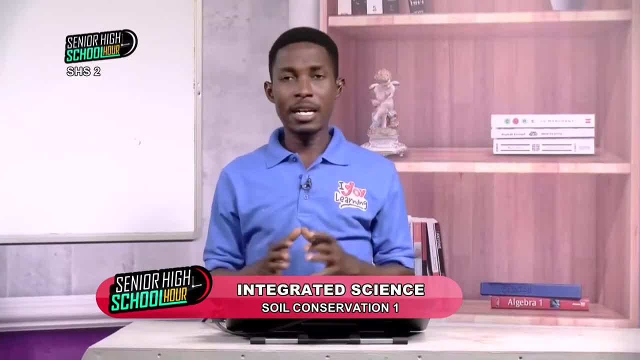 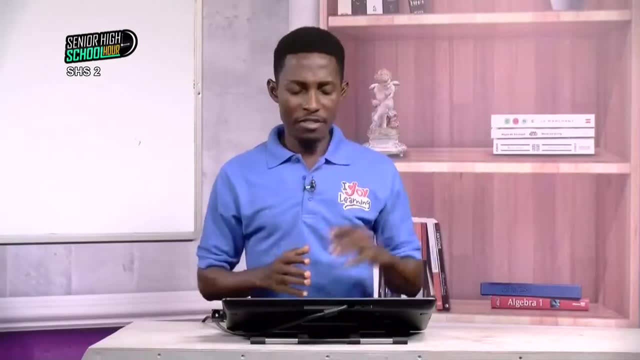 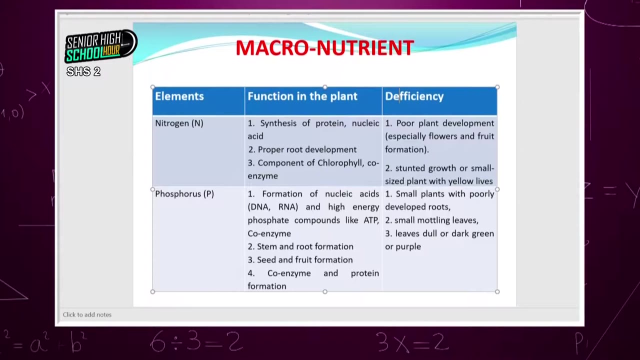 We'll just pass through the critical ones and keep them in your head and observe it on plant. One is nitrogen, which I've mentioned during the teaching. Key thing is that nitrogen is used in protein synthesis- tessus- you the body that grows. we need a lot of nitrogen and also good for proper root development. 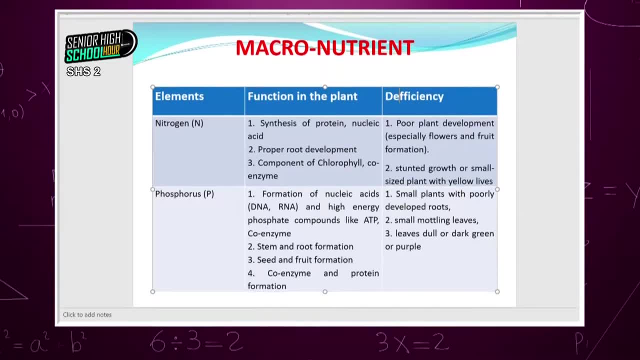 if they don't have it, because it's good for proper development, is the root that holds the plant. once they don't have it, there's a poor plant development or growth. then the plant doesn't grow well because, human being, you need protein in every part of your 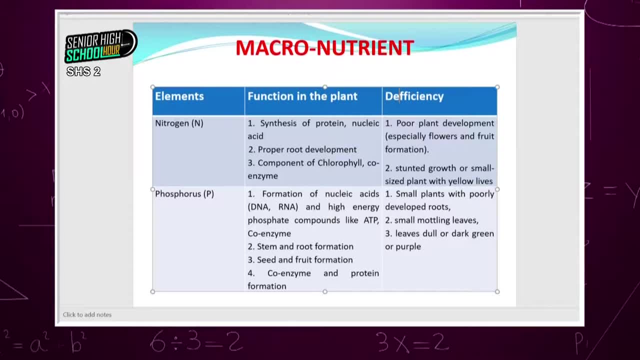 body plants also need protein, every part of their cells and their body. once you are not getting it well, then their standard growth or you grow in a very reduced rate and become small. nitrogen and phosphorus are needed in the dna, so as nitrogen is in that, in protein synthesis or your dna. 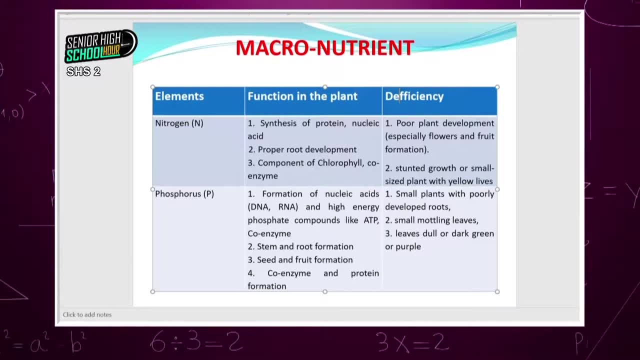 formation. phosphorus is also needed in that same dna and rna formation. so they also for the same stem and root formation, seed and fruit formation. not getting it the same consequence the plant to have standard growth of have a small growth size. then there's what we call molting of leaves. the leaves doesn't. 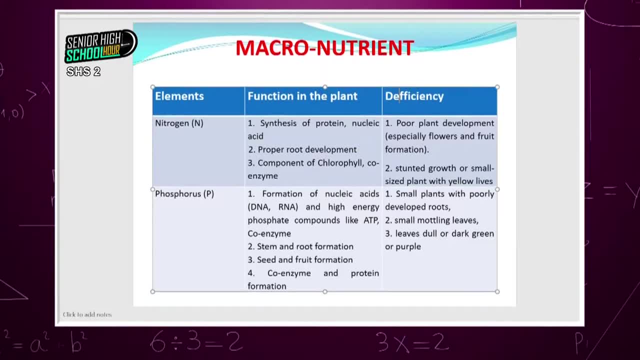 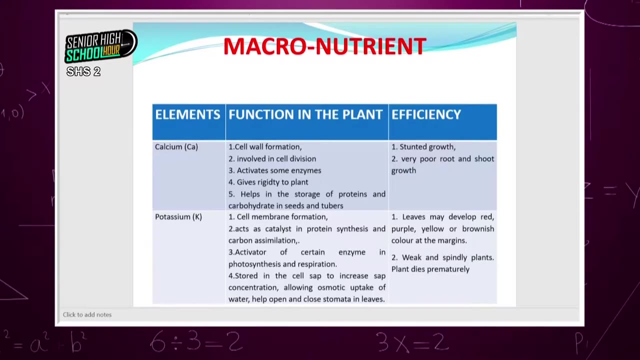 open and grow in a nice, greener form. they say we use the word molted, they become so dull or green, they grow in color at the same time and they 300 neut. 그러니까 all the difference between color tones you need is open. here you start serving and they don't grow so quickly. 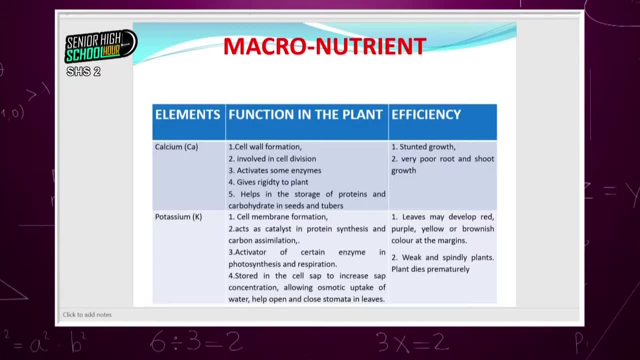 they grow to leafy shape. so it's all about growing. they already have a lot of the DNA that's part of the root of their plant. this is what we call transplantation. you don't have it, you get stunted growth, very poor root and shoot growth. another is potassium. 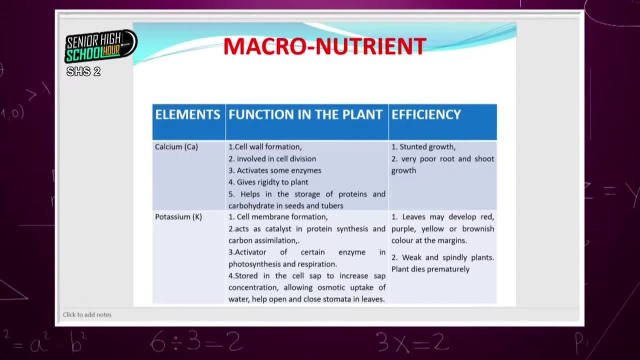 it is needed in activating some enzymes in the plant life, especially in the photosynthesis and respiration process. failure to get immune, that photosynthesis will suffer. they are also using as a catalyst in protein synthesis. the way we make protein. potassium is needed. there is also made in cell membrane formation. when you don't get it, the leaf may develop some red. 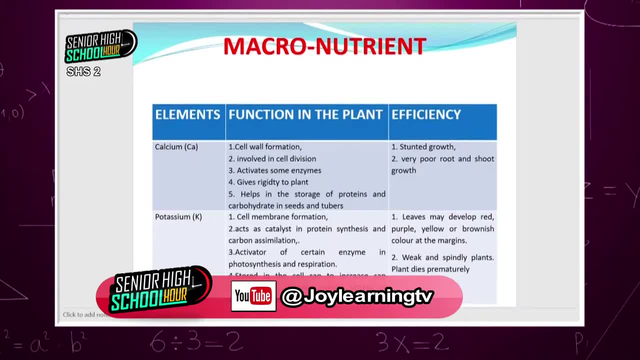 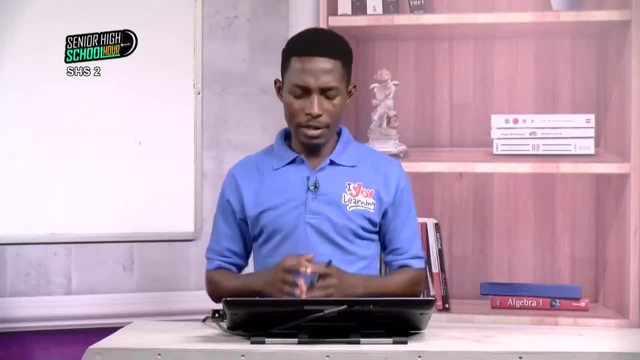 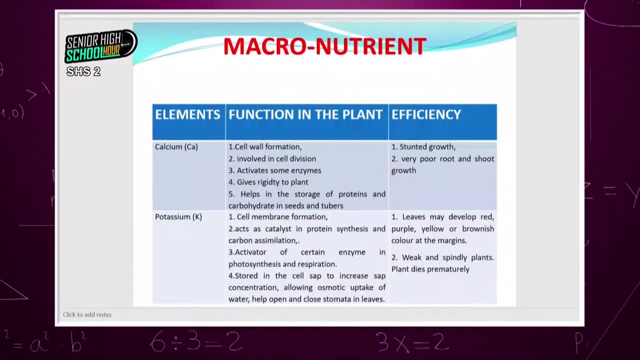 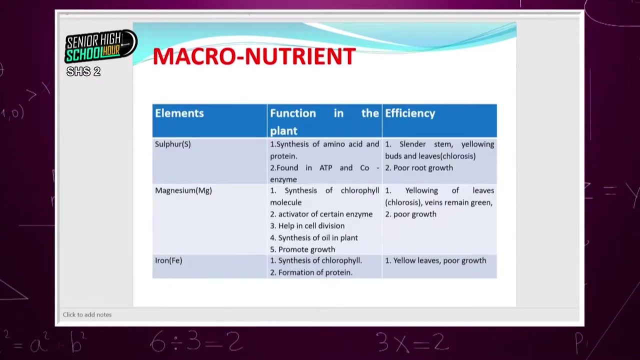 color, or purple or yellow or brownish color at the margins. so if you see some dots and yellow color just at the margins, not at the main side, then know that potassium is inadequate in the plant. then the plant become weak and plant may die prematurely. sulfur also found in atp and coenzymes. they're also used in amino acid, amino acids, the building. 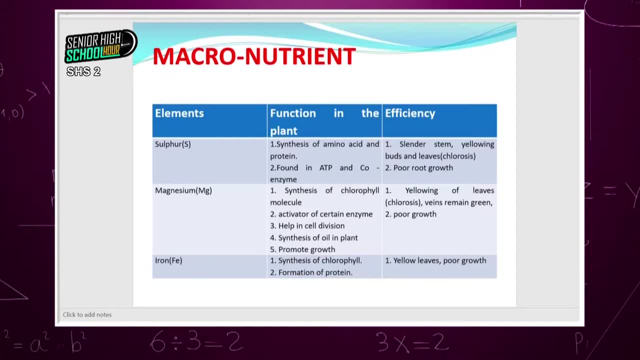 block of protein and sulfur is needed in making that. if you don't get sulfur, your stems become smaller or slender. so if you know the natural size of the stem of the plant, you can see the growth in the plant in this mega manifoldof a tomato and at the normal month. 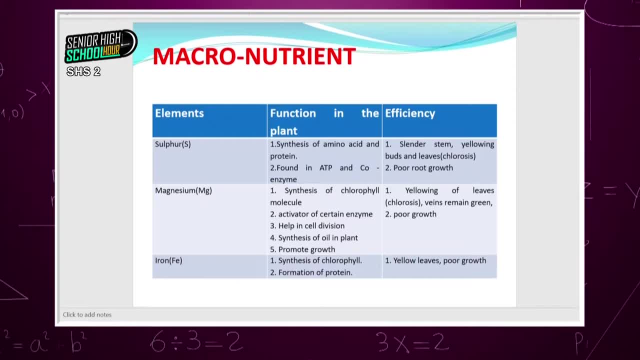 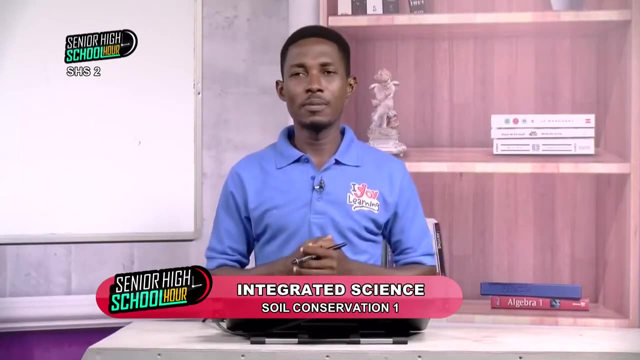 as opposed to seed growth acceptance. it's not growing, then you can then predict that you have a sulfur problem and there's poor roots growth magnesium somebody needed in chlorophyll. you've had chlorophyll- chlorophyll, the key component in trapping the light to make photosynthesis magnesium. 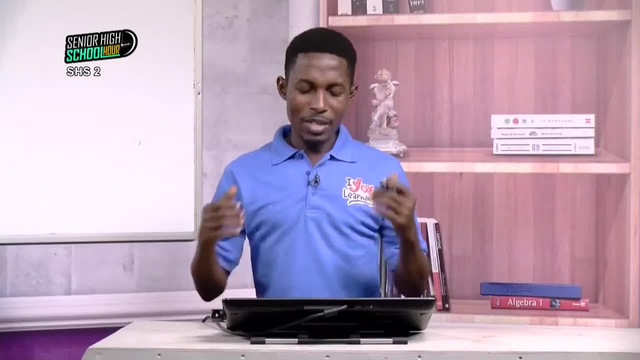 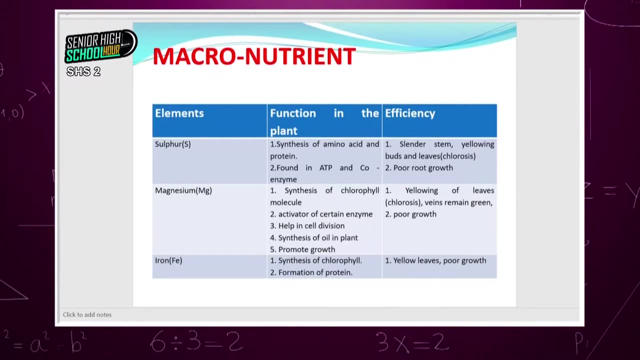 because plants will need to make photosynthesis, so they're also needed in cell division and activating some enzymes. failure to get it means that plants will not make their photosynthesis. then there's some yellowing- these are not at the margin spread on the leaf. it's called chlorosis. 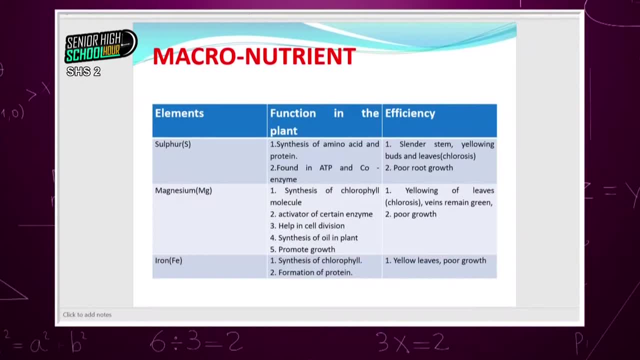 usually on the vein part, the vein where we transport the water. if you see yellow in there, they are chlorosis and it's due to lack of magnesium. then ion is also synthesis of chlorophyll. same. if magnesium is used for synthesis of chlorophyll and they become yellow, ion is 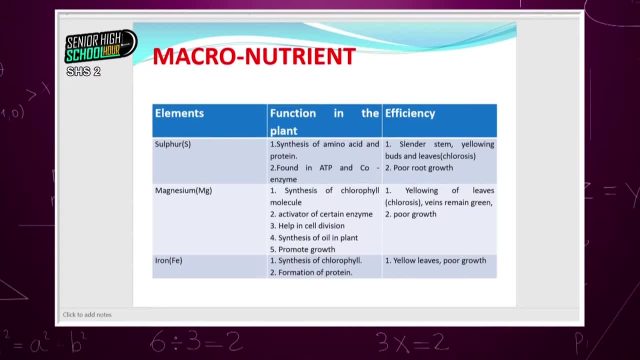 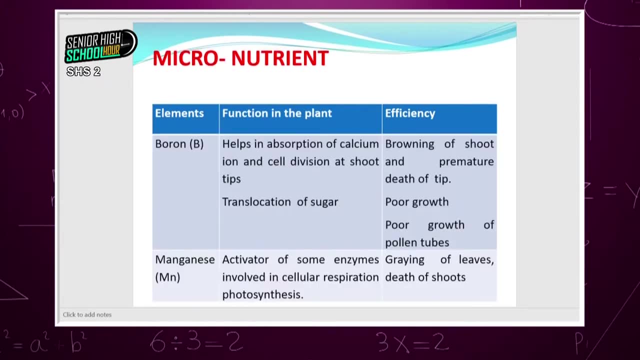 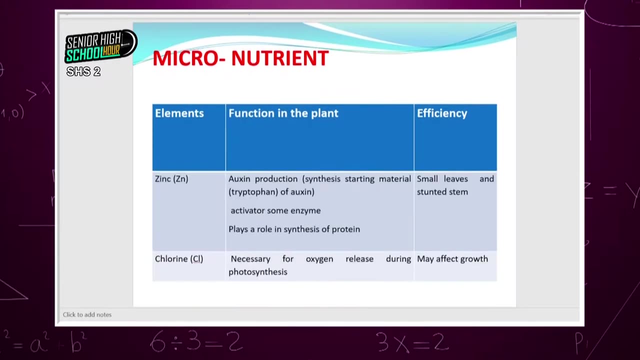 involved in the structure of the compound needed for photosynthesis, so they also become yellow. let's look at the last area, which is the micronutrient. those needed in trees amount small amount zinc. the first one is zinc. plants also have homes, like the way you have your own hormones, what we call growth hormones. 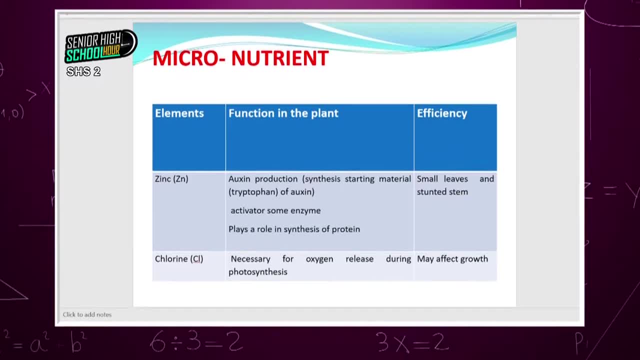 it's called. the popular name is called oxygen. we need zinc in most of the plant hormone formation, the oxygen formation, and this same zinc is involved in protein synthesis and activating of some enzymes. once enzyme come in and synthesis of protein, come in if you don't get them. 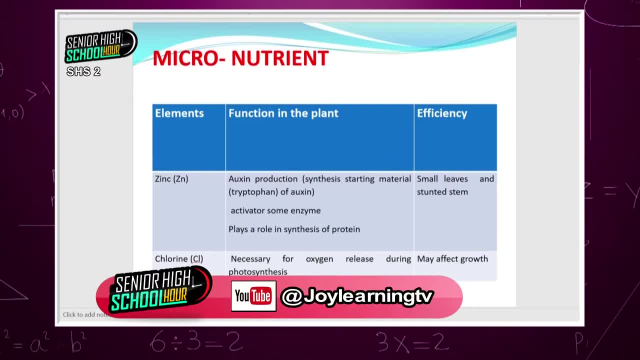 your leaves will become small and have stunted growth. chlorine is needed for oxygen to be released during photosynthesis. it needs to be there for a chemical reaction to take place before we can release oxygen. if we can release it, the whole process, the oxygen will stay within the plant and we say this affects growth. 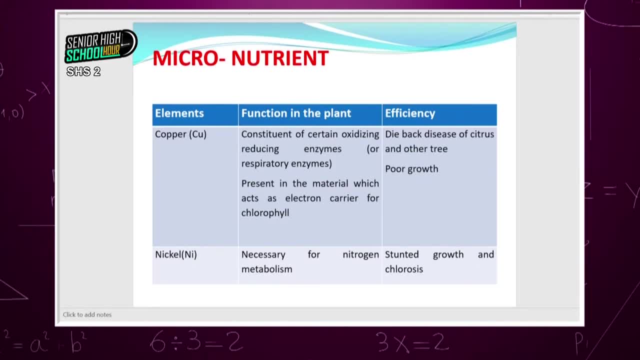 copper. we use copper as oxidizing constituents of certain oxidizing and reducing enzymes. they also act as electron for chlorophyll, a very complex process. but copper, though tiny, is needed in the electron carrier process for fuel. if you don't get copper in your body and that's implant, they die. 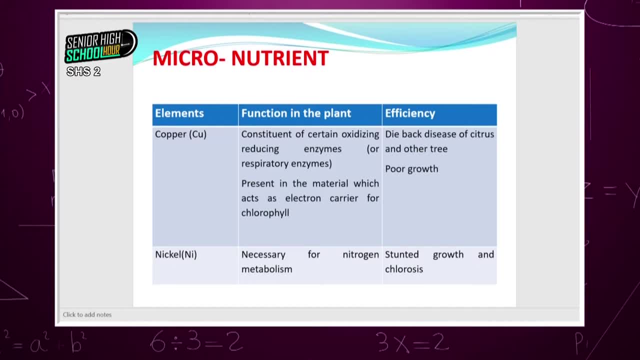 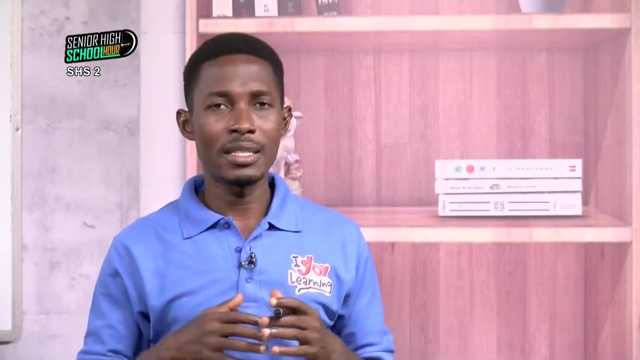 we are something called a dieback disease of citrus and other trees, and that's what we call poor growth. the last is nickel, necessary for nitrogen metabolism. when we say metabolism, we say biochemical processes that go on in your body. nickel is needed for those kind of chemical processes to ensure that it is smoothly. 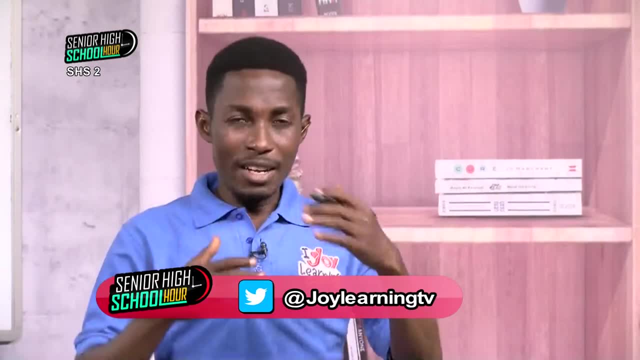 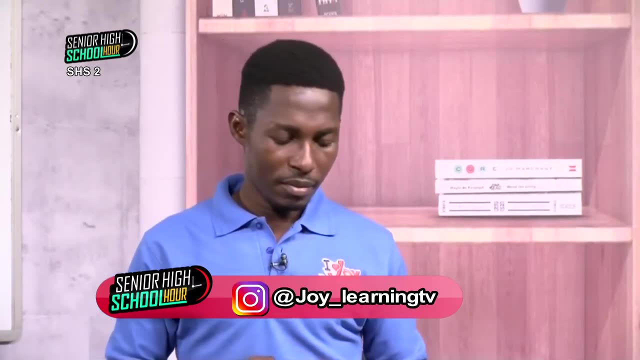 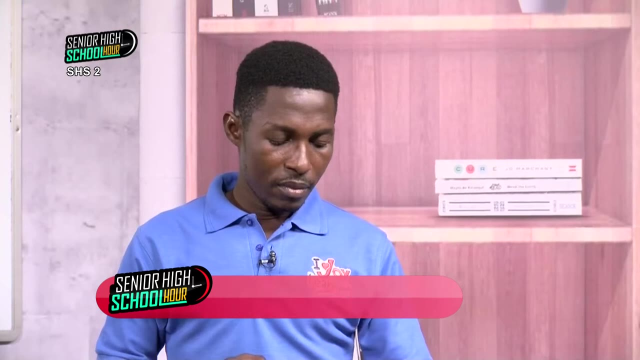 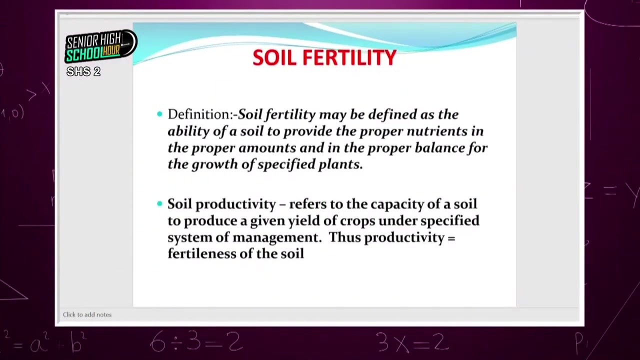 occurring. once it cannot occur, it affects your entire group. so that's what we call stunted growth and chlorosis deficiency. we have mentioned having all die in your body. if you have it in good amount and say that the soil is fatter, if nutrients adequate, air is adequate, water is adequate and the amount of soils quality is adequate, then we 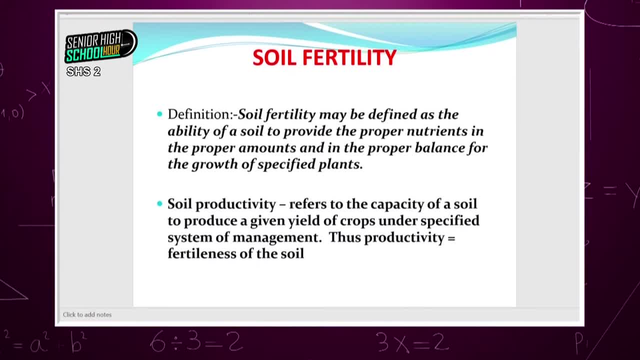 see, dis stewing produces more and more nitrogen, so we are supposed to look at fertility. but not coconut water we mentioned 생겼 this particular study. so this study, this study, see that the cardio from jack bllaus chage'll use the duodenum. i'm not going to highlight this as much ok than you. 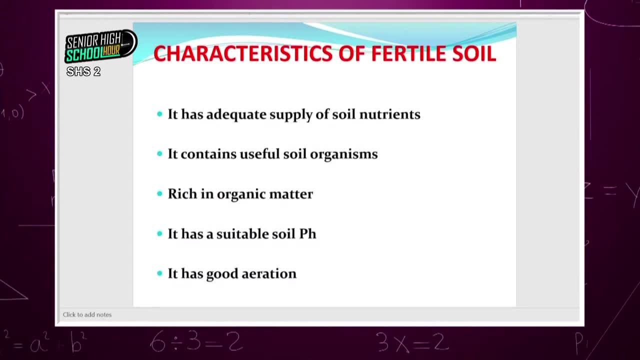 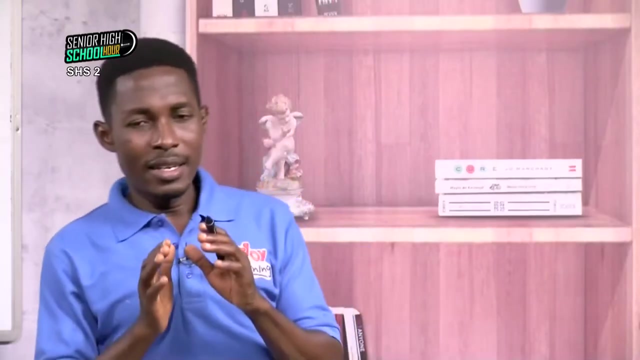 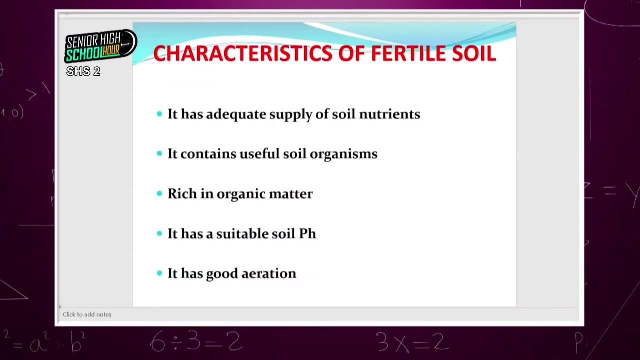 there is fertility And the characteristics are said to have adequate supply of soil nutrients. The content should be useful for soil organisms. rich in organic matter, a suitable pH and a good aeration: These are the good characteristics of a soil. This is the first part of our soil study. We'll come back with the part two, where we look at 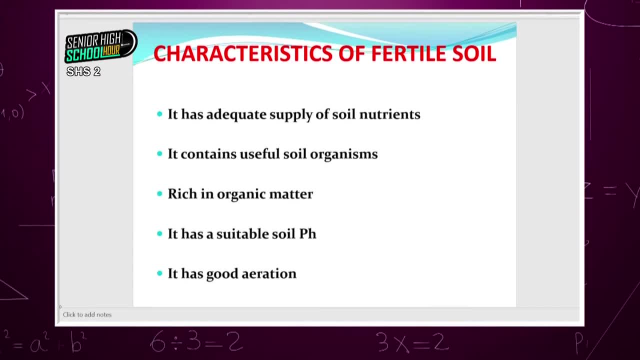 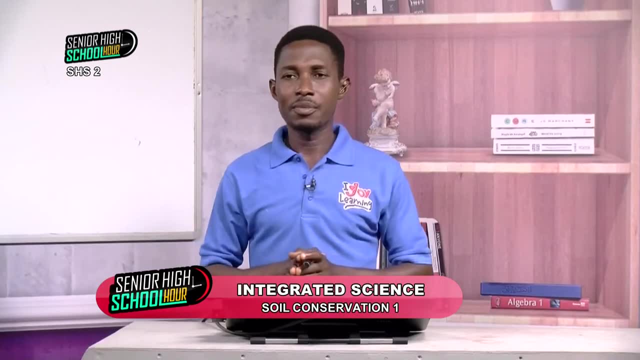 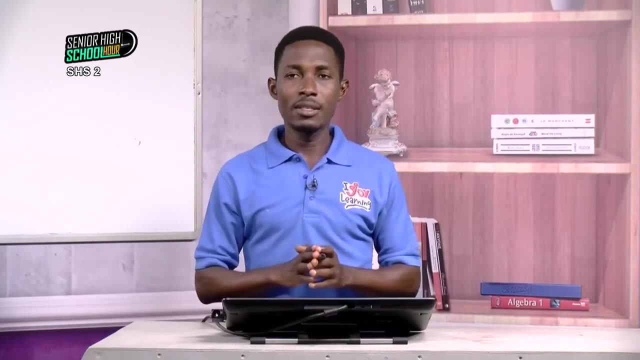 other aspects of the soil, such as loam, sand testing and the texture and everything. I believe we've covered enough. We've looked at soil definition. We looked at what can let us lose our fertility, What can other nutrients and maintenance of the soil, moisture or soil. 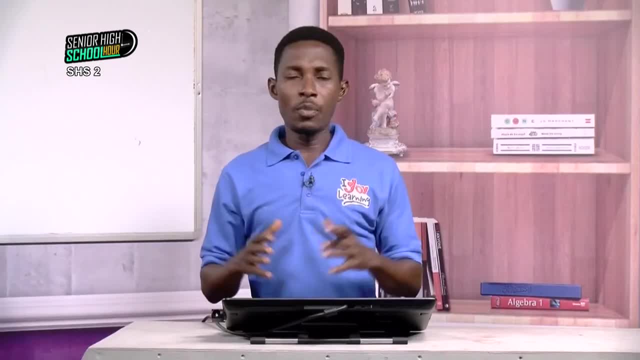 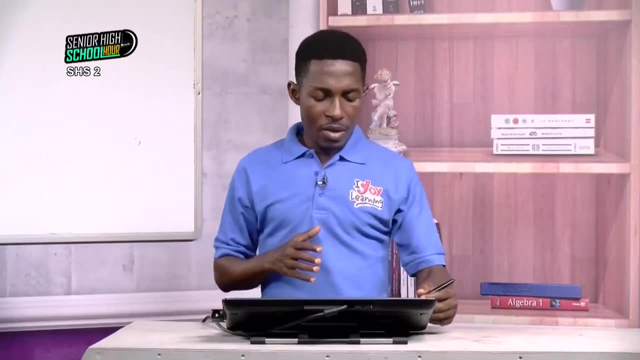 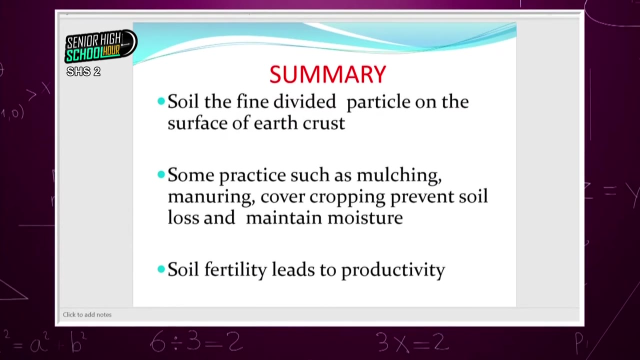 We've also looked at the nutrients Our employee to go over as it to be the basis of the 성공 part, What I think it is. it says soil is the fine divided vostmusic of earth crust. Practicing, ahhm, Mulching, Manuring, cover cropping will prevent.